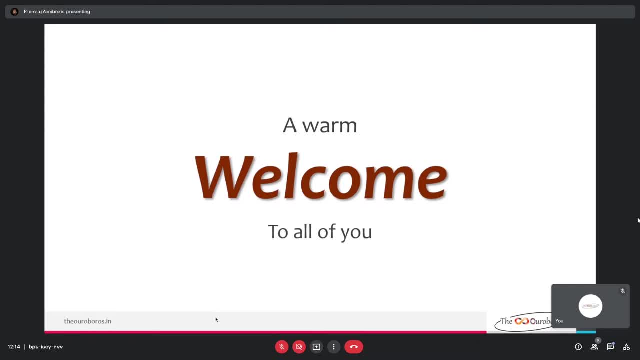 the most. okay, thank you for the participation and I want energy in this whole session. so before I jump into the topic, we must know what is Aurobis community is why we are here and what this community will give you. 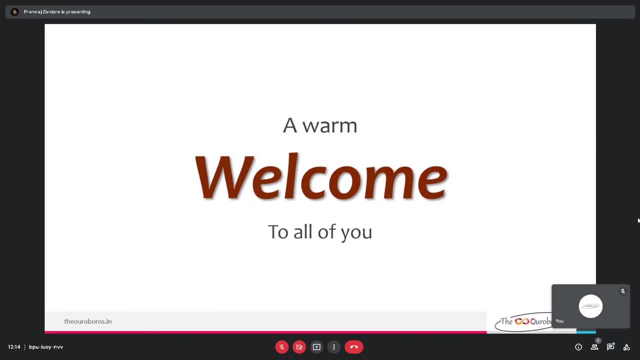 so Aurobis community is a platform where you are provided with a good education system, where you can study about different technologies. here, job-oriented training is given to achieve your dream job. whatever you want to dream, there must be a dream company, right? so you? 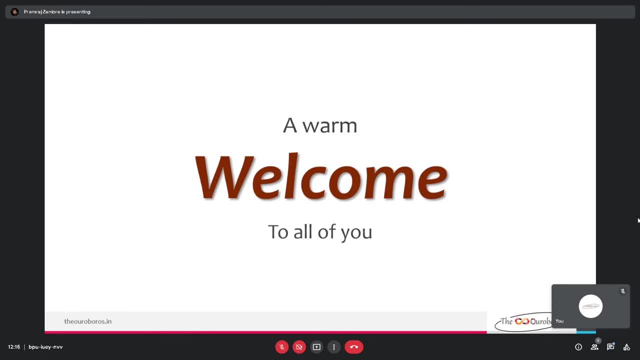 can achieve that. we give that guidance and the guidance is provided to those people who are working in a multinational company, in this company and also in good companies. so welcome everyone here and to know more about AuroBis community, you have to be still connected in this session so that you will. 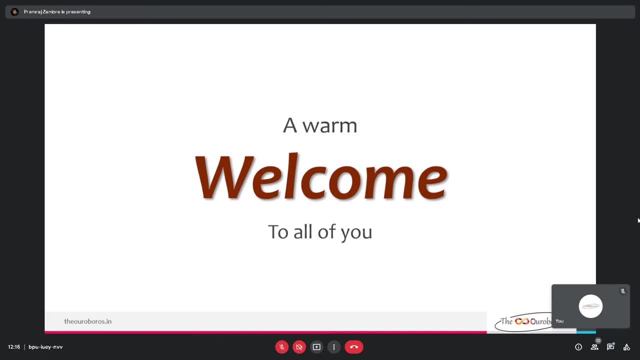 know more about AuroBis community. so we can jump into the session now, which is SDLC. if anyone knows about SDLC, they can type in the chat section or you can unmute by clicking subscribe and then on the right side. 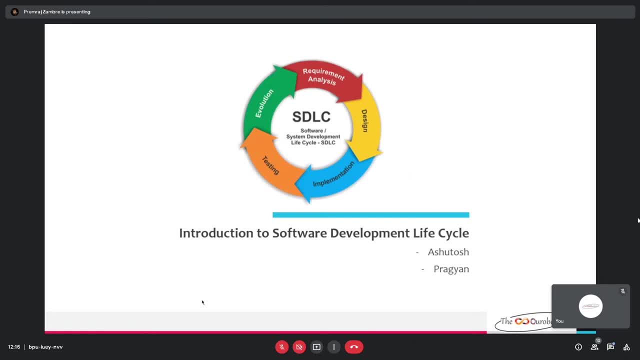 be free, don't hesitate. there's a first rule. if you want to continue this session, even if you want to speak in hindi, it is allowed. in this platform there is no barrier. so anybody knows what is the full form of sdlc. so great, mithilesh, thank you. thank you so much awesome participation. 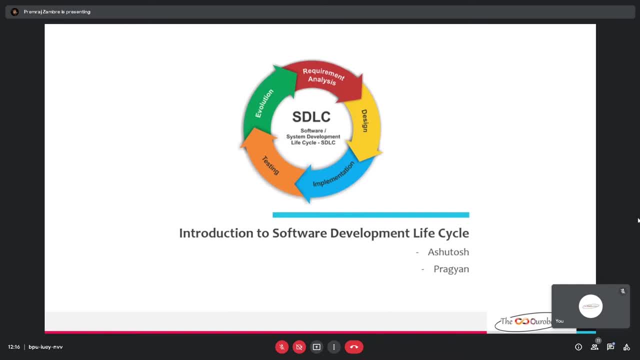 anybody else who want to give the full form of sdlc? yeah, it is right in front of you, even though fine. so it is a software development life cycle and this session will be hosted by ashutosh and me. so before i jump into this topic, let me ask you one simple question and promise me you will reply. 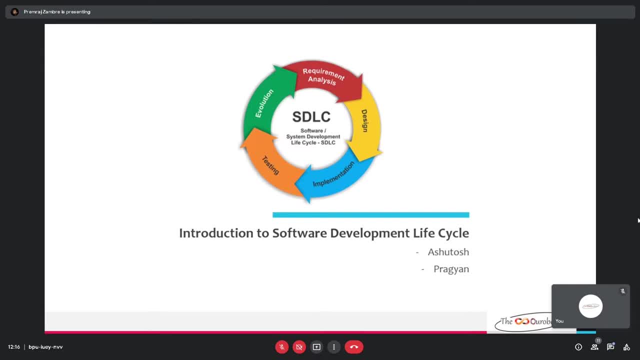 this time you can't be silent, okay, so any group activity like social science exhibition, science exhibition, any group activity at least type yes or no. yes, okay, awesome. how many group activities have you done in the past? this means active participation and that's the answer we want. you don't say much thing. 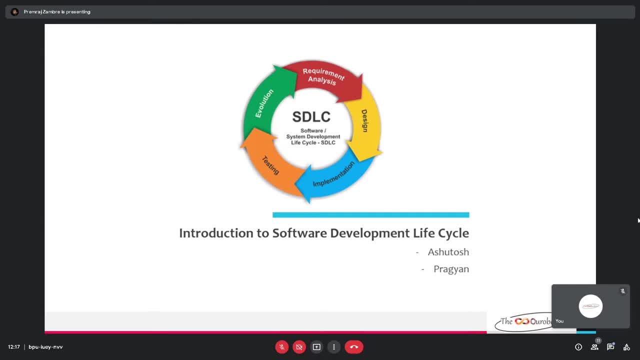 but at least say yes, no, okay, we get got a one. yes, okay, that that is a great thing to start with. so, yes, some of the people have went under the group activities. so anybody wanna share his or her job experience? any group activities. any group activity. so what have you done in that group activity? anybody wants to share the experience? 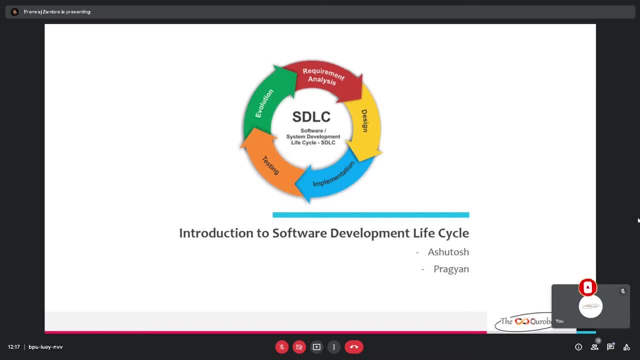 okay. so i will ask, ashutosh, if you have any experience of such a group activity in your school days, so we all want to hear that. hello everyone, am i audible? yeah, hello guys. my name is ashutosh. as told by pragya um, i work in a multinational company. 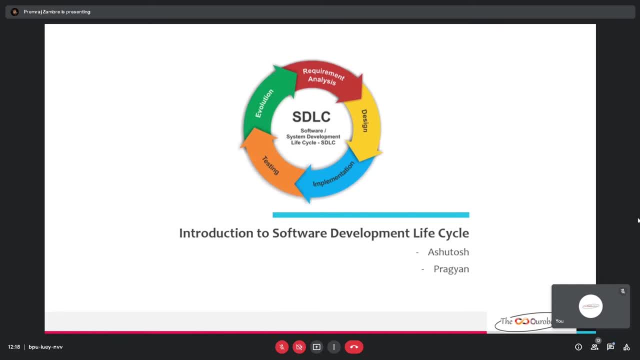 as a software developer and over here, like pragya asked me to like tell one of my experience working in a group project or something like that, right? so yeah, i have one experience, not one. i have many experiences, guys, okay, so i will share one with you, okay, uh, like, 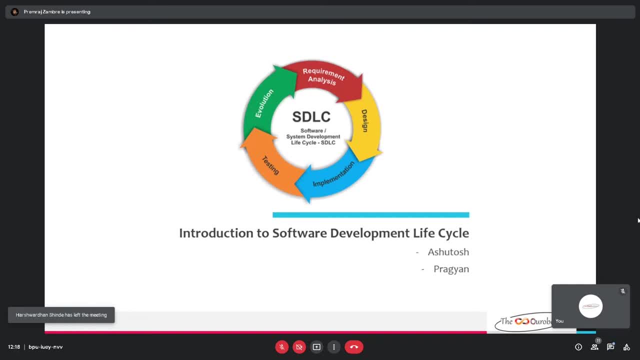 then, after, like, i formed a group with few of my friends- one was priyansu, pisley and varun and all those peoples- and we decided our day: okay, that we will meet up at priyansu's home and we will discuss what discuss what we have to build. okay, so when we met together, 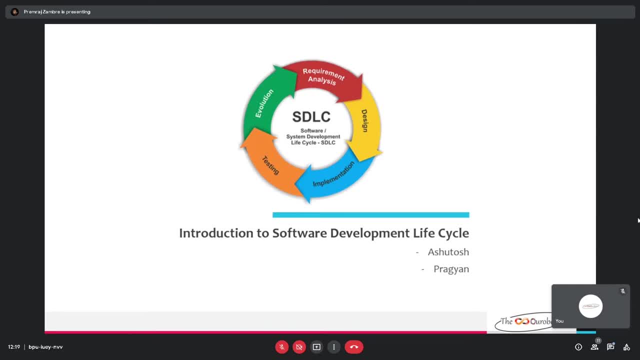 we did stupid tasks and was playing games, eating, etc. we were really busy at that- right working anything for that matter. Then, after 1-2 hours, we realized that we had to discuss something. so we discussed those things and we decided that we will build a model on a smart city. 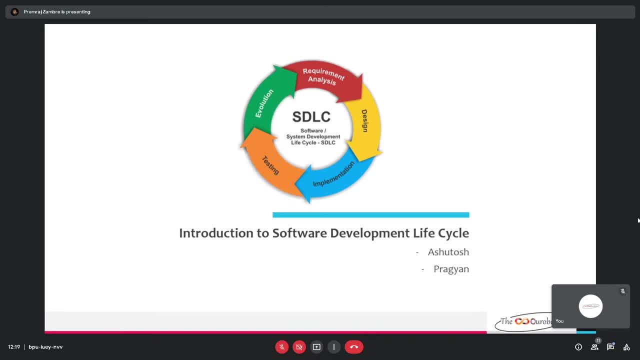 Then for the model, we thought: what will be the requirements of things like how? we will want to build it From PPT? sorry, we will want to build it from POP, ie from plaster peris wood, thermocol clay and all those things. 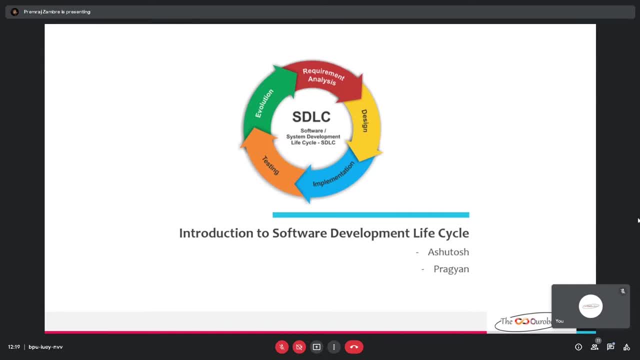 From whom we will want to build it, what features we will want to add to it and how much money it will take, what resources it will take, how much time it will take. We were discussing all these things Then. when we discussed all these things, then the time came for us to build this thing. 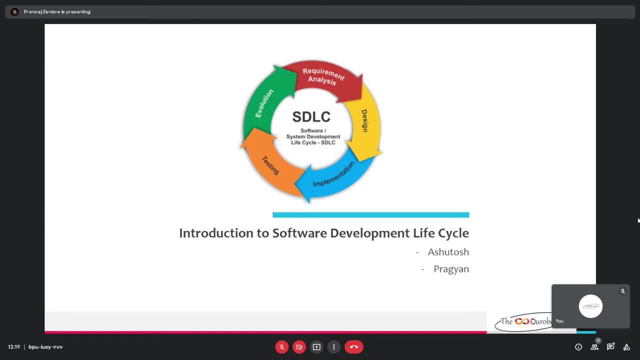 So when we were building it, what happened? we forgot a lot of things, that what we had to do and how we had to do it. And do you know why this happened? Now I realize why this happened Because when we were discussing all these things, so what happened that way? 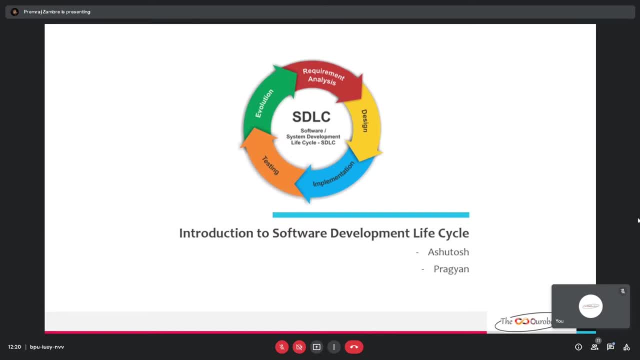 We didn't wrote anything like, we didn't specify or write any details that, yeah, these are the things or these are the crux points that we are going to do in later stage. Okay, so this is the thing that I realized over there. 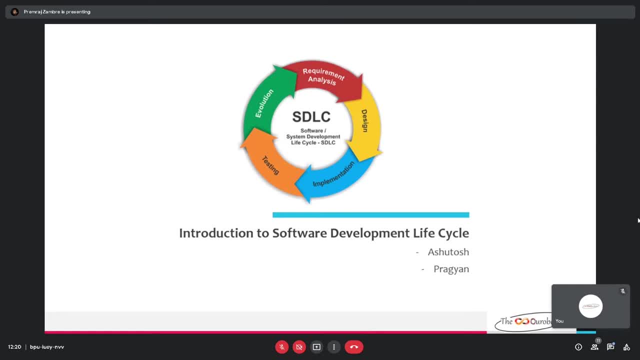 Okay, so this was my experience when I was like when I did a group project, So does this answer your question, Pragya? Yeah, yeah, Thank you, Ashutosh. So before we move on, there's a link which is coming to your chat section. 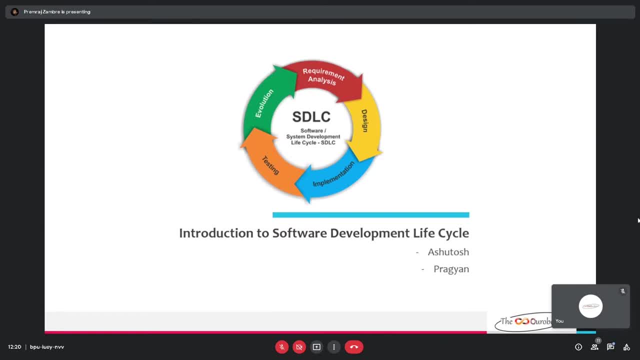 So there's an attendance form, just a small form, And please fill that form so that we know how many of you are enjoying this session. Of course, everyone is enjoying this session, So you can say it's a love of token from your side to us. 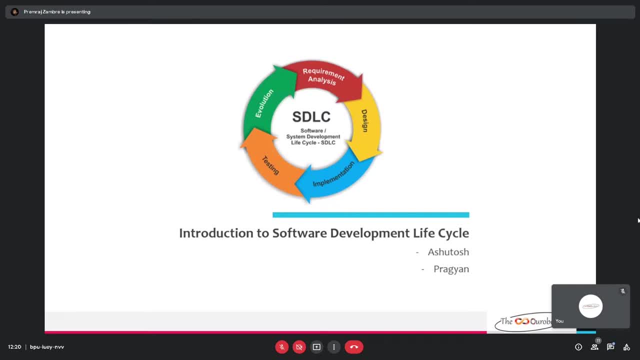 You can please fill that attendance form. So thank you, Ashutosh, for your experience And we love to hear that how you planned it. Whenever we decide something, whenever we want to make something- even if we want to make a website or cook something- we need a plan. 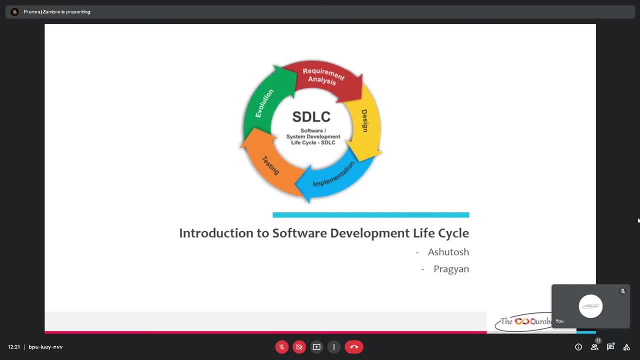 We need a strategy, right So, when we have to make so many plans and strategies for so many small things? so these large organizations, these multinational companies, these IT companies, how they are handling this large project- Microsoft, Google, There are so many different modules in it. 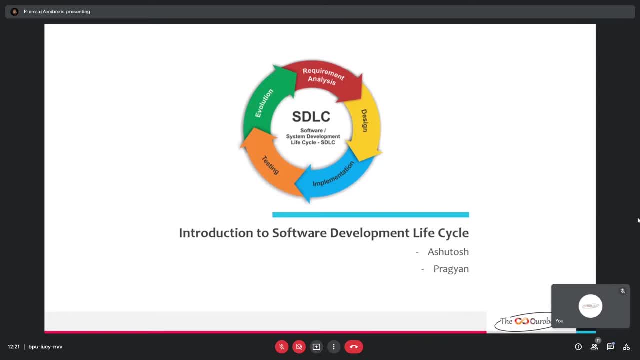 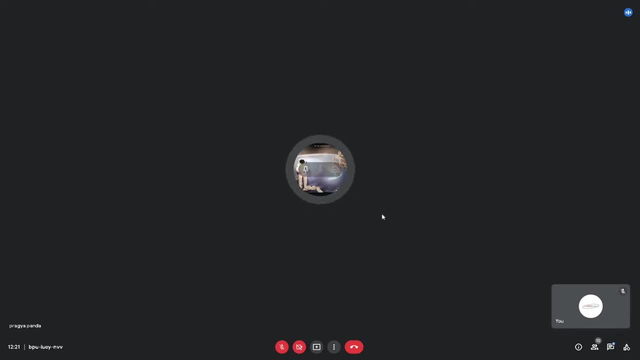 What are modules? You can say it's a small part, Okay, Like if we are making today that we want to make a North Indian thali, Okay, And in that there is a dal, there is rice, there is chapati. 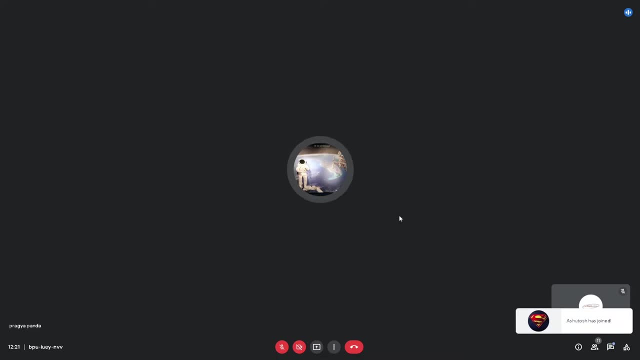 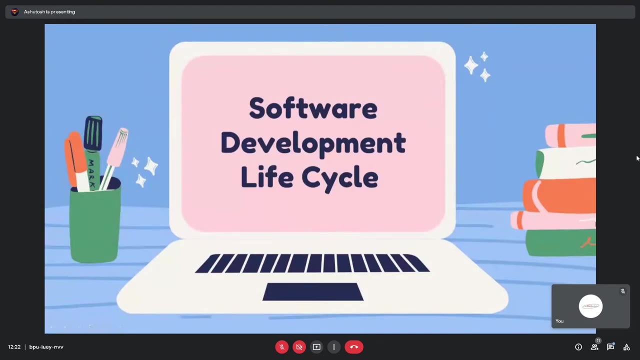 So these are different modules In the IT industry. if we are making a website, then there is a login page and a sign-out page. After the login, the page will come Okay, Which you also see in Facebook, which is a great example of this. 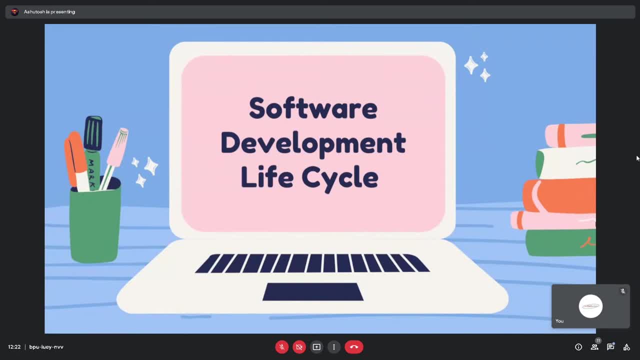 Okay, So to make all these things? it's not like we sit down to make it all of a sudden. Okay. If we sit down to make it, then it will go wrong. So for that we need a planning, we need a strategy that provides us with a software development life cycle. 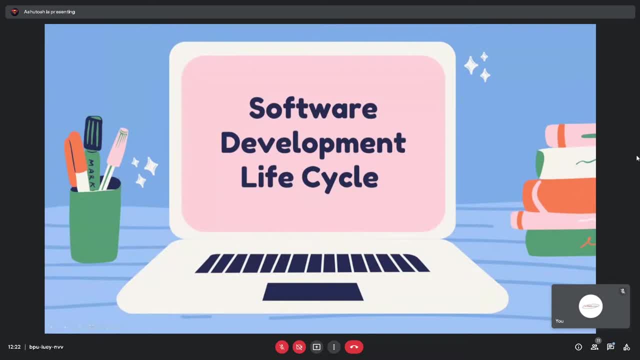 Okay. So, Ashutosh, can you tell us that why we need? because before starting anything, before applying, we should know that what will be the need for us to have a software development life cycle. But we need it, Okay. 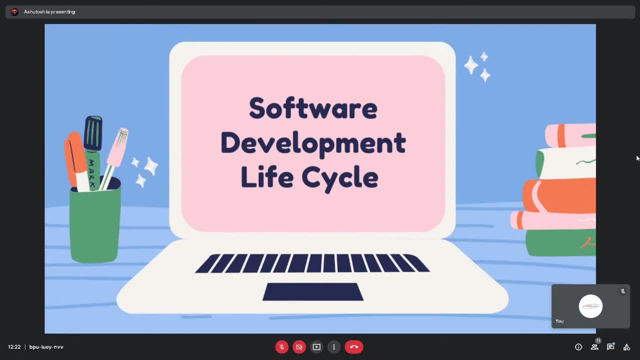 So why we need software development life cycle and what is the purpose of this. So, Ashutosh, can you tell us about this more? Yeah, Of course, I will be more than happy to tell you guys all about why not first. 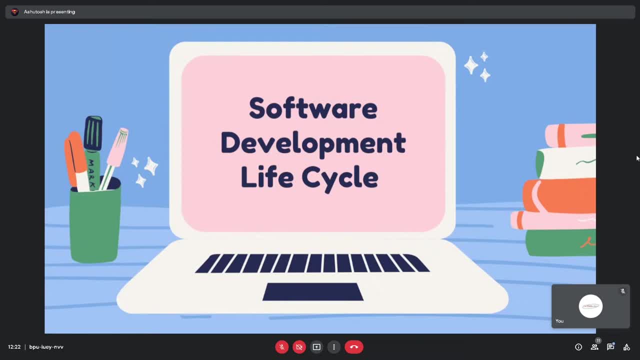 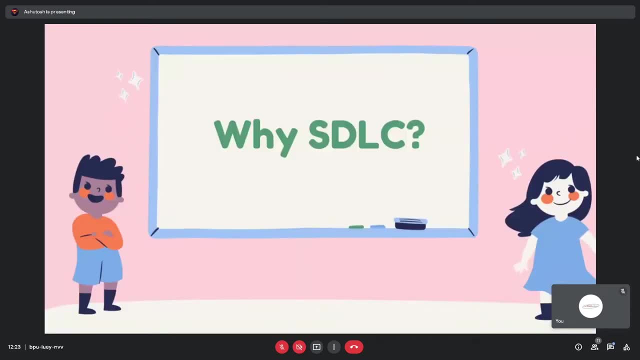 I will not explain first that. what is software development life cycle? Okay, guys, I will first say, like, why should we study this, or why should we know about this? Okay, So why Why SDLC is used? Anyone wants to like? 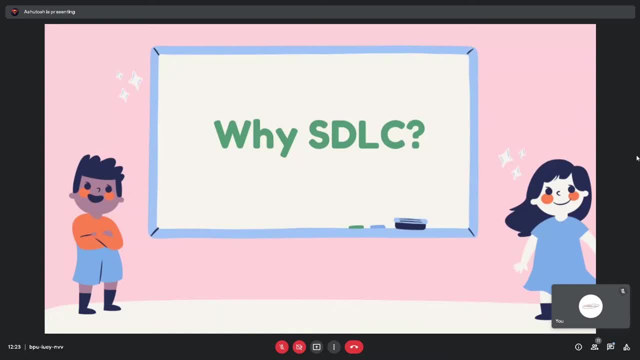 anyone wants to like share or like tell why sdlc is used? and uh, one more, like apology from my side that i will not be able to see your comment. so if it will be better, if you guys can unmute yourself, or if not, then my team will like convey, or pragya will convey that. what have you responded in the 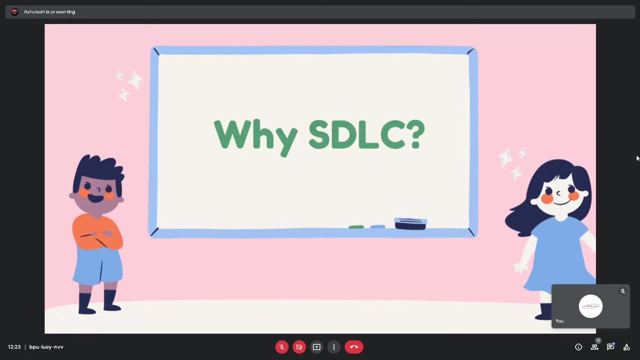 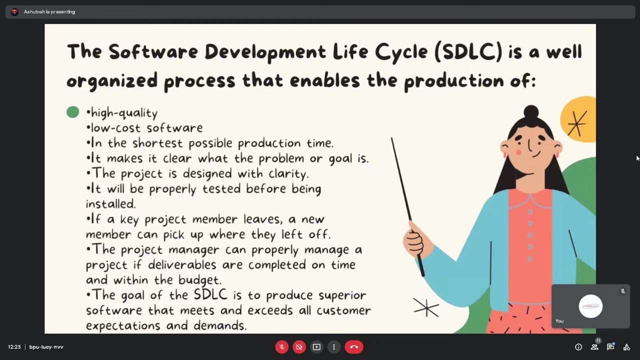 comment section, so i will like wait for three second. guys, can you tell why we need sdlc? okay? so, uh, no worries, i am here to tell you why we need sdlc. so see what happens now, uh, in any organization or in any company, in any business, uh. 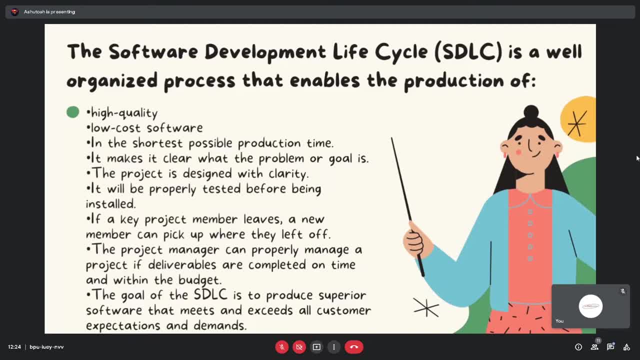 we will not go like we will expand, expand the money extravagantly, okay, so also like we will also want that, and after a year we are telling them that your product is ready, sir. that will not be like an acceptable thing to do, right? moreover, what sdlc like enables us to do that? suppose that you are. 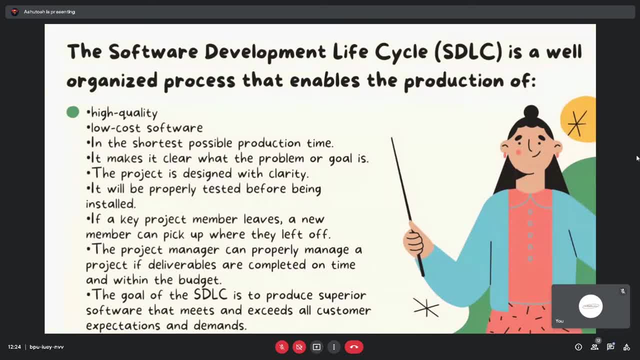 building something, okay, and you get, you got an urgent requirement to go somewhere else. okay, and you left that project in between, okay. so when the other person comes, how will he continue that if you have not properly documented that thing right? it is not like you have seen any code, or. 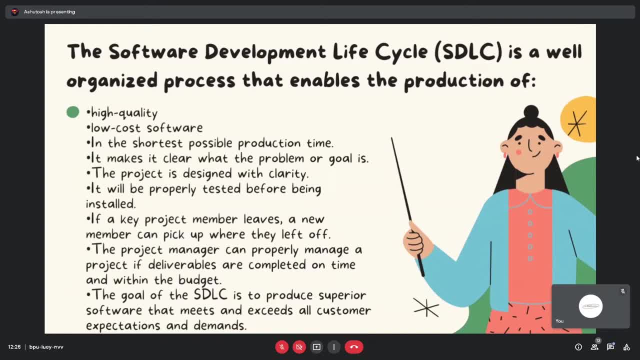 you have seen anything. whatever you are building, some other person can come and continue that thing without any specific document, right? so all these things that, how will we build our project? how will we ensure that it is of very good quality? how will we ensure that it is built on very low? 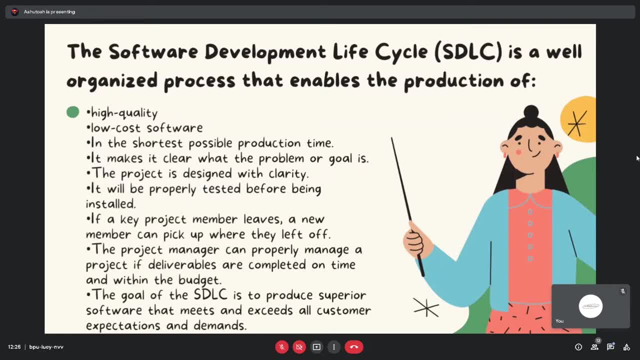 expenditure. how will we ensure that? how many resources we have. okay, guys, is it clear, like why we need sdlc in any organization and yes or no? yeah, kindly tell me if anyone responds yes or no in the chat section. yeah, definitely, please, guys, because that's why we are here. 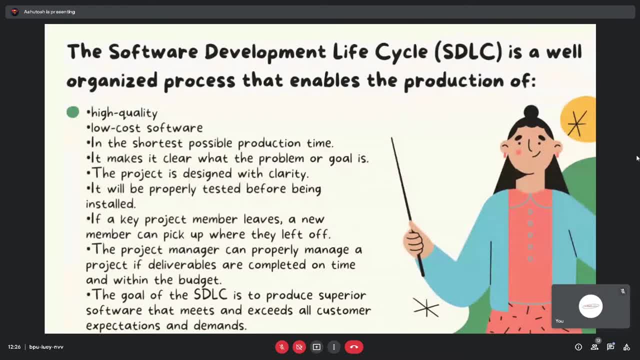 thank you, thank you. okay, yes, there is a yes we got, so, yeah, we can continue. oh, it pleases me a lot that you guys are understanding whatever i am telling. okay, so moving forward, as of now we discuss why we need sdlc, now we will discuss what. 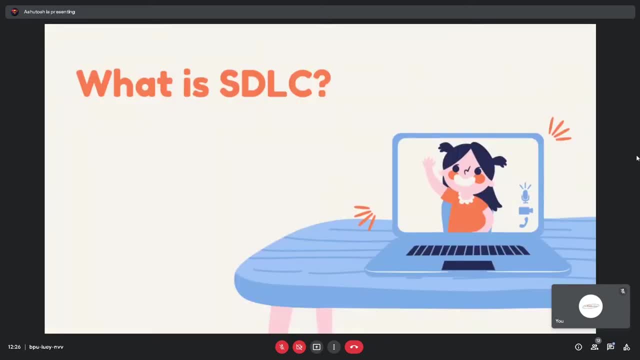 is this sdlc? okay, guys, so moving forward, we have to discuss this. what is sdlc? now again, let me ask you guys, like as i already told you why we need sdlc, can you guys now tell what is sdlc? okay, so in sdlc, you will be able to tell what is sdlc and what is why sdlc. 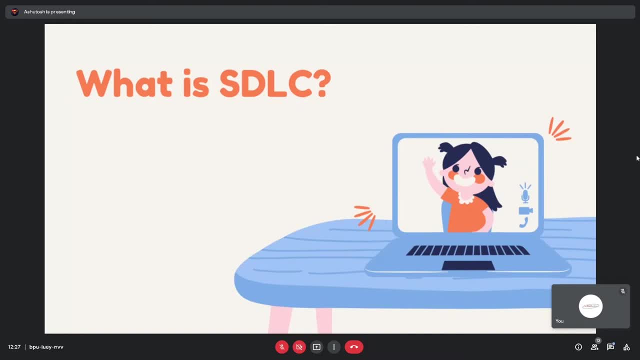 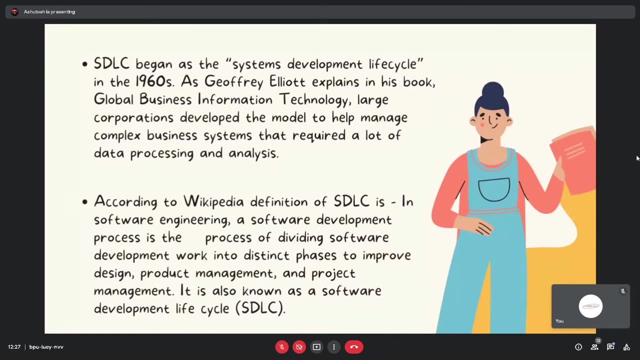 even if not, that's not a problem. that is why, like after this session, you will definitely be able to tell what and why is sdlc used in any organization. so don't worry, i'm here to tell all about this so earlier, like you guys can also read the things written over here. but anyways, i will like tell you. 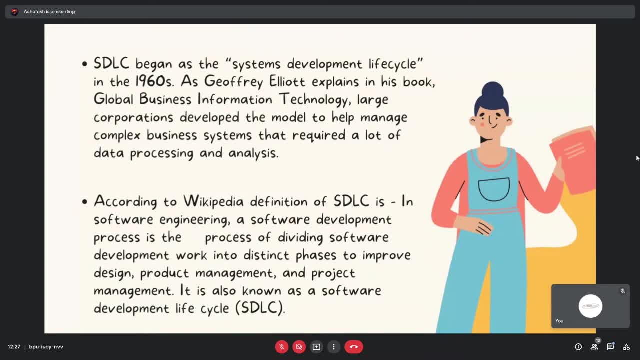 earlier. what happened now that there were like large organization also. okay, then for the first time, the first time they were using sdlc for this project- few small organizations emerged. okay, then the economist or the business person: they thought that how we can help these small organizations to develop or to grow, okay, so then they like 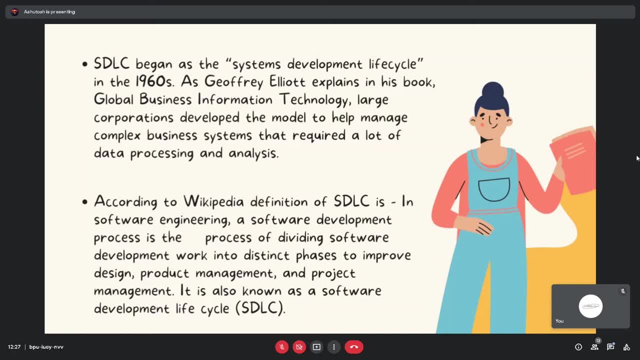 came up with an idea that system development life cycle, in that they like explained or like they wrote down all the things that how we can help an any, a small organization to grow. okay, so like when, i will like go with what is sdlc then, according to wikipedia, the simple definition. 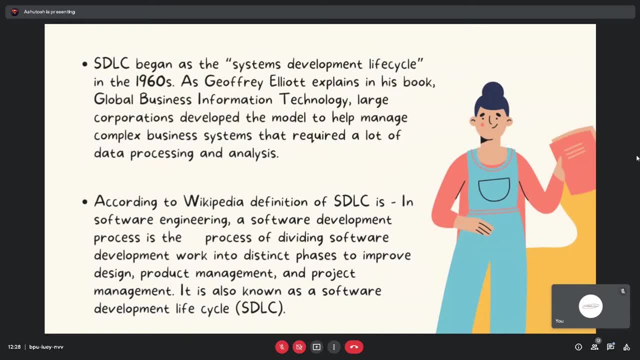 of sdlc is in software engineering, a software development process is the process of dividing software development work into distinct phases to improve design, product management and project management. it is also known as software development life cycle. so by this definition what we understood that in sdlc there are certain phases, right like how we will design our product. 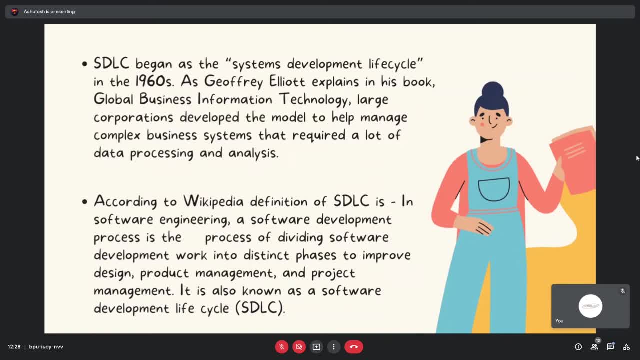 what are the requirement that we will need, how we will manage those things and our even after development, how we will maintain those things right. so all these things that is governed in sdlc are divided into certain phases. okay, guys, don't worry in like moving forward, we will tell. 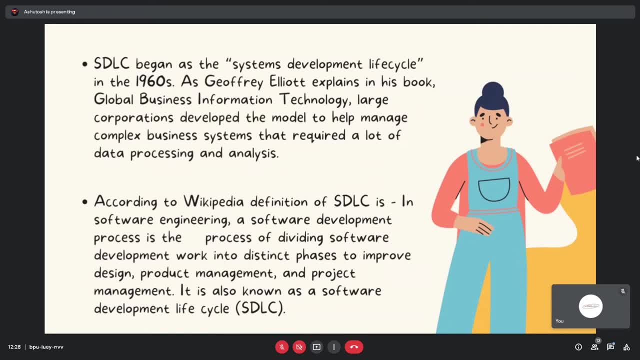 you about all the phases of sdlc. so, as of now, like. what is s sdlc? is it clear? like sdlc man, like. let me switch to the hindi and the lc: may hum kiya karte hai, hum ek. let's define this. what is sdlc? so like what will often happens in lighting, which is: 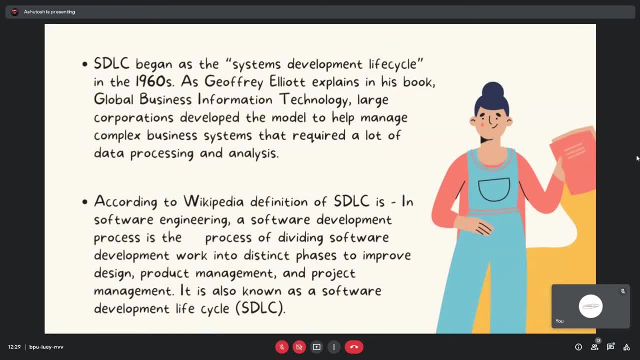 avlaunger: ok, he is theuito unclean. and what will happen here in hardware, electronics patients, okay, summers, and i and i teach you to ride. so there, ecosystem, there are almost in these type of chapter, da fall drinking this last. you know the question? the question, cuz we don't focus on the result itself. this will jeunes racism which manufacture. 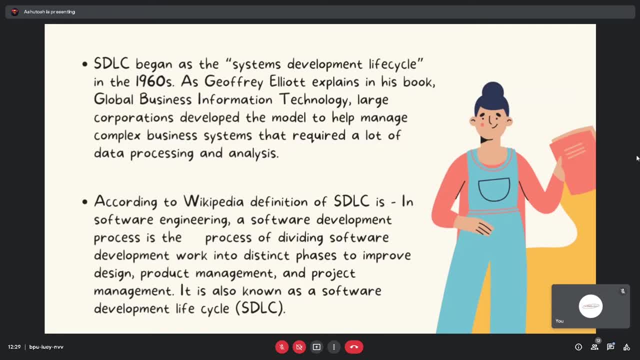 oh, we accept and test that. okay, guys, elements that are to be directed to our ends will provide and like, because, like, if you guys, if, if all of you guys have to say yes or no, because we can't proceed further. if you don't understand right now what is SDLC? 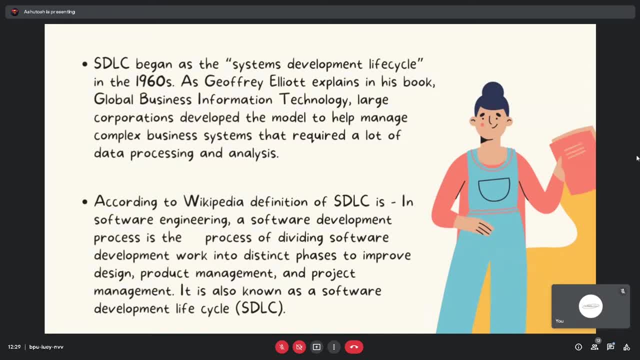 so kindly to respond yes or no, that you guys stand. yeah, we got one response from Magnesh. okay, what about all those guys? at least tell yes or no, because before moving forward I want to ensure that you guys are understood. what is SDLC? Anuja, can you understand what is SDLC? you just need to type yes. that much is enough for us. 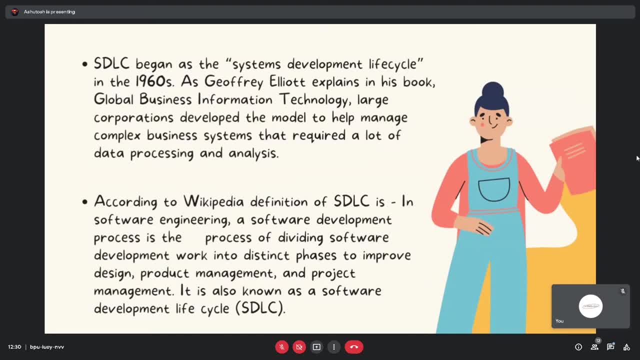 to move forward. okay, yes or no, especially yes and you didn't understand, yeah, like if you have any doubt, you can definitely say no, that I am not understanding. if you want to ask, you can unmute or you can type the question in the chat section and also please fill the attendance form. 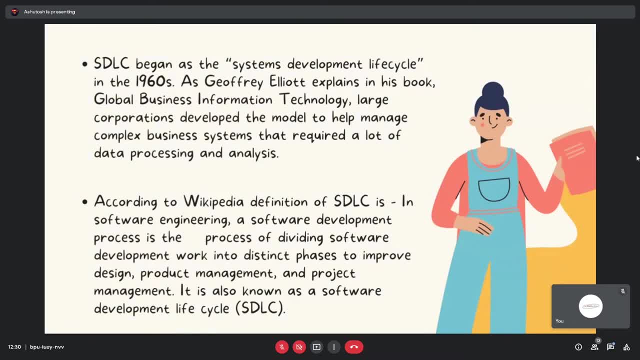 okay, we got enough. yeses, I think, yeah, you can move on. yeah, moving forward, guys, as of now. I told you why SDLC is used in any organization and what is SDLC. yeah, I think that you guys might be thinking that, yeah, the why and what phase are. 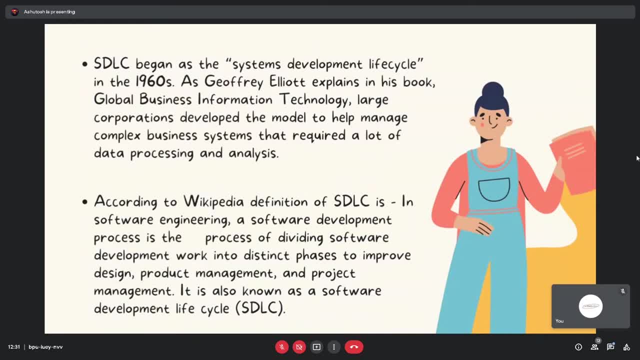 like similar, but no, there is a difference. of course. there is a difference in why we learned that, why we specifically need SDLC, in and in what phase we learned that. what is this? okay, what is this? by this I mean SDLC. so, moving forward, as I told that there are certain phases or stages. 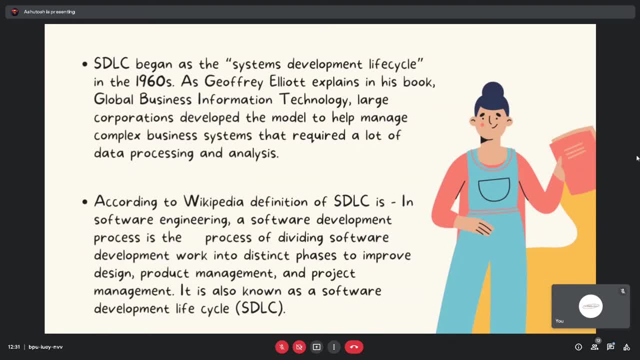 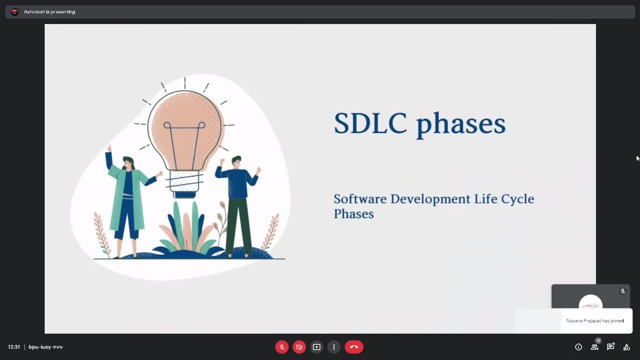 in that any any SDLC process. okay, so moving forward, I will like jump into as DRC phases and for like for you guys to explain, like to tell you that what are the stages or the phases in SDLC. I will like invite Pragya to start with this. thank you, Ashutosh. so, before we proceed, what can we come to? how can we talk about this? 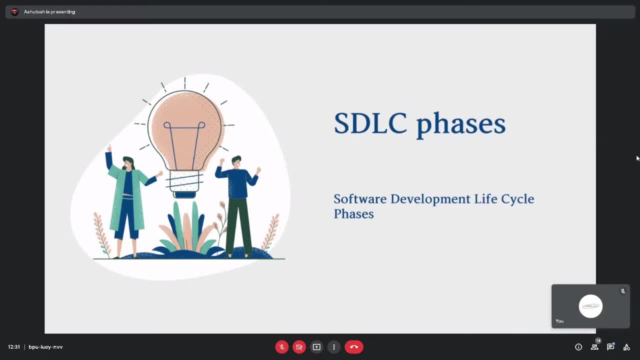 thank you, Ashutosh. so, before we proceed, what can we talk about? so, before we proceed, what can we talk about Now? we will continue with the help of what phases or what are the strategies that we can follow to implement SDLC so that our project can come out beautifully, because ultimately, that is our target. 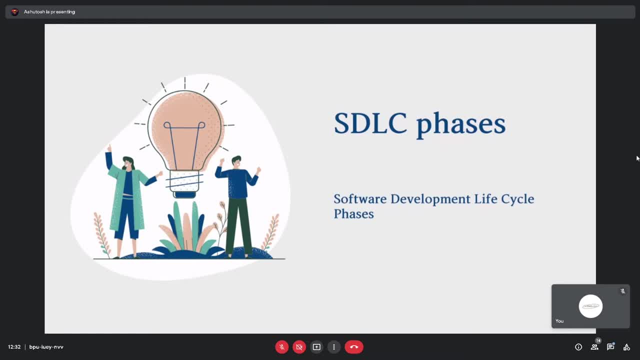 So, before I proceed, this is a simple question, at least I want everyone to unmute and answer it, and I will be very happy if that happens. Okay, so tell me which is everyone's favorite food Like. if you ask me, I like Shahi Paneer very much. and what about you guys, Anuja, what is your favorite food? 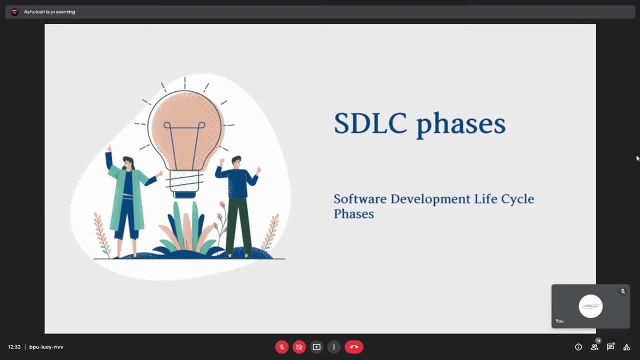 You can unmute or you can type: Sobham, what is your favorite food? Chicken or biryani? Wow, that's awesome. Nice, bro, nice. This answer won my heart. Yashashree, you want to say something? What is your favorite food? 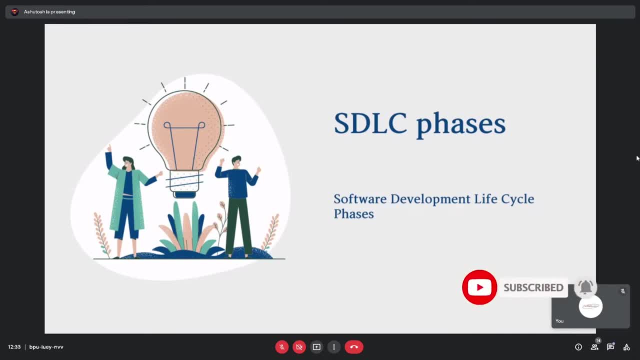 Nayana. what is your favorite food? Guys response: Magnesh Badshah. Awesome, Welcome to the session. What is your favorite food? Chicken Biryani. What is the only food you like the most? Biryani. 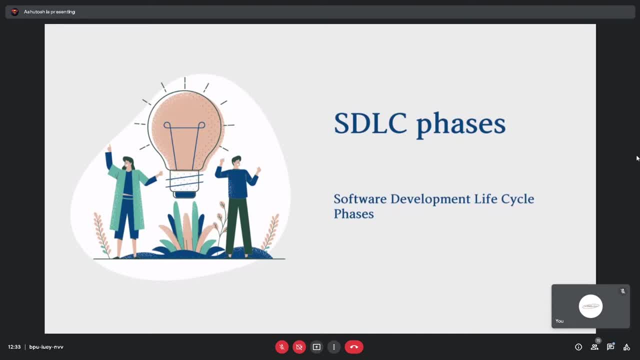 I think Vik Unreal has one very specialelliang food. Ah, that's a Punjabi boy Got it. Awesome, awesome, Delicious. Thank you, Prem Raj. Okay, until now we have chicken bhature and biryani bhatura hai biryani hai shahi paneer, aur kisi kuchh pasand hi nahi hai as the discussion 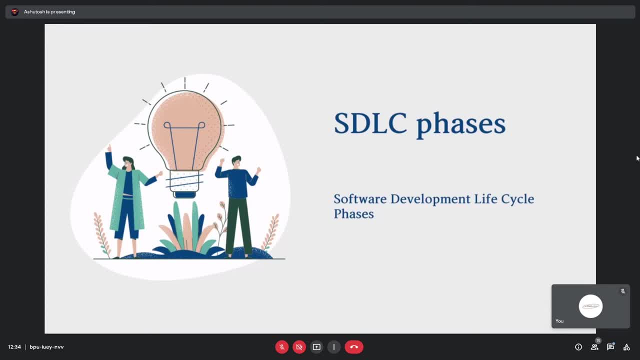 about food is going on, so, like i will like, i will also like to add that my favorite food is also sahi paneer and yeah others response like you can type this in the chat, guys like: what is your favorite food? sab healthy diet follow kar rahe hain? yeah, sabhi abhi ghar. 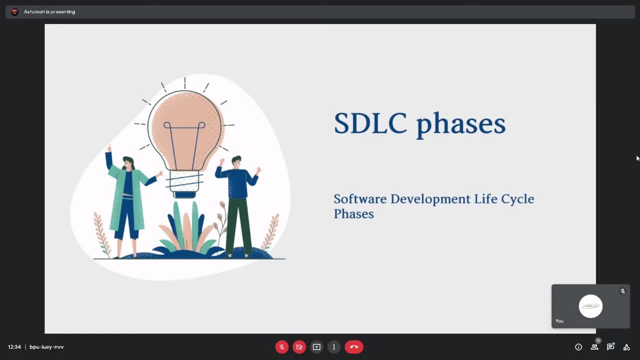 par rahe, ke like dieting karne ka soch rahe hain healthy chane chaba rahe hain. guys respond: lockdown mein unhealthy hoga hai shahsa, unhealthy hone ke babajood bhi jawab nahi hai. simple se question hai. 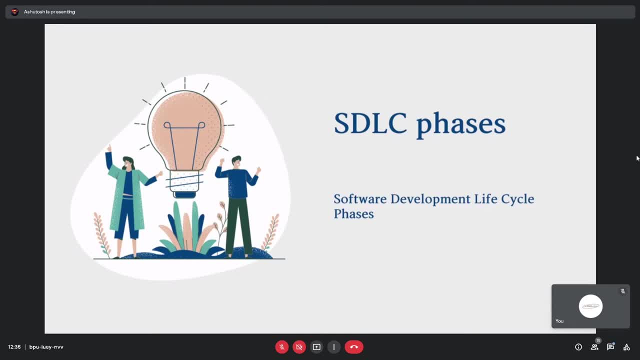 esperiment zyada ho rahe hai, lockdown mein chalo. let's we take an example of biryani chika hai, toh jab hum biryani banate hain, toh hum yato ek din pehle decide karenge. 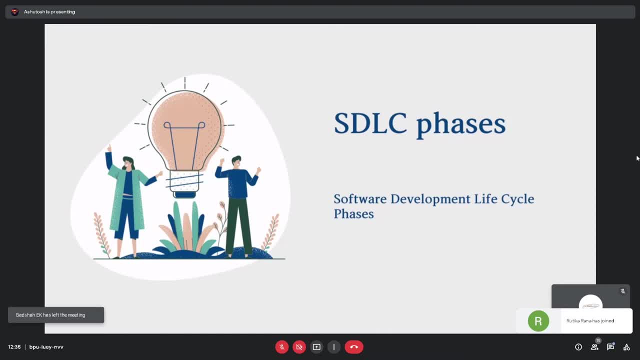 yaa, usse welcome, ritika reyna, apka favorite food. kya hai session continue karne se pehle hum sab ka favorite food pooch rahe hain. taaki zomato se deliver kar sakhe aur attendance ka attendance bhi bharde. je, taaki zomato se deliver kar sakhe aur attendance ka attendance. 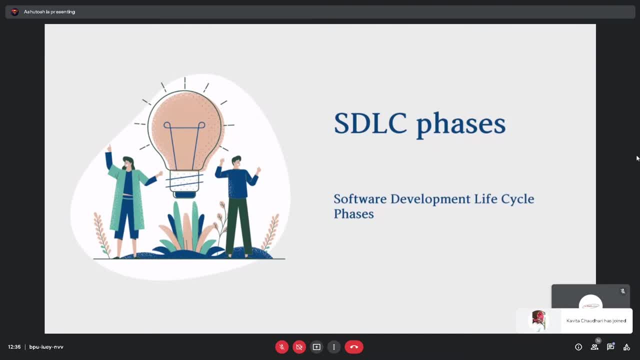 bhi bharde je taaki, zomato se deliver kar sakhe aur attendance ka attendance bhi bharde je taaki, so that I can reach you easily. Kavita, welcome to the session. What is your favorite food? 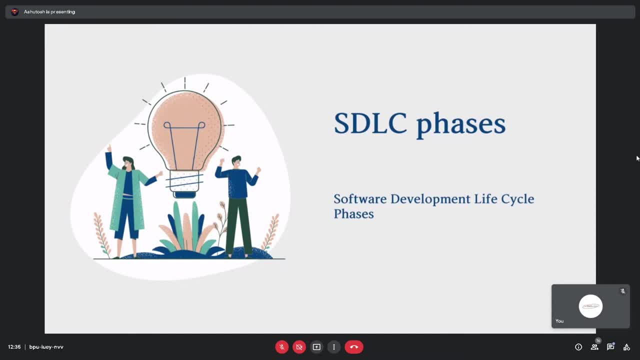 Type it. You don't need to unmute yourself, You can type it. Okay, we will go with biryani, Because it is a very awesome dish. It takes a lot of time to prepare it And it should be perfect. 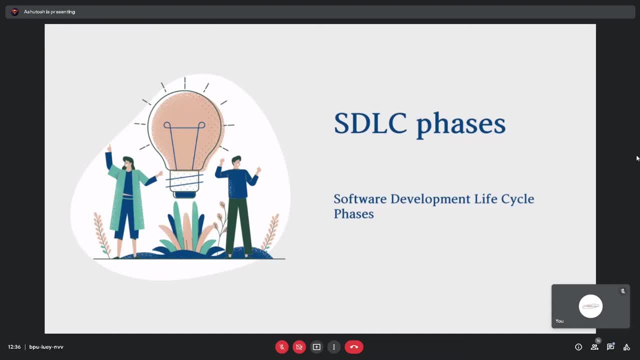 Otherwise the taste can be different. Okay. So the phase number one of SDLC. or when we are making food, Okay. Or when we are making a website, Even if Tesla makes a car or any automobile industry designs anything Before that, there must be something. 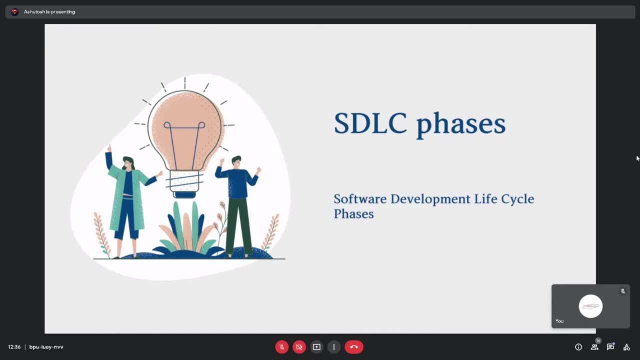 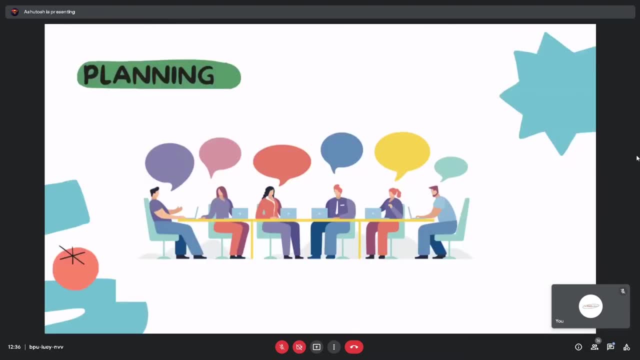 What do we need When we do a trip? first of all, what do we have to do? Planning, Correct, Awesome. So our first phase is planning Where people meet. they decide that we have to make a budget When we go to Manali. 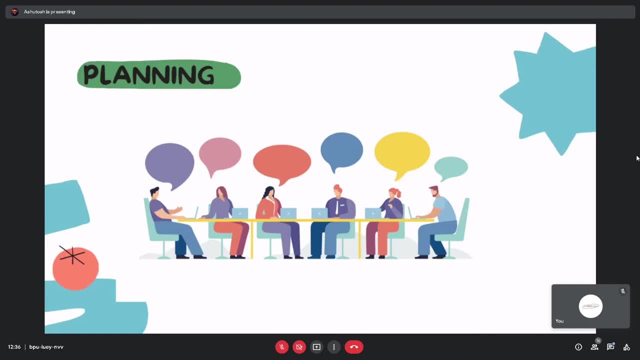 we make a budget. How much budget do we have to make, Who will come, Which friends are coming, How long will it take And how to travel right? So if we talk about biryani, then we decide which ingredients will be made. 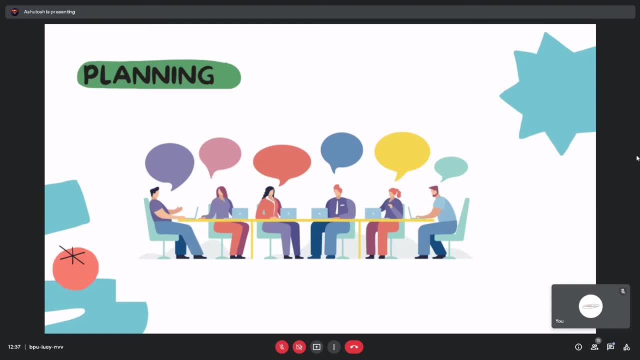 We have to buy, of course. And which YouTube channel should we watch? Because we don't know how to cook biryani. So which one will be good? Kavita's Kitchen or Nisha Madhuli's? Okay? 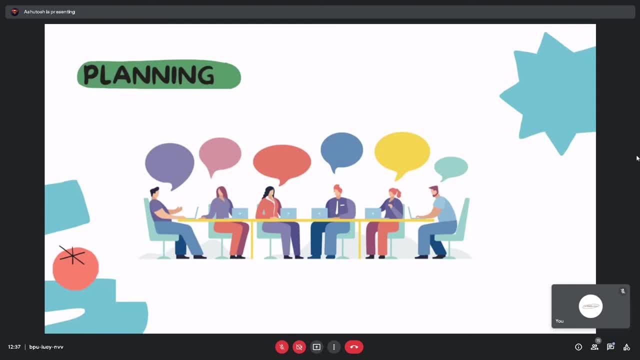 So in this way we plan what we need. Similarly, in IT industry and all the big organizations they follow this planning rule first in the SDLC. So in this they discuss about the budget, Staff and timelines. Okay, 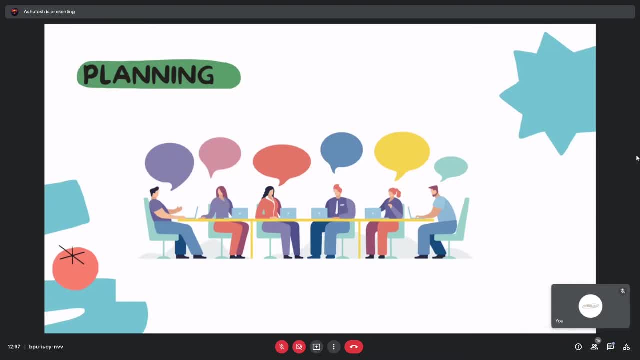 So they decide how much time it takes to complete that particular module or that particular project. We cannot say randomly that we can complete it in two years, because that is a very big time. So we decide a small time frame, for example 6 months or 3 months. 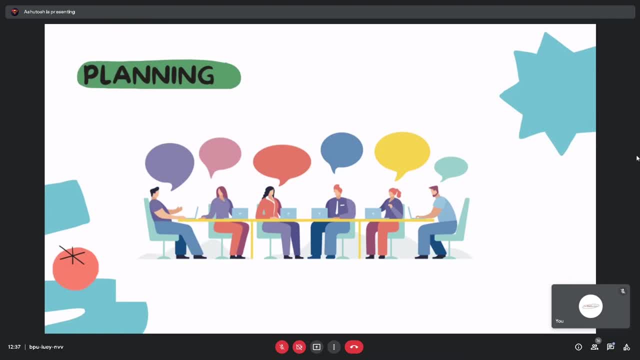 as it is discussed. in that discussion. The budget is decided, how much money will be spent to make that project, And the staff decides how many developer teams are needed and how many tester teams are needed to test it. For example, Sovam has made biryani. 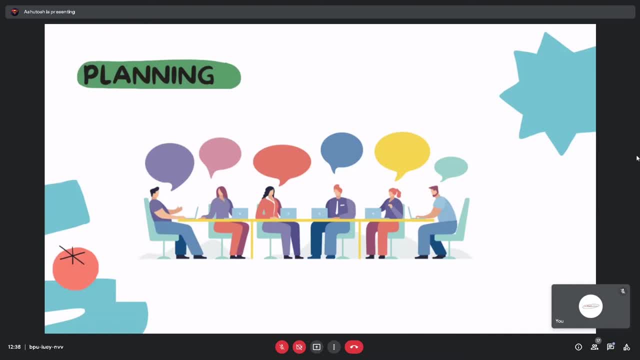 He needs a tester to test it, And Sovam is a developer. He has made biryani. So in this way, similarly, we have to decide while making the projects, how many testers are needed, how many developers are needed. when should the deployment take place? 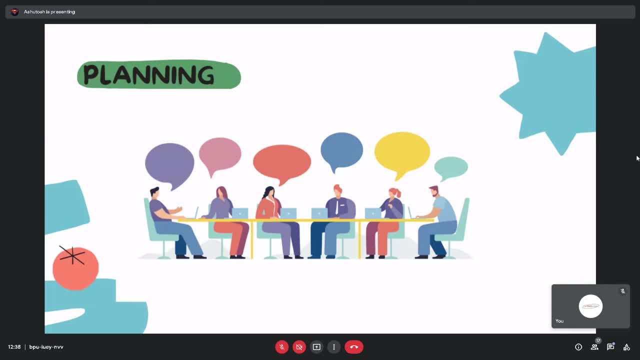 and if there are bugs during testing, then the duration increases, But we don't consider that It is an approximate. the timeline is decided And all this activity is happening during planning. Okay, After deciding which spices to add in the biryani. 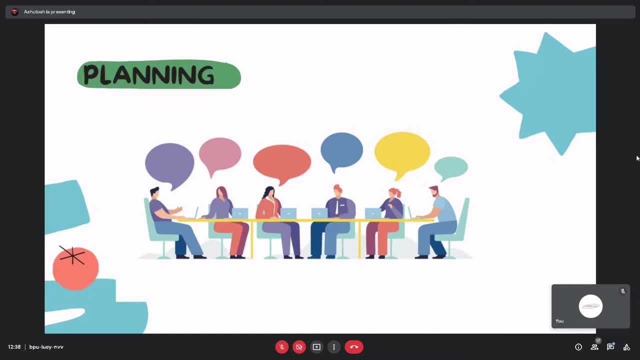 and which login pages to make in the websites, which introduction page to make. after doing this planning- complete planning- we will move on to the next, which is analysis. Ashutosh likes Shahi Paneer and all that thing. So you tell us how you analyze after planning. 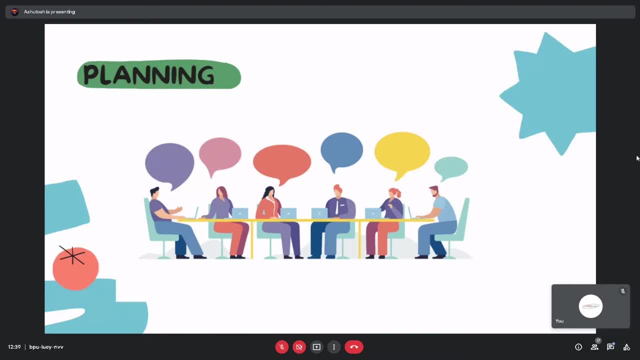 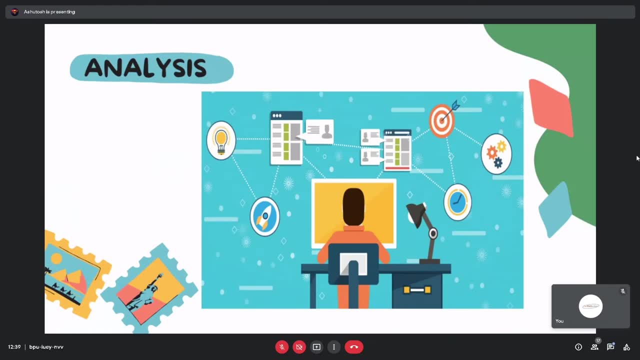 That particular thing, Or after you decide that, if we are going to create a website or application. So after that, how do we analyze the whole process? How do we continue further? And please fill the attendance form. whatever is here And we will be very happy. 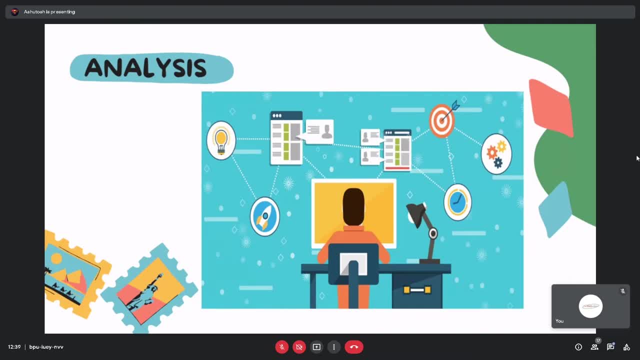 And yeah, Ashutosh, you can tell us how your analysis is done. Yeah, Yeah, So any like guesses after the planning, that why we are going into the analysis phase? Like, as Pragya told you guys that, what are the things that we do in planning phase? right, 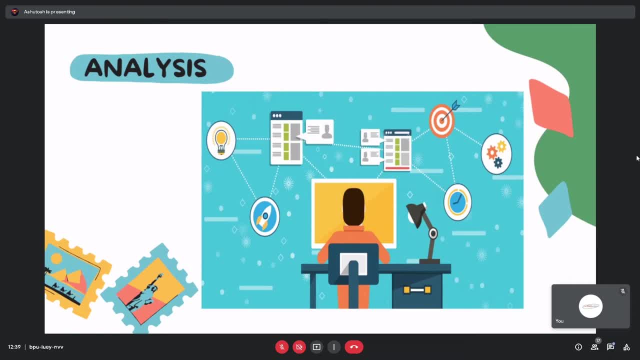 We gather all the requirements, like we discuss, we brainstorm and all those things with our stakeholders, with our manager, all the developer team, tester team, all those people organized together and like discuss or brainstorm all the requirements and planning phase. Can you guys now tell what are the things that we are going to do in analysis? 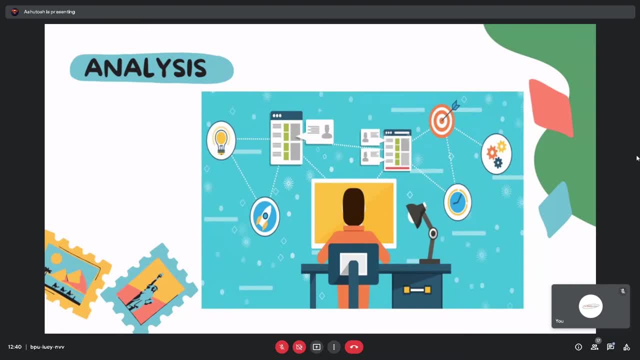 Okay, There is a simple thing: What we do in analysis phase is that all the things that we have planned out in planning phase- Okay, All the things that we have planned out in planning phase. One simple thing is that we write it down. 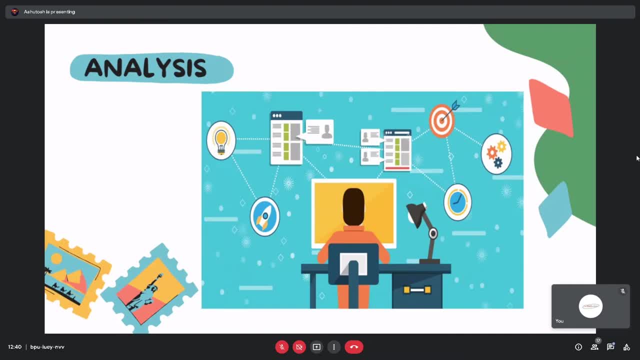 Like, if you remember my experience of my childhood, So I had just told you guys that when I was doing group project in childhood, when we discussed things and then when we started working on those things, we had not written all those things, So we forgot a lot of things. 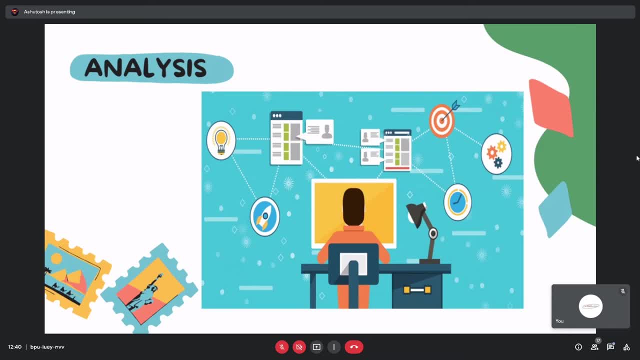 Okay. So if this does not happen in an organization, what we do for this is that we prepare a document in analysis phase. Okay, And that document is known as software requirement specification document, In short, SRS document. Okay, guys. 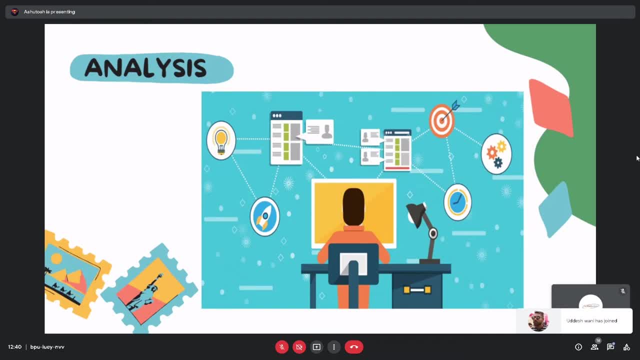 In that document we write down all the things that we have brainstormed in planning phase. Okay, Moreover, in analysis phase we also analyze that what software or product development we have done. whether it is economically feasible or not, It should not happen that we are doing such a project. 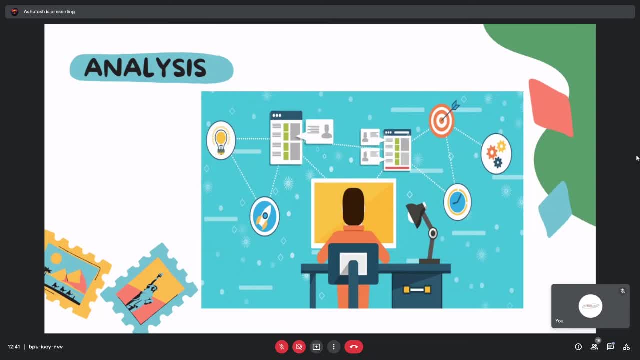 due to which our company is at loss, Like its expenditure can be higher than our afford or GDP. Moreover, we have also like to cover the legal procedure. Okay, We can't use any licensed product without purchasing the license Right. So all these things like, moreover, 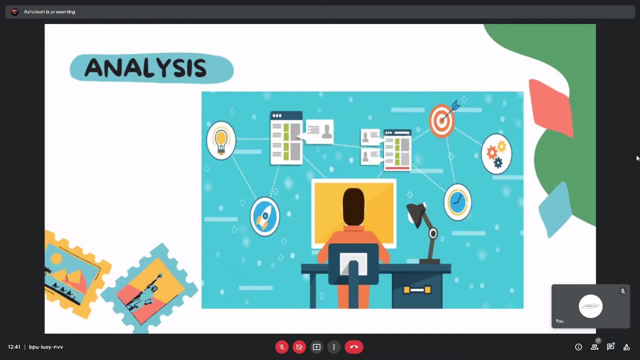 all the other things that we do in analysis is that we also decide that our technical staff should be of which level, Like what would be the requirement of the software developer. Okay, Moreover, in analysis phase, which is our software requirement specification document, 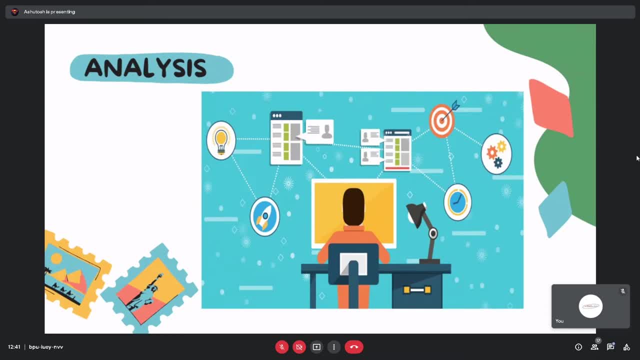 we will also write down these things, that our schedule will be, that how much time this whole process should take. So, in simple point, in analysis phase, all these things that we discussed in planning phase, Okay, We organize that, We write it down in an organized way. 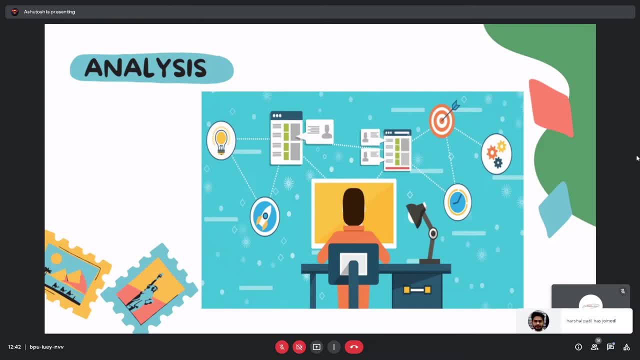 Not in much organized way, Okay, But all the things that we discussed we write them down in SRS document, Okay, Is it clear, guys, That what we are doing in analysis phase- By I mean organization and all the business people- 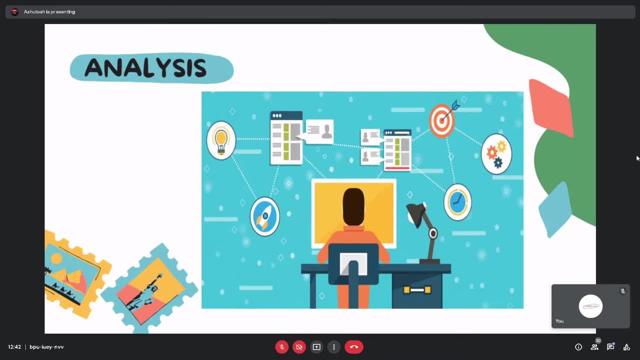 Is it clear, guys? I want to see your point of view. Yeah, Sure, Sure. So in analysis phase we use agile scumming model for analysis purpose. As a normal person, we use Trello as an example. So if you go to Trello, 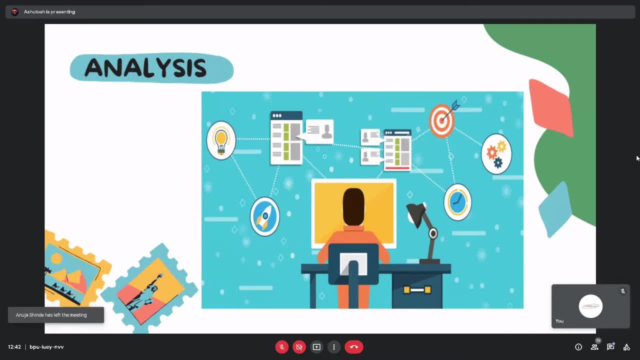 we also do analysis from there. So mostly in analysis phase we just see what we have to make, what analysis we have to do. There is a particular check point After that. there is a particular duration. It can happen after every day. 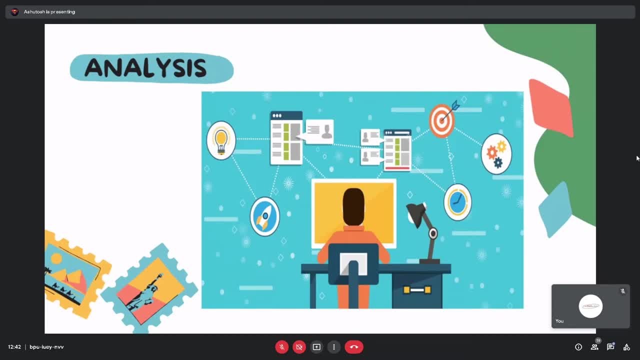 There are team meetings. After that we do analysis That particular check points will not be fulfilled. for us This also happens in analysis phase. That means check points which we already add break points in projects. So nowadays it is used in many agile scumming models. 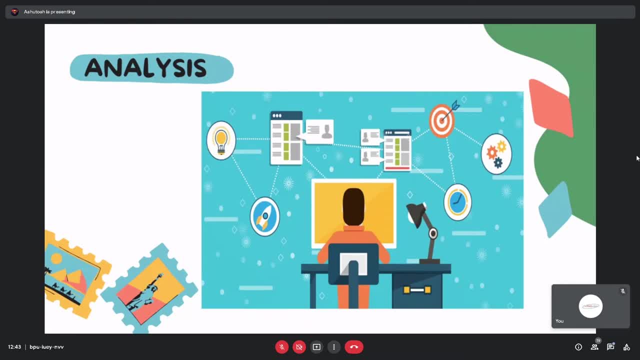 Like Trello is also there. Trello is an example of this, So we also use it there. So, in progress, what we have to do and what has been achieved- in front of us, Of course, Like really valuable information. 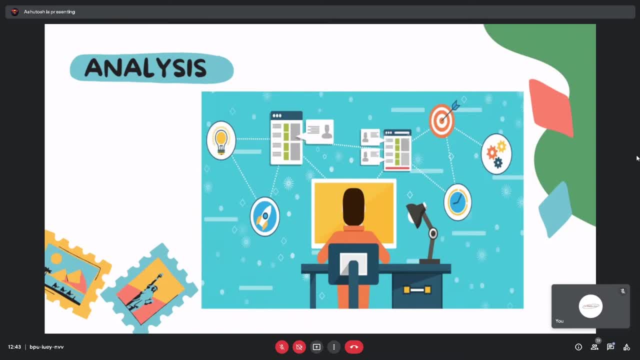 May I know your sweet name, bro? My name is Sobham Pradhan. Yes, Please repeat again, My name is Sobham. Is that audible? Yes, Sure, bro, That's a nice name bro. Yes, All the things that you told. 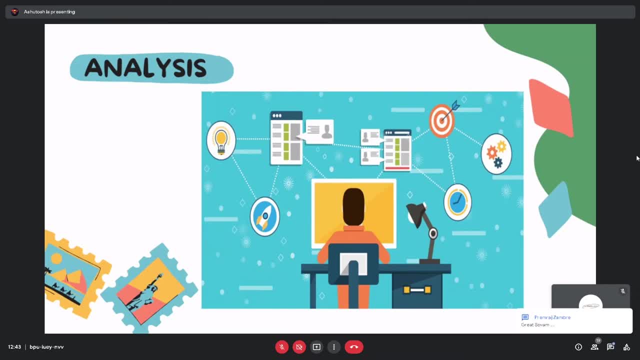 at the check points and using of Trello. You already told, bro, that you yourself told that this is a methodology Right, And we haven't been like, we haven't gone to that phase where we tell you what methodology we use in SDLC. 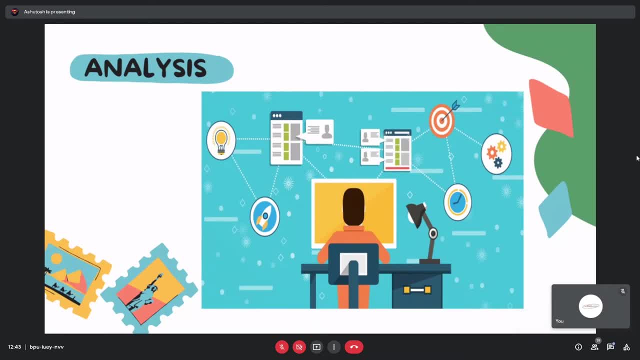 So, like all the things that you told is absolutely correct, Okay, But have some patience, We will reach there. Don't worry about that. Right now, what we are discussing are the phases of SDLC. This is a generalized term, SDLC. 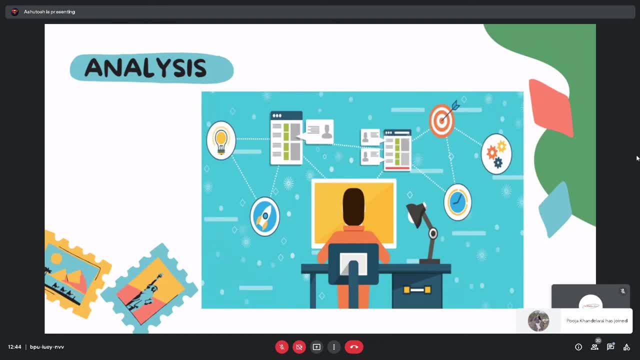 Of course, there are many more methodologies in SDLC, For example, Waterfall, Agile DevOps That you told about Agile, Right, So don't worry about that, We will reach that part also. And, yeah, your point is absolutely correct bro. 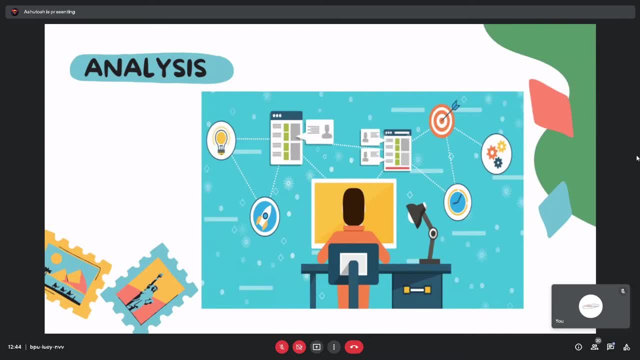 Don't worry about that And really thanks a lot for like bringing this up to the light for all our audiences. Okay, So moving on to the next part. So, okay, So moving forward. Yeah, Sorry, Okay. 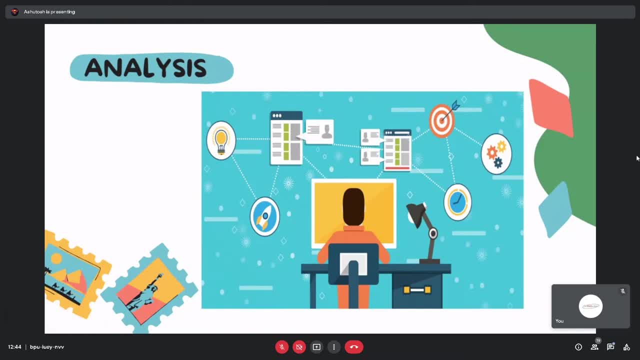 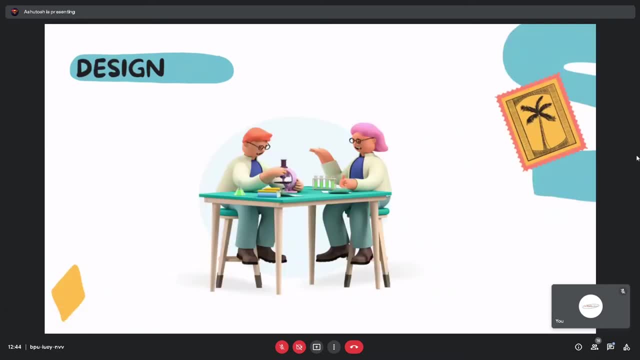 Moving forward. after analysis, we have our other, our next step or phase, that is design. Okay, So this is also very simple step. As I already told, I am audible. guys, Right, Yeah, Yeah, As you touch. 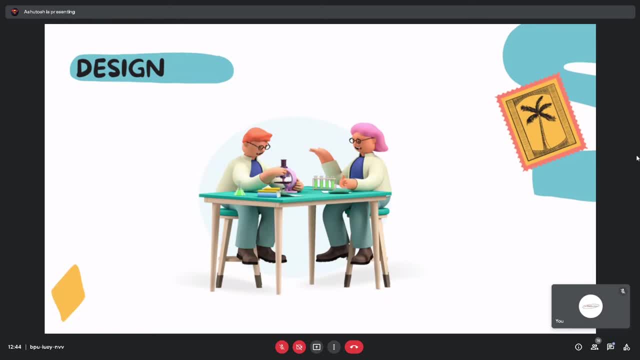 you are audible, Okay, Sure, In design there are a lot of things that can be done. So in design phase, what we do, that in earlier phase, what we did in our analysis phase, we were preparing an SRS document. 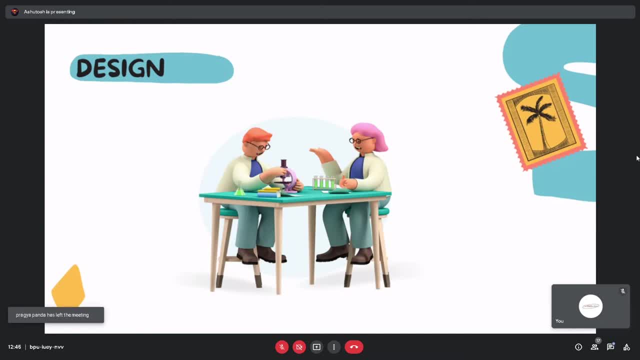 Right, And I also said that in planning phases, all the things we had planned after brainstorming, we have documented it in SRS document. But there are a lot of things in it which are not filtered Like. there are a lot of things. 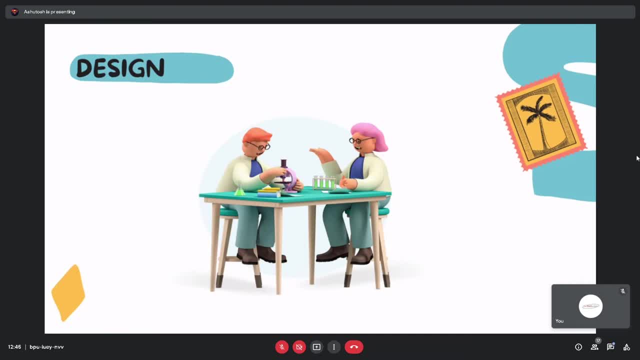 which are unnecessary. There are a lot of things which are not feasible to implement. Its operational cost will be very high. It is not legally possible, Some of the expected things which cannot be fulfilled. So all these things we have to do it outside. 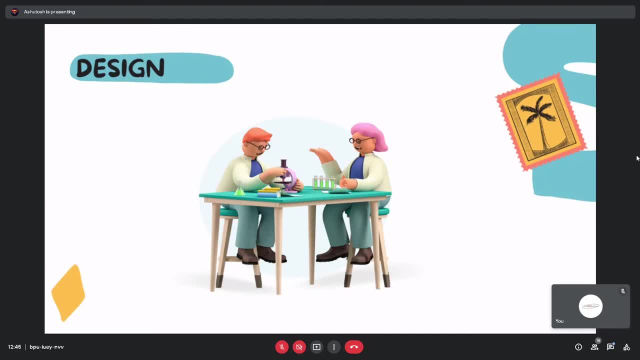 Right. So in design phase we organize our software requirement specification document in a very good way And we name that document as software design document. Now, when we have prepared our software design document in design phase, Okay, After this, all the phases. 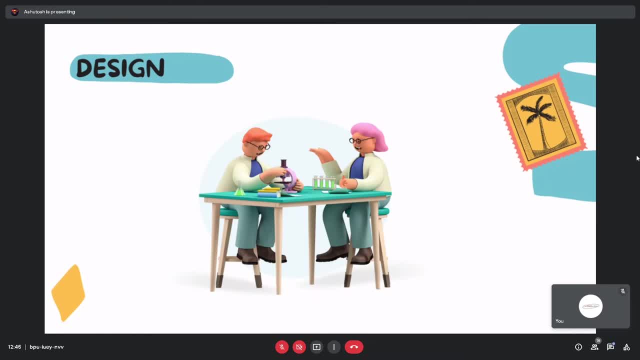 okay, In all those phases we will use software design document only. Okay, In software design document we write all the things that how our user interface will look, Because obviously when we are developing any software we want our end users. 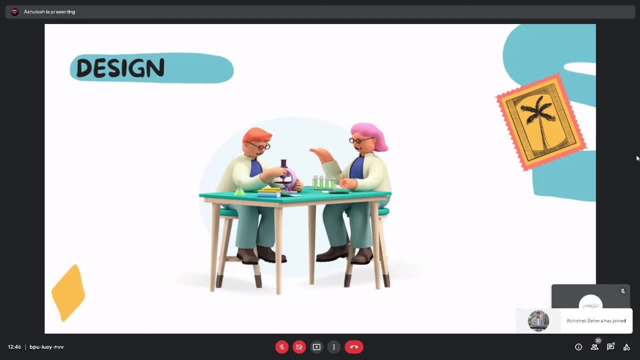 to use it very easily. Right, It should be self-explanatory, Like: here you have to click on yes, here you have to click on no And all those things. Right, It should be readable. Okay, Moreover, the interface that 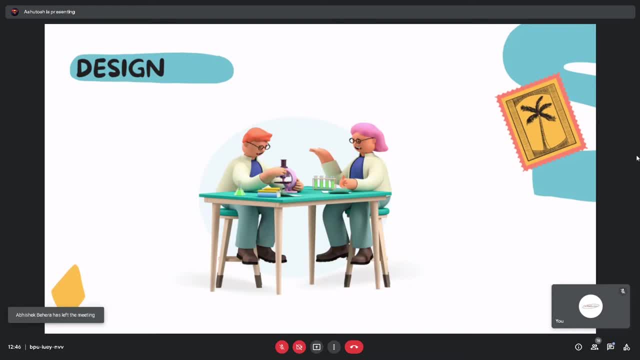 the user are facing all those things. the design aspect- Okay, That design aspect should be perfect. All these things are like documented in the design phase. Okay, And remember this point: In in analysis phase, we build a. 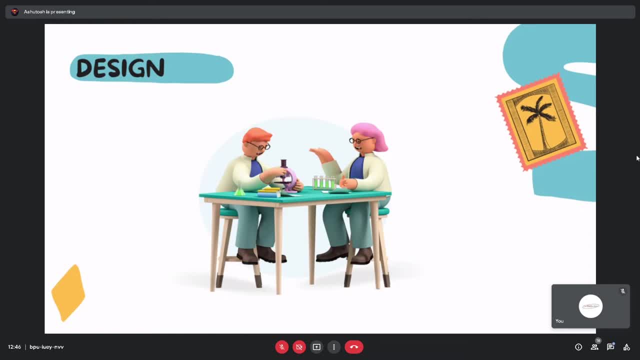 SRS document right And in design phase. we will organize that document and we will organize the documents that we are planning in design phase. Okay, guys, For the next phase, I will like to call Pragya, Pragya. 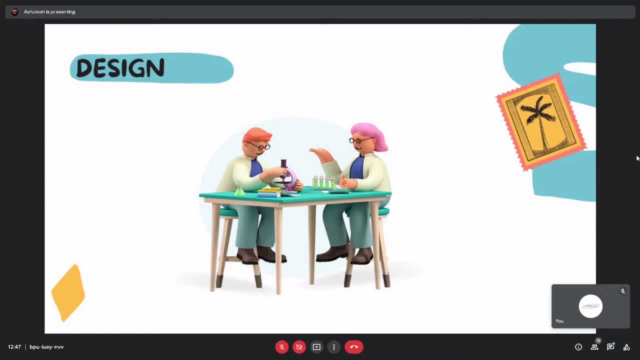 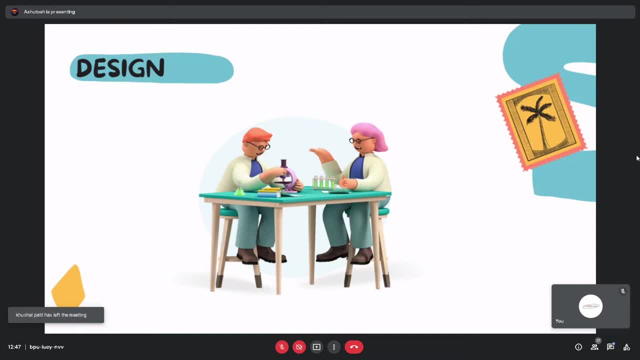 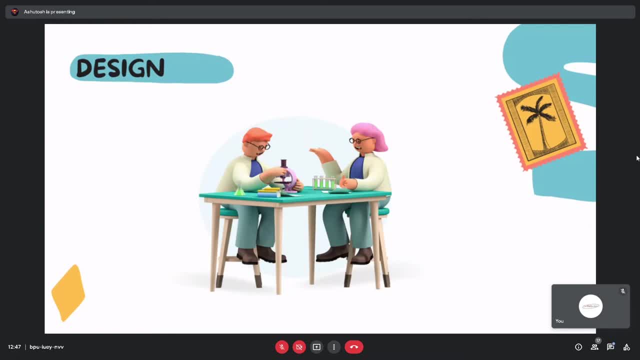 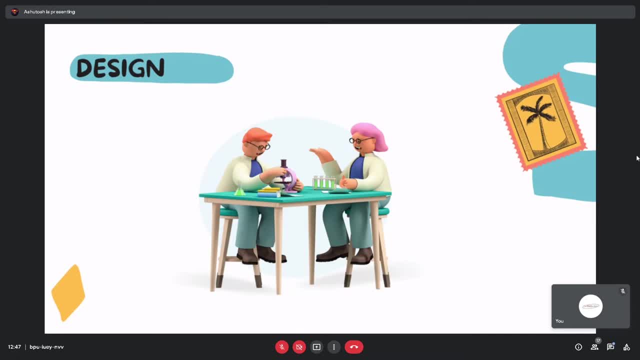 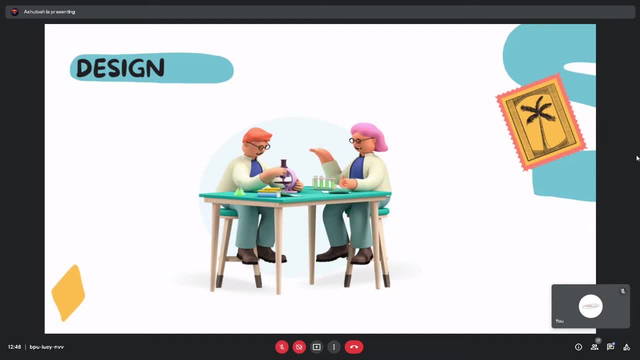 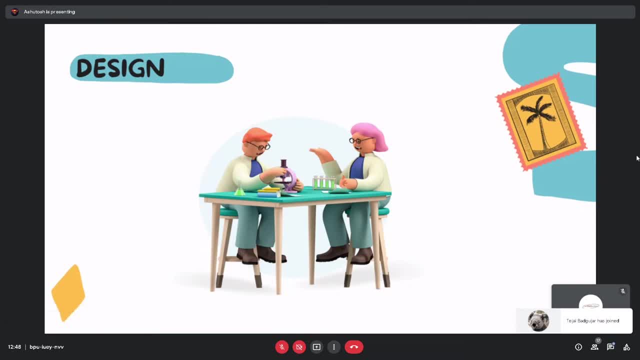 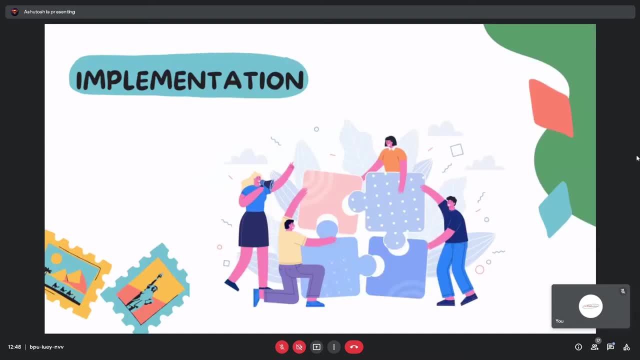 within a particular time frame. Now, whatever software design document we have made in it, we will implement it. So our next phase is implementation, where you are seeing a beautiful diagram, a beautiful picture, where, whatever people have learned, they have implemented a puzzle. So whatever we have decided in the design phase, it is like a puzzle Until. 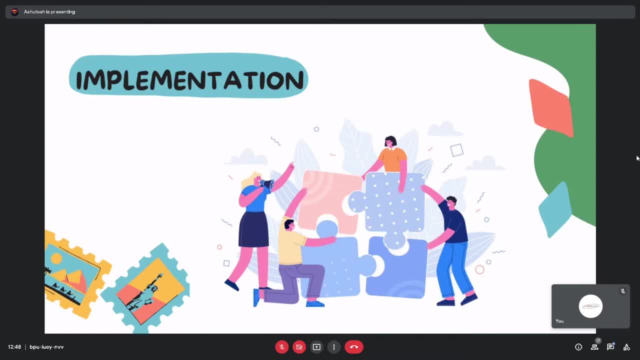 unless we join it together, it won't come as a complete picture. okay, So what the developer does here is, whatever has been decided, that you have to make a login page. there should be a button in it. there should be a user name. you have to make a registration page. 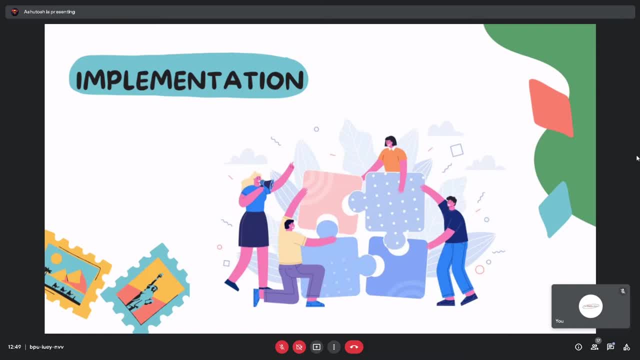 or you have to make a card section. Whatever has been decided, we will implement it in this implementation phase, especially W2W2.. Ok, OK, Ok. So, after completing this implementation phase, our development is done. the developer has developed it. now is it right or wrong? who will check it? 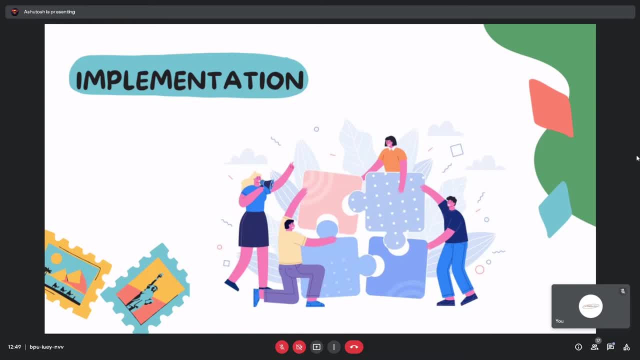 Food is prepared. come on, leave it. who will check the code? we will see later, Mummy as a team leader. Very awesome, awesome answer, thank you. So now mummy will test and tell how it is made: less salt, more chili, whatever it is. 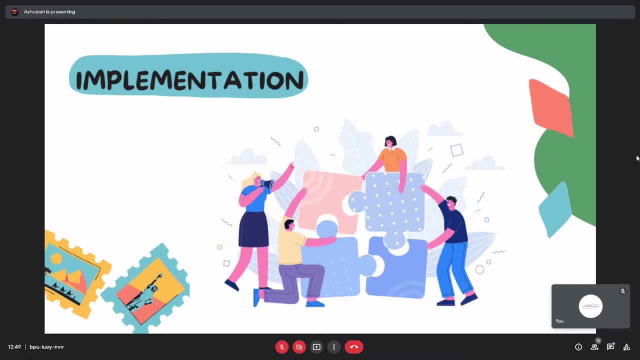 Similarly, there are testers in our industry who test and tell that whatever the developer has designed, is it according to the software design document or not? If it is a little wrong, it is called as a defect and it has to be corrected. Until this correction is not done, 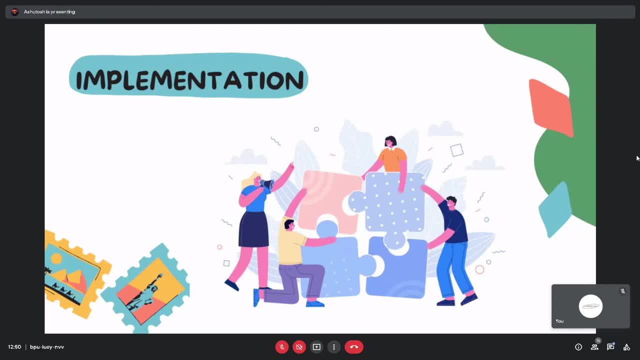 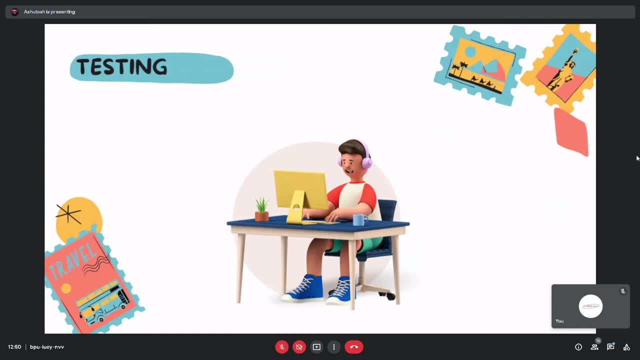 Okay, So it will not go to the second phase, which is the phase after testing. So, Ashutosh, you can. yeah, thank you. So the tester is doing the test while listening to the music, but it is not that easy job. 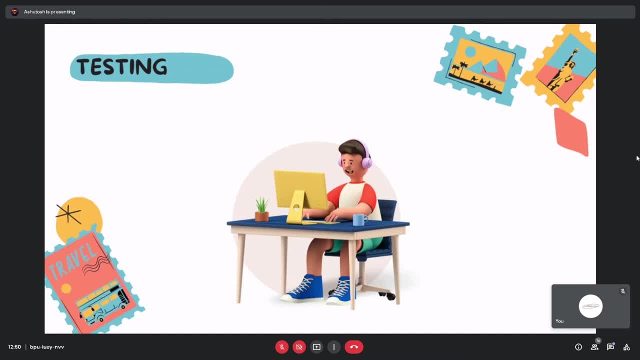 Okay, So he does the testing. tells what errors are there in the code. what are the drawbacks? cannot give suggestions, of course, 100% bug free project. It can never happen that there is a 100% bug free project. 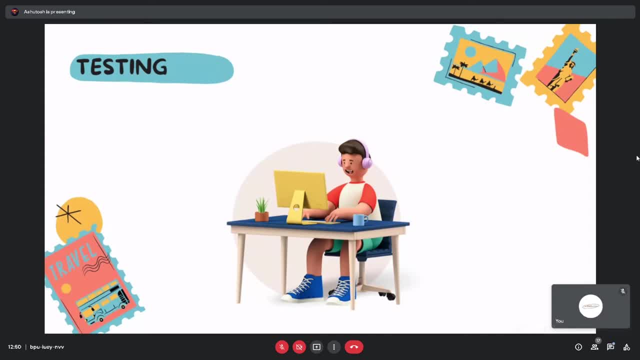 Okay, We can lead to 100%. It may be 99.9999%, so many nines, infinite nines, but it can't be 100%. Whatever we test, it can never be 100% Okay. So when it does not reach to 100%, we cannot deploy it. 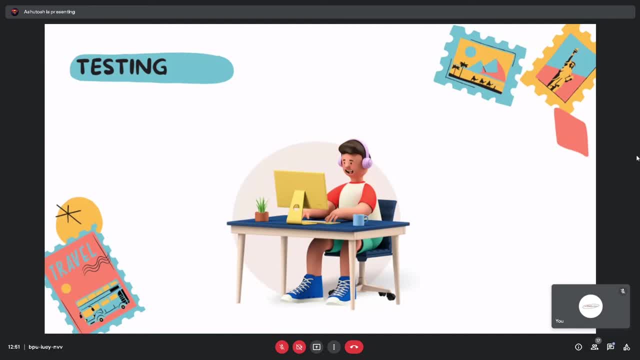 Okay, As we make food, it is absolutely perfect. We cannot say Okay. According to some test words, maybe it is not good. According to some test words, it is very awesome. And according to some test words, it is on an average. 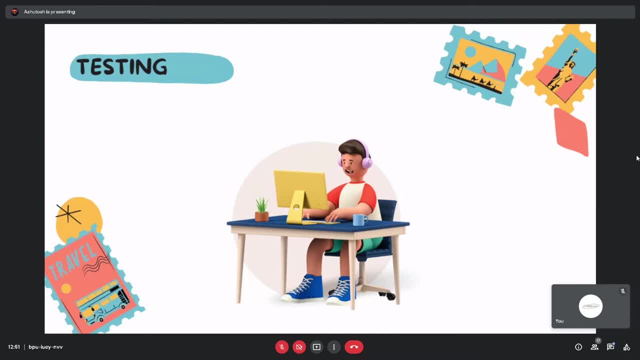 So this is done according to its scenario, But we will come back to this reality scenario, which is in IT industry. So here we can't be make anything 100% proof. It can be made, But it may like there is a probability. 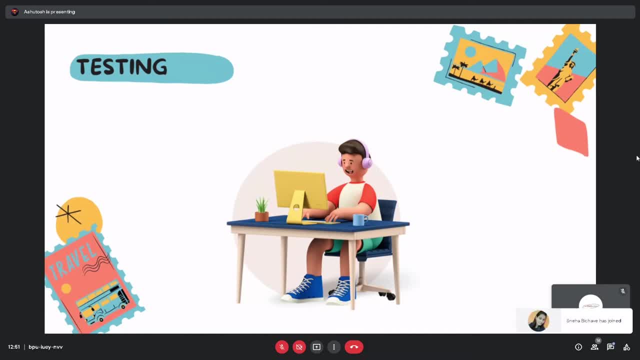 It is between 0 to 1.. The probability is always between 0 to 1.. There is no probability that it is 1%, Like how much is the probability of the sun rising. But if some cosmic effect happens tomorrow, big bang theory happens or something happens. 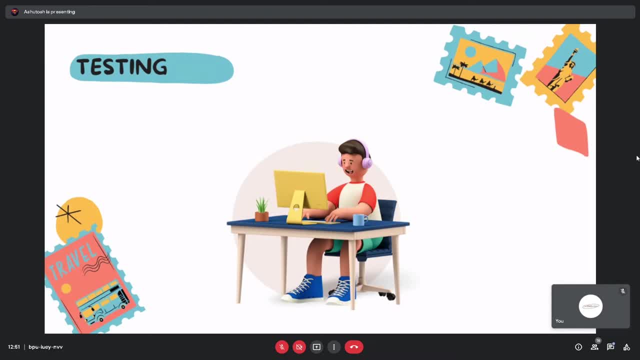 you can't predict anything. Similarly, the probability will lead to 1, like 99.99%. Similarly, testing is up to that. So in this, the QA, the quality analysis, that is done. that the way it should be designed. 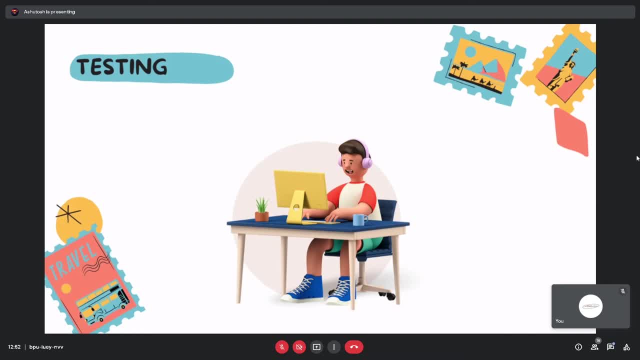 the way it is designed, or the database, its construction, the architecture is made. Has the developer followed the same thing? So, in this way, we decided in the planning that 4 testers will be used, or 2 testers will be used to test this project. 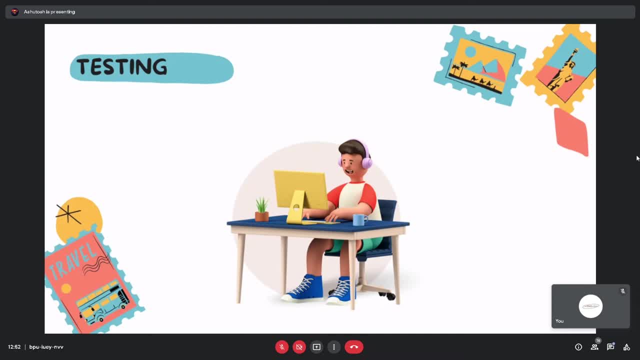 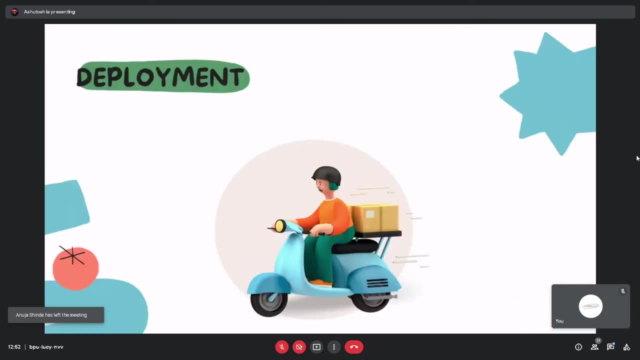 So that test is done, So that we can make a good application. After doing this testing, I would like to deploy my stage to Asutosh to deploy this project. Yeah, that is a clever use of like words. The next stage or the phase is deployment. 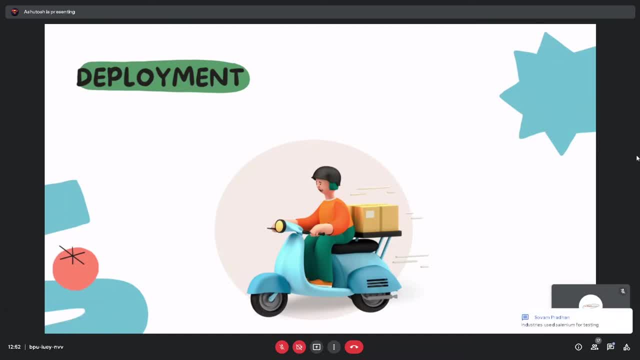 You can see this guy over here that is going to like deliver something, right? Let's suppose that is like delivering your Amazon product. okay, Asutosh. sorry to interrupt, but Sobham wants to say something. He mentioned one thing in the chat window. 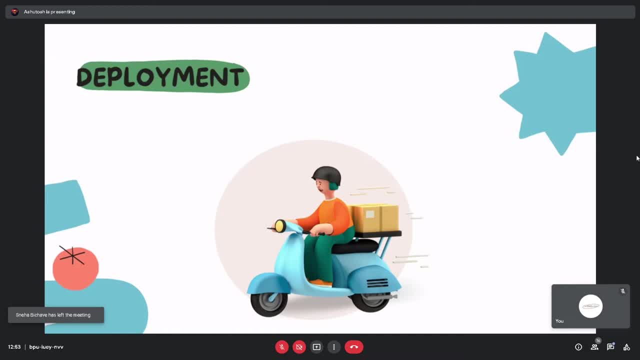 Yeah, yeah, please Can you tell me what that is? Yeah, we are sorry that we couldn't see it, But yeah, of course we will answer. Yep, you are correct, We use Selenium for testing. There are a lot of tools that are used nowadays for testing purposes. 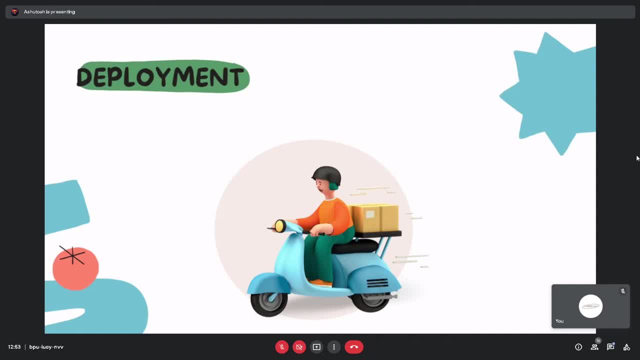 Yeah, right now I can't see that. who like wrote Selenium. Really great response, bro. Like yeah, Selenium is used for testing and it works on the Java framework, So that's really a nice addition. Thanks a lot, bro. 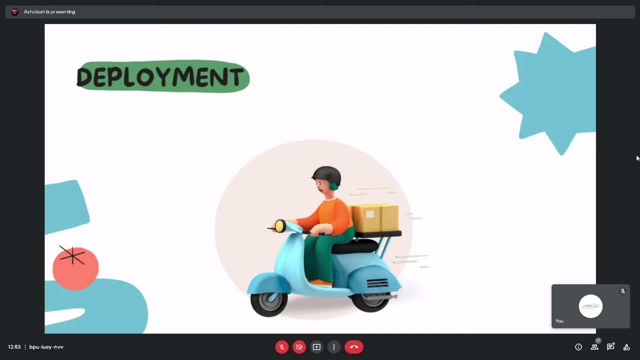 And I must say I love this active participation from all of you, All of you even who are not typing, but they are listening And that is a great thing for us And thank you for this participation. Yeah, now we can deploy our module or project. 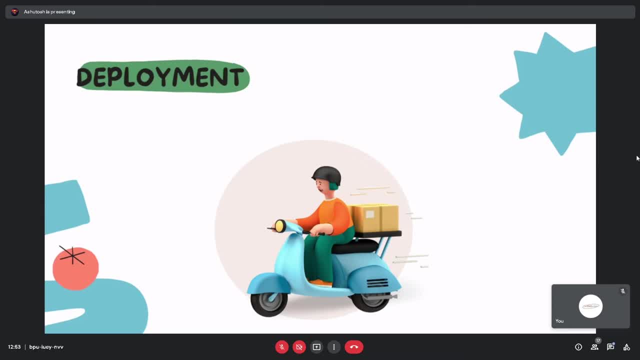 Yeah, See, let's suppose that this is our pizza delivery guy. Okay, Yeah, He's taking our product Or he's coming to us. Sorry, he's not coming. He's coming. Okay, So like he must have made like pizza, right. 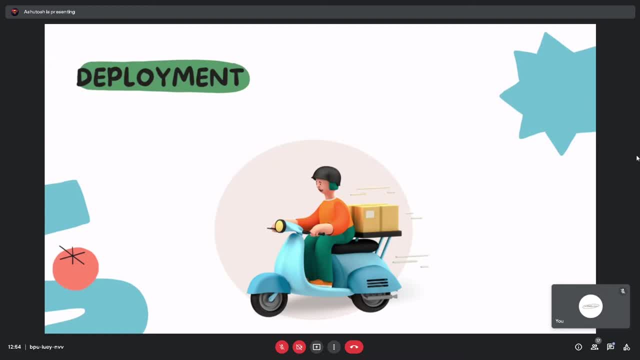 And the obvious thing is he must have tested like his test and everything all right or not, So he's going to deliver it right. Same thing is happening in the IT industry, When your client asks you to build a project right. 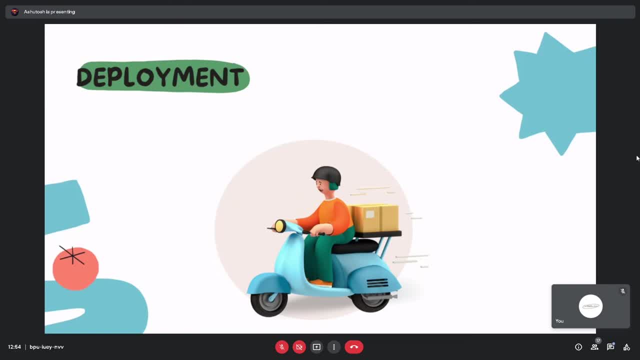 So you like: plan, analyze, design, implement. your developers have also tested it. Testers have That. yes, our project, whatever the requirement is, has been made right on it right. But when we go to deploy, this is also the responsibility of the organization that they deliver that software or project to their client right. 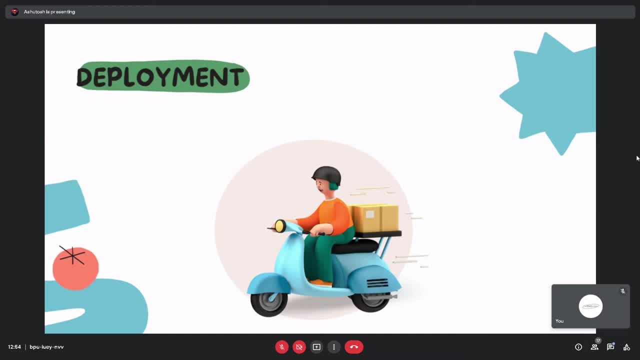 And, along with that, all the work we have done so far. okay, Where was this happening? In the environment of our organization. Okay, So when we go to give this project to our client, we go there in their environment, in our client environment. 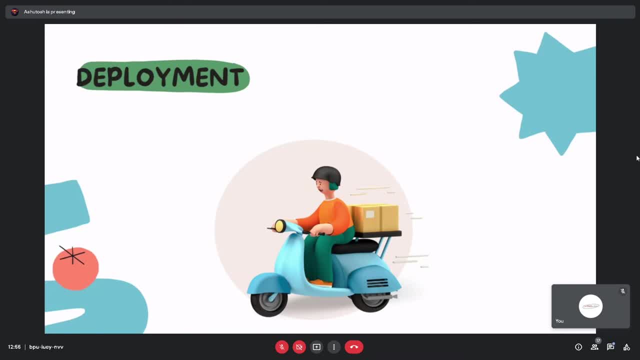 Okay, This comes under. when you will guys like to study about all these things in depth, You will study this in UAT, that is, user acceptance testing. Okay, In that there are two terms. you guys might be familiar with that term: alpha and beta testing. 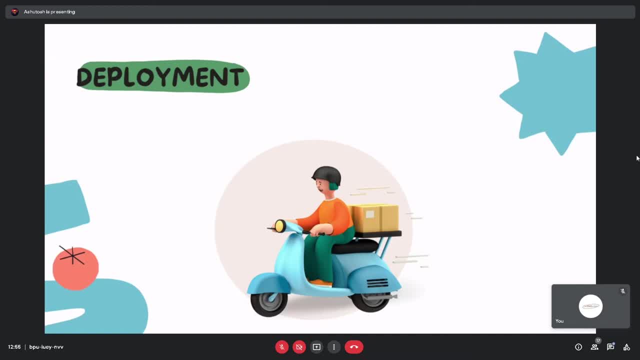 Those people who like play games. you guys might be able to understand me that. what is beta testing? Okay, I will not go that much deep right now, So let's go to beta testing. Let's go to beta testing. Okay, Let's go to beta testing. 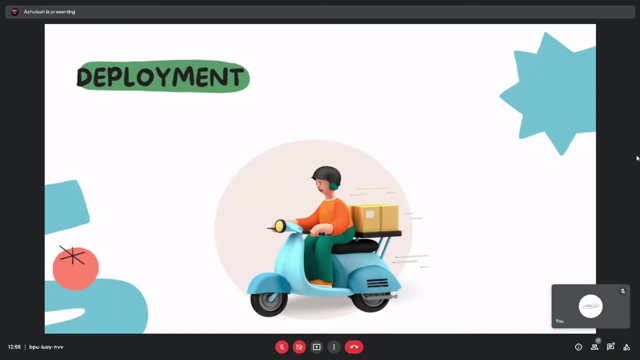 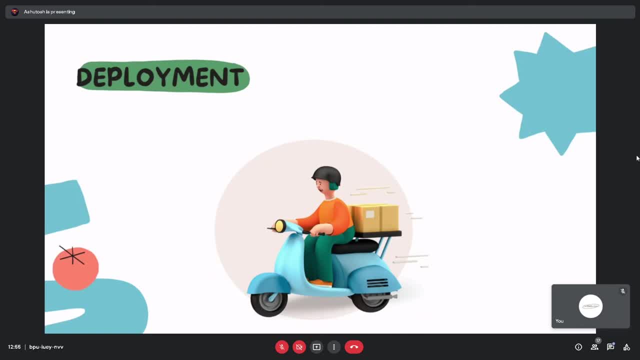 So, coming back to deployment, what is happening over here is that our product is getting deployed to the user or the client site, Okay, And also we are going to test our product, our build project, on to the user environment And if our product is working well in their environment, fulfilling all the requirements. 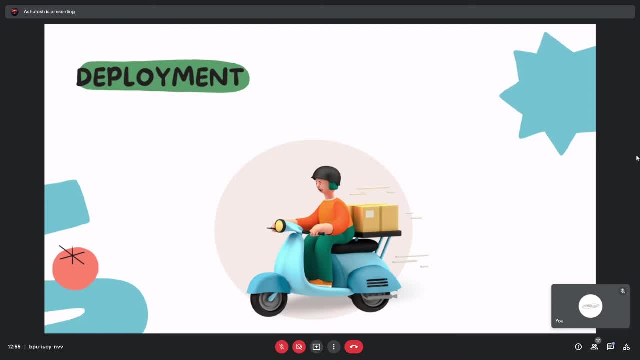 our project, our product is now made to spread in the market. So this is the thing that is happening in our deployment phase. Understood guys. Yeah, one more point I want to mention: Ashutosh ji. It will be helpful if you mention the deployment server names, like where we can deploy the things and all. 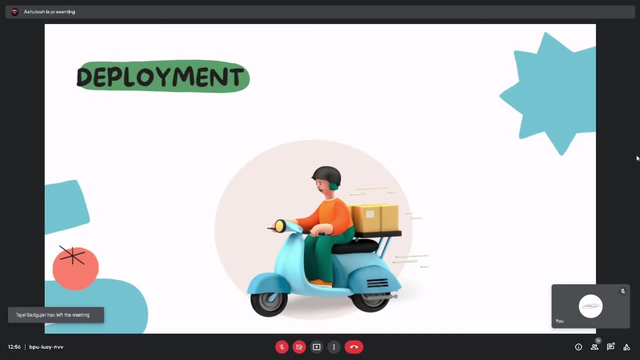 It will be helpful for understanding the things, As first I thought about that not going that much deep, But if it is a request from you guys, then of course we can go into that much depth. Wait a second. Yeah, So we can deploy our product into the like the databases of our user or the client that have requested our like the project to be built. 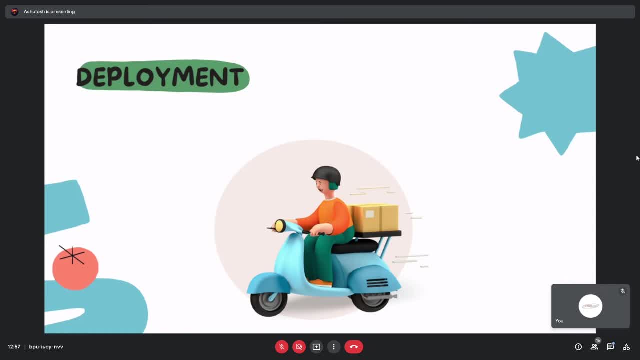 So this is the thing that we do into the deployment stage. Does this answer your question, Premraj? I think you are Premraj, right, I can- like I remember you- Yeah, Ashutosh, Yeah. And Sobham also gives the answer- like we can use the cloud platforms for deployment, like AWS, Azure. 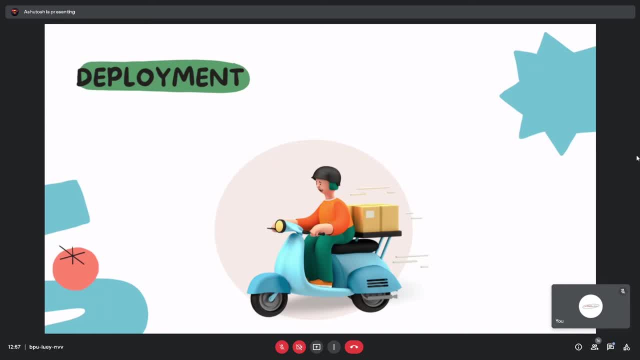 G Suite Like Google, Yeah, yeah, I only told you about the databases that are right now My bad guys Like. yeah, of course, if the like, as the technology is progressing day to day, According to now, all our projects come, all the client requirements come. 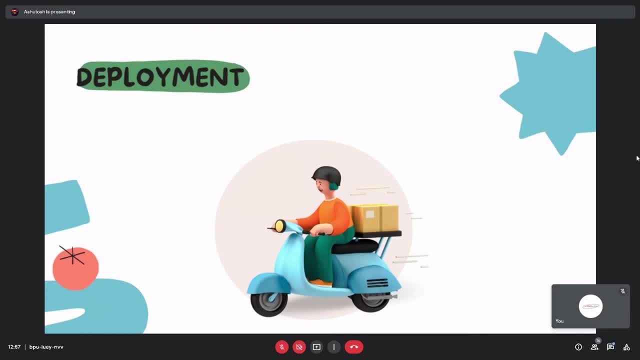 They want all their projects to be stored on cloud services, Because it also has a lot of benefits. Like that was our previous methodology. Like previously, when we used to backup data or upload it, we used to use rare technology. We used to do that. 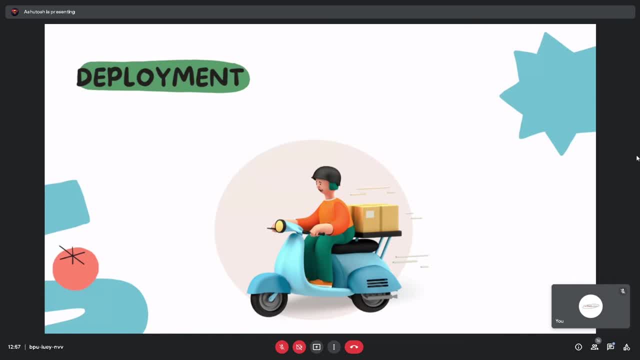 Rare. You guys might understand Leave that part. Right now we do all those things in our cloud services- AWS and all those things. So thanks for that input, bro. Who were told about the cloud part? Really Thanks a lot bro. 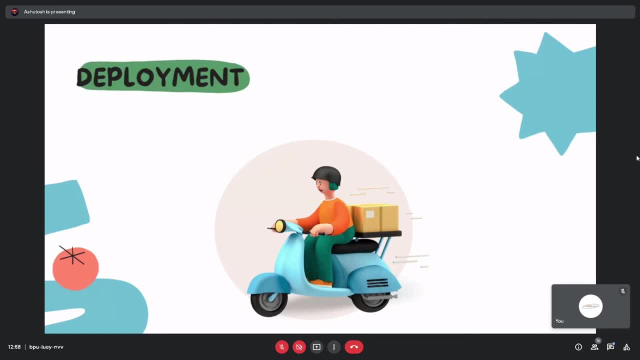 Moving forward after deployment. See, as of now, we we have like sorry, we have deployed our project into the like user environment. And now what if? Okay, What if it happened that, like, we delivered things to our client and they like in between? 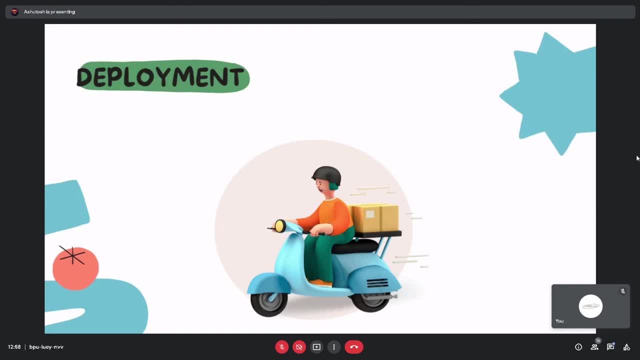 like they thought that this feature should be added extra to it. Okay, Or there was a bug or there was a glitch, that they have to quickly maintain those things Like fix those defects or bugs. So what will happen? Right, So for that we come to the next phase of SGLC, which is maintenance. 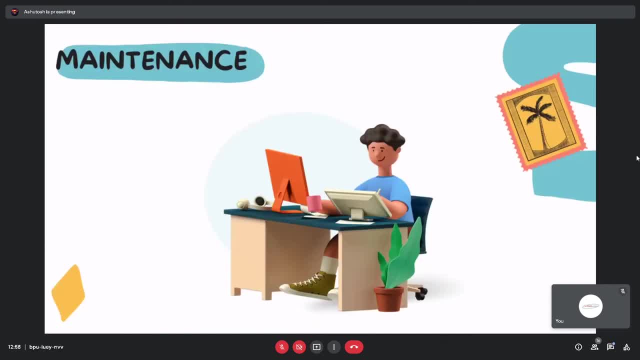 In maintenance We ensure that in the future, in our project, in our product, in our software, whatever bugs will come, whatever defect will come, we will detect all those things properly and remove them. Okay, In the maintenance phase we have to do extra addition, which is an upgrade. 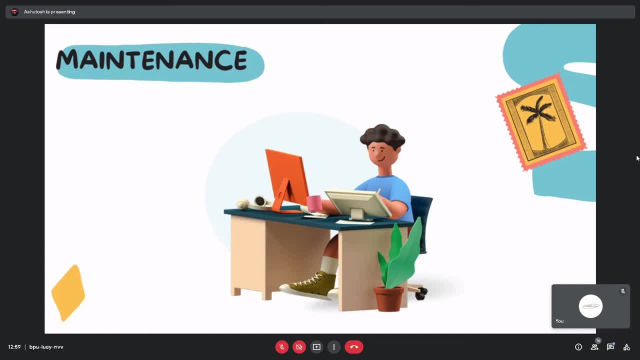 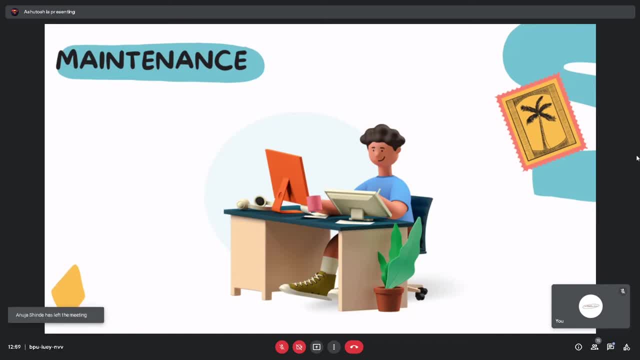 If you have a software then you must have seen that many times the updates of each software keep coming Right. So what happens in those updates? Those updates are the previous bugs that mean that the encounter had happened. that the user said, or even they, like their backend team saw like. 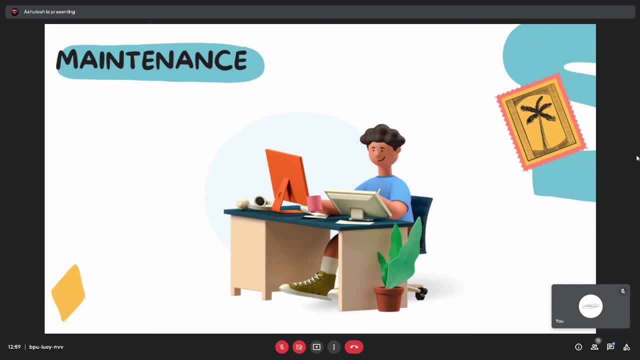 They fixed that bug Right. So the maintenance phase that is there is for indefinite period, As long as our project, our software, is in the market. the maintenance phase is going on Right, Because the bugs that can come in the future, right. 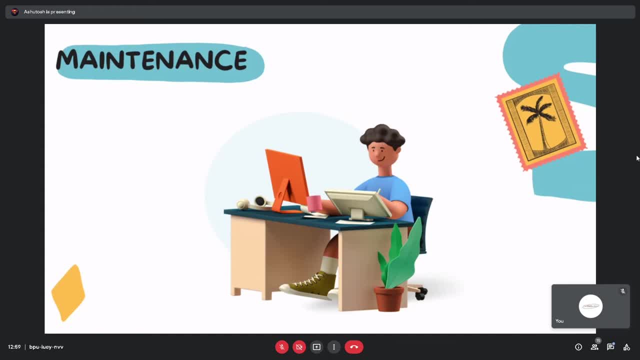 So we are happy with that. So in the maintenance phase we have to fix that Right, Right, Okay. So we always have to maintain those things, that new bugs will keep coming Along with that. if we take an example of a game, then there are many such features that are added to the game later. 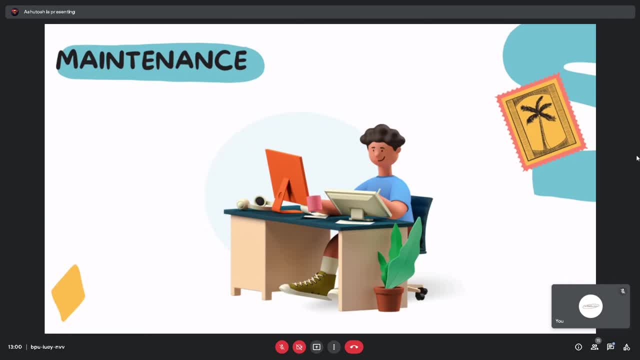 Or there is a software in which there is also a feature. for example, there is a software in which we have a feature to call. In the future, we want to have a video calling feature in it. So this will be an upgrade right. This is not a bug, it is a simple enhancement right. 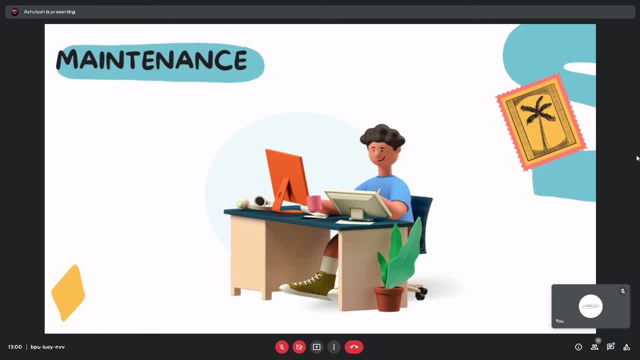 This is an upgrade, so we include these things in maintenance. That is, in maintenance we include bug fixing, upgrades, enhancements, all these things. Okay, guys, so these are all the steps that all the phases that we do in our SDLC. 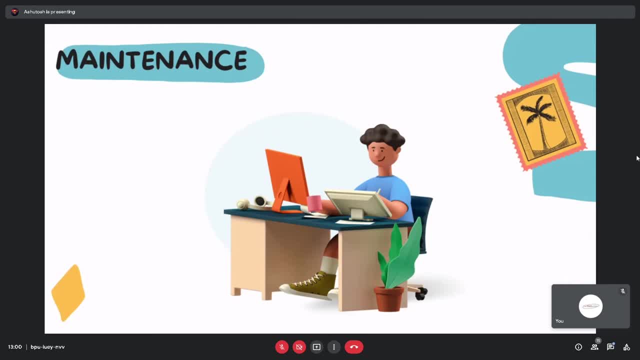 Okay, guys, Is it clear till now that this is the final phase of SDLC? So can you guys see, Please, please, please respond that. Did you guys understood what are the stages and what are the phases of SDLC? Okay, till everyone responds, whether they understood or not. 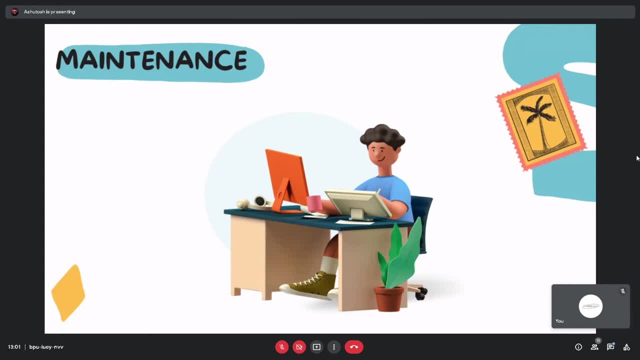 So everyone thought that there are some tools for testing- correct- And there are some places for deployment where we can deploy. So did anyone think that when we do planning or whatever we decide, will there be a place for it Where we can write it down? 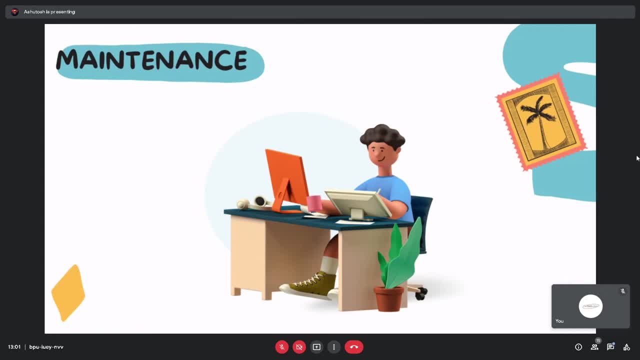 Is it not like that? we have written in the notepad that today we have to do these things. that's it. Did anyone ask that thing? Is there any tool for planning, Where we can write, where we can maintain the record? We use Trello. 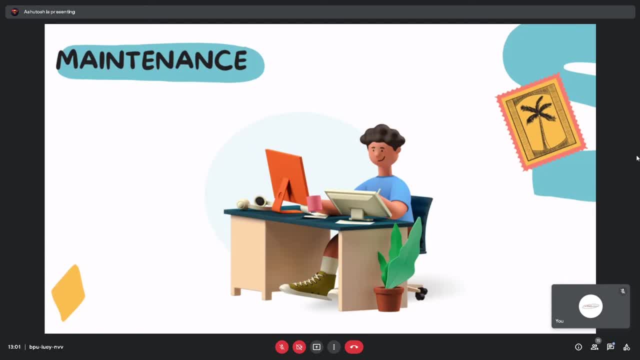 Awesome response, And anyone else And anyone who is using right now or who knows something Input want to give. I use Trello. I use it. I think it is better. It works perfectly. Actually, what happens in it is that the whole team can work in it. 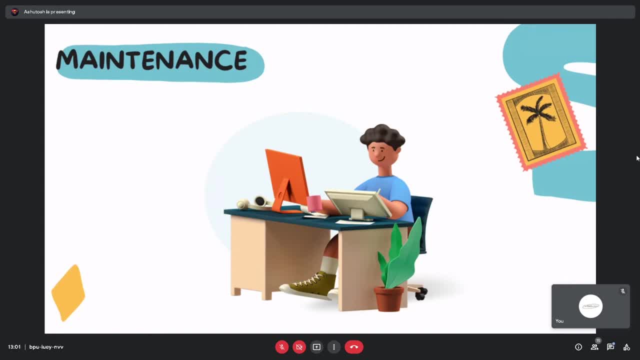 If we can give access to the whole team in it, then it becomes clear what is the overflow of the project. So it is better understood from there. And if you can make three boards there: what we thought, what is in the planning phase, what is in progress and what is completed. 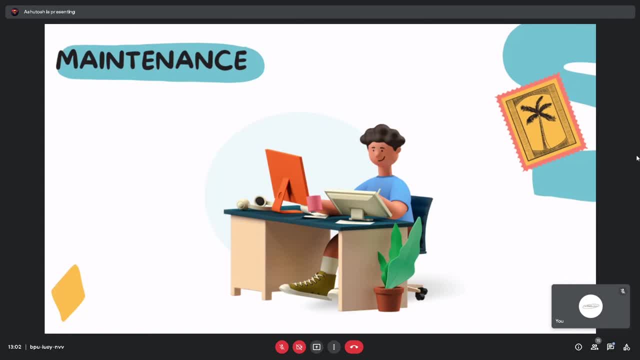 then it is better understood that, yes, this is happening, so much progress has been made. Yes, And normally the company's industry strategy is that the agile is coming, but they make their own ticketing system, Because if you are in the industry, then ticketing is the form of issues by the clients. 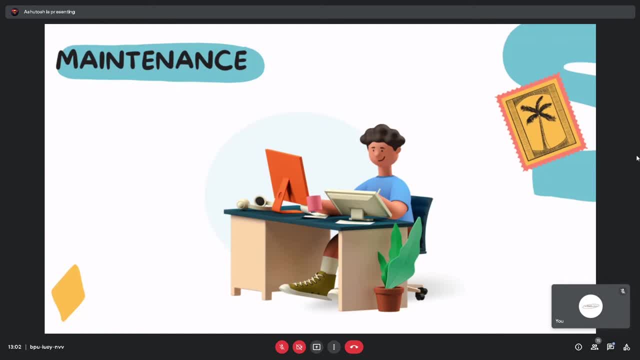 Correct. Normally they use the ticketing system to apply for that particular system. Correct, This is too much, this is not enough. No, no, that is really valuable information, bro, Because in Trello our collaborative team effort is a must. 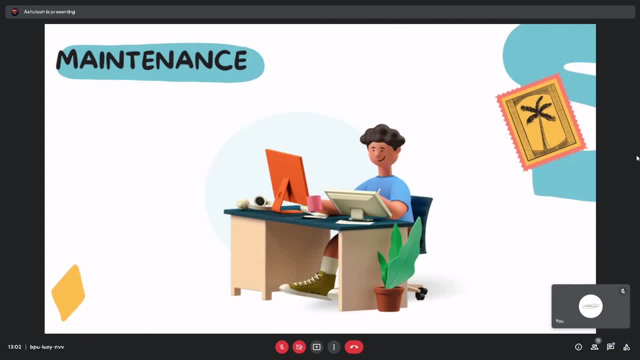 So don't worry about all the things. All the things that you are telling is absolutely correct, bro. We really appreciate it, bro. Yes, So, as we said earlier, we use some such applications Similarly, right now, if we. 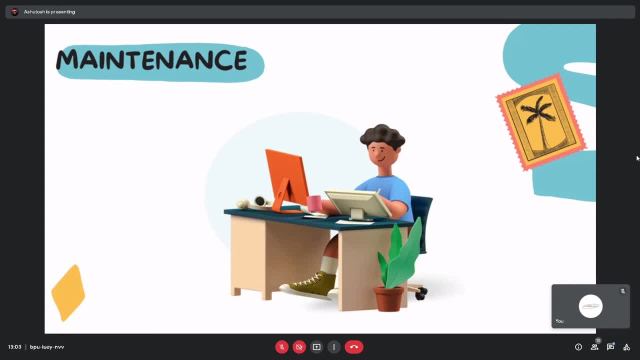 Q-test, Q-test Okay, Especially if I speak from the point of view of the tester. then all the evidences that are taken are uploaded in the Q-test where anyone or when UAT is performed, as Ashutosh said. 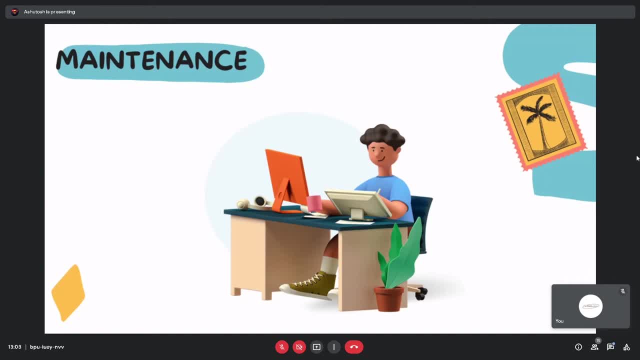 or anyone has to see whether it is rightly tested or not, Because even if you close your eyes, you cannot trust that this is tested correctly. So some evidences that are proof: as per requirement, as per software design document, these things have been implemented. 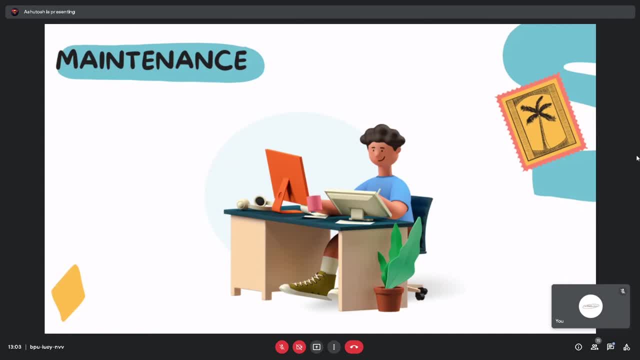 Test evidences are uploaded there. And, Jira, These are small components that you can divide into sets. This is a bigger set. Suppose there is a bigger project you want to develop, you can divide that bigger project into smaller part. That smaller part is called as. 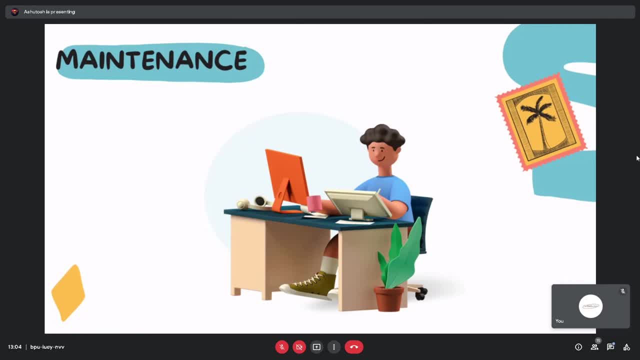 Story. In that story you must give the description. Like software design document, you must give the description And this is not the duration of planning After budgeting and all that stuff. it happens Where you write what we needed And it is also written for the tester what you need to test. basically, 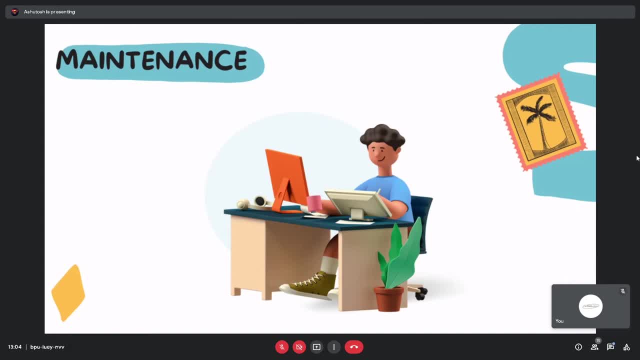 Okay, That happens in Jira Right now, which we are using. Okay, So for planning, you got to know what you can use for testing and deployment. Still, if anybody has doubt, they can ask. If not, we will move on. 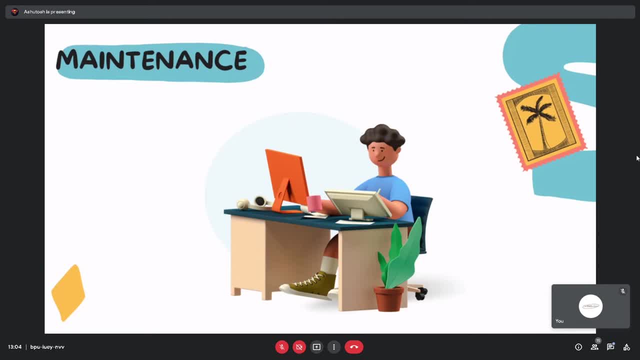 Tick, tick, tick, tick, tick. You have to be faster. Type yes or no. And thank you, Soham, for participating. I must say you are a great guy And we are having very beautiful future, Like Pragya. sorry for interrupting. 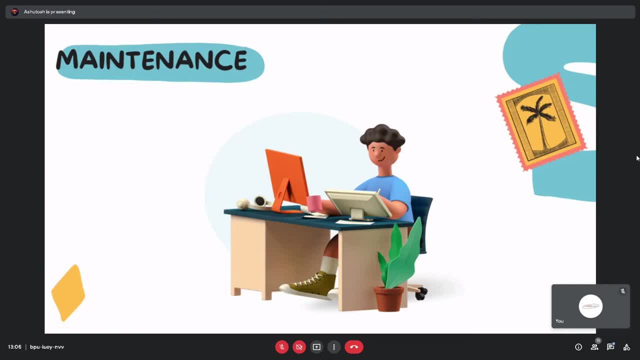 but I am curious about Soham's background. Soham, can you please give your little bit introduction? Yes, Soham, I am Pradhan. Actually, I am not working in industry, But I have intensive experience. That's why the industry is how we are using it. 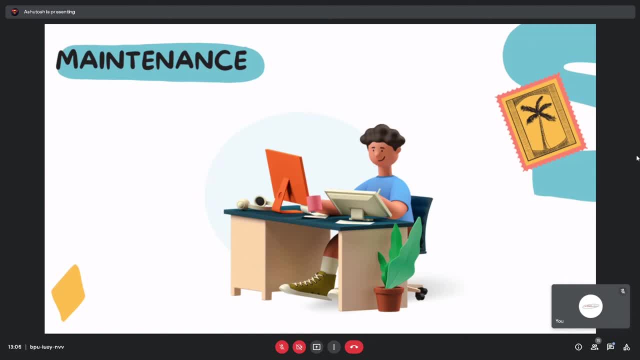 Actually I am in fourth year, And this is my fourth year, So I am placed in three companies. So it is starting our next year. So then we can start my corporate life, But till now I am doing internship in three companies. 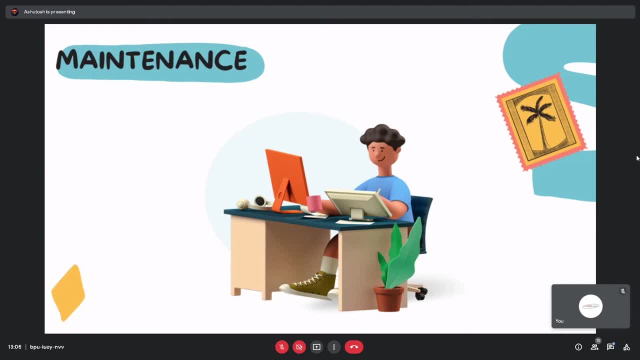 So, whatever process is there- that's why I am selecting these things or not. Really great, bro, And all the best for your corporate life. Thanks a lot And enjoy that life. Thanks Yeah, man, Definitely means you will. 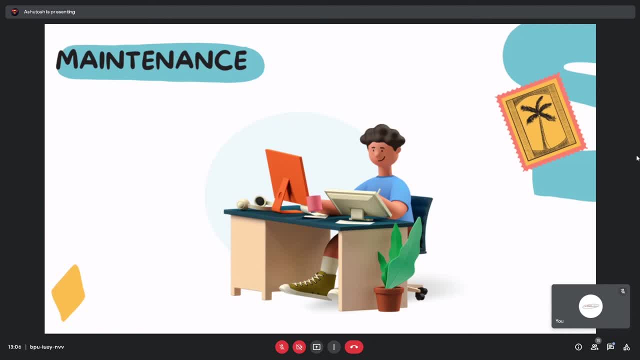 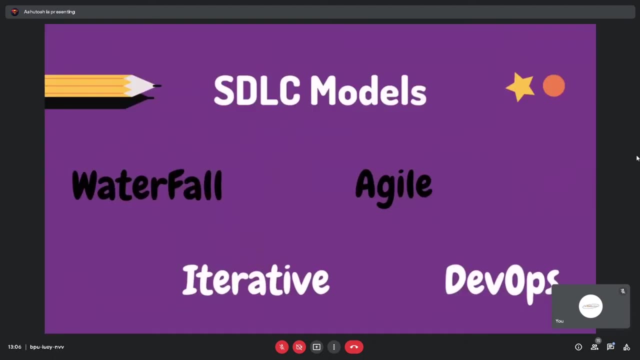 You have explored much more things before going in corporate industry, bro, So keep it up And all the best. So, without wasting much time, we should move on. Modules used in. I think, Pragya, your voice is breaking. 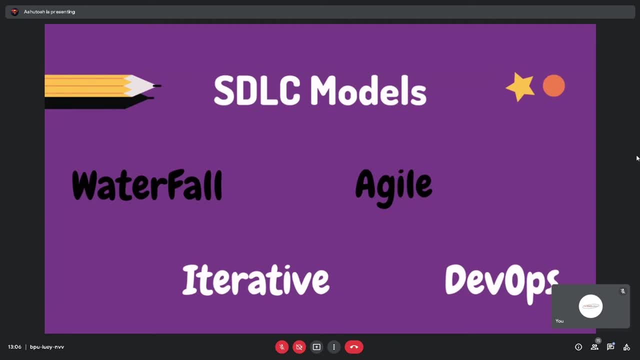 Just give me one minute. Yeah, it is fine now, Okay, Am I audible now? Yeah, yeah, Yeah, you are audible. Okay, Just give me one minute, Or you can give only five seconds. Just count one, two, three, four, five. 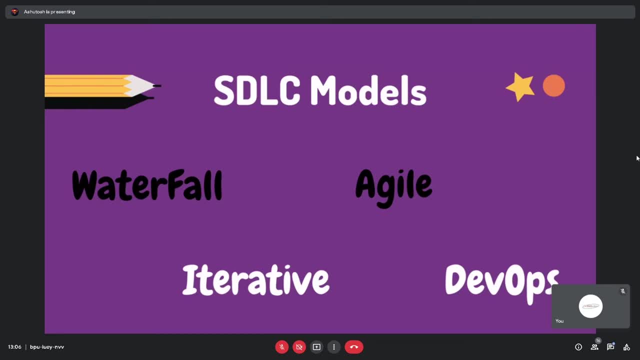 Okay, Till that, I want to mention that those who haven't filled up the attendance form yet, please do so so that we will reach out to you and we will And we will give some. So please feel free to fill that form. 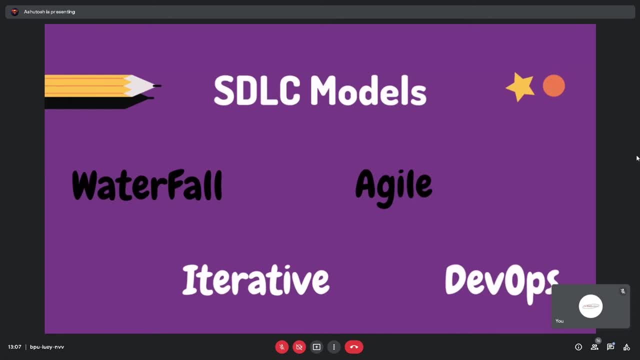 And, don't worry, we will not forward any few details to anyone. Okay, now it's good. Yeah, it's good. Okay, thank you, So, yeah, So there are four. Basically, we here represent only four models. 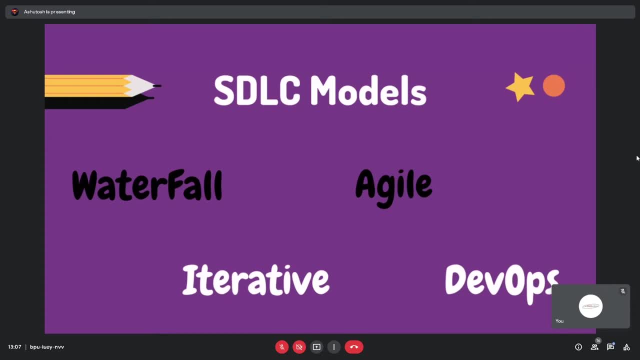 And there are so many other models also, As Soham earlier says, a lot about Agile, Agile, Agile. And who haven't heard about this Agile methodology? you will gonna know about this Because in this session, we are basically focused on Agile methodology. 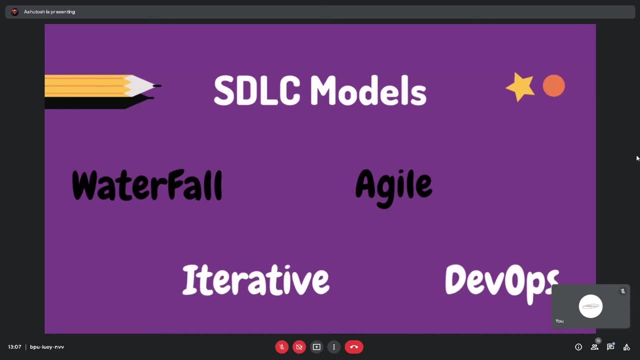 Because right now, this is a leading model which is used in SDLC as an SDLC model And this bigger organization Okay. So yeah, Ashutosh, you want to say about waterfall, iterative and some You can brief it out- some of this model. 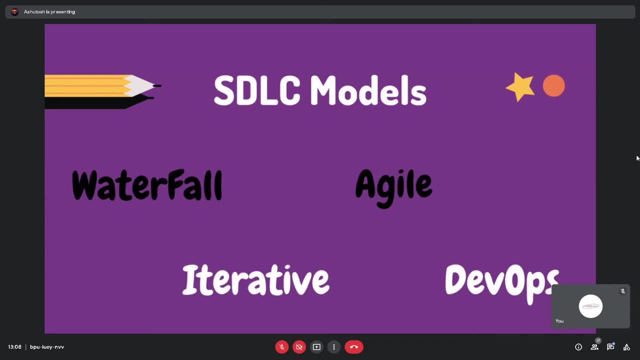 Yeah, So, guys, And also I want to say that you must, If you remember about NASA thing, you can please give that beautiful idea to our audience. Yeah, sure, You guys must be curious about what I said about NASA. 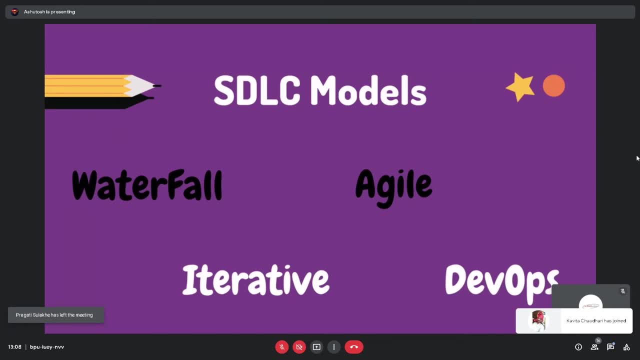 Right. So the thing about NASA was that when NASA was working on its Mercury mission, when they were working on this mission, when they were sending their orbital spacecraft to Mercury, when they were working on that mission- this is a long time ago. 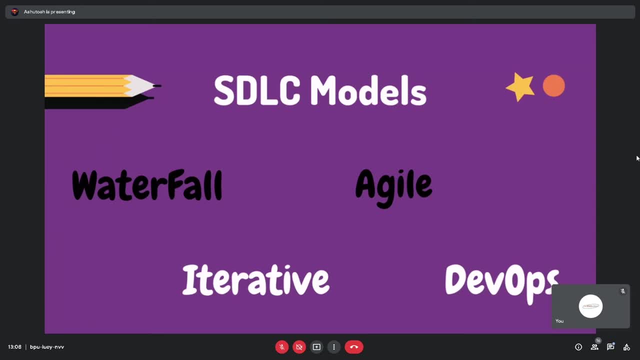 Okay, So in that time in the organization these were all models. At that time Agile DevOps models were not there. Okay, So when NASA team was working on this project that they were sending their mission to Mercury- 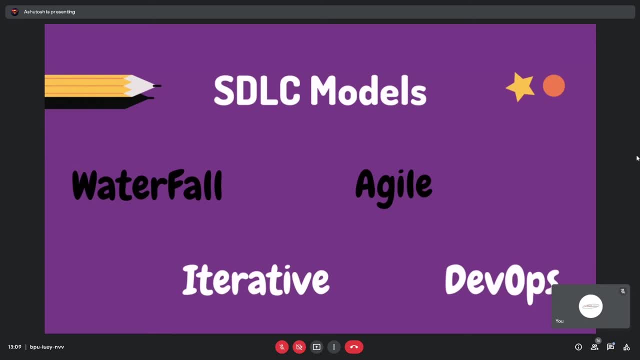 then what happened was that? like, of course, like it is a dynamic thing, Like the environment of Mercury, not environment. the atmosphere is dynamic, Right, It is not like our Earth's environment. So what happened was that? when they had to plan out their mission. then the requirements suddenly changed. Okay, Like they would have required a heavy vehicle first. Why? Because, obviously, Mercury's gravitational attraction is less than Earth due to the smaller size. Okay, So all these requirements. 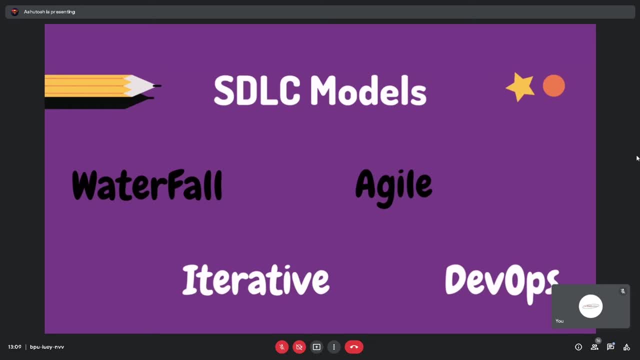 this is a simple example of requirement. so their requirements, like in between the project, have changed. So at that time, NASA team developed a new methodology model, which we call iterative model. Okay, They like divided their work into small pieces. 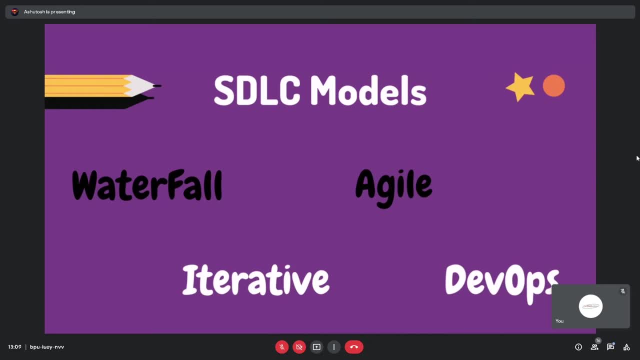 and divided that work into different teams so that each team could complete their part of the work perfectly and efficiently. Okay, So these are the things. these are the small, like incidents of human nature, due to which, slowly, many models came along. 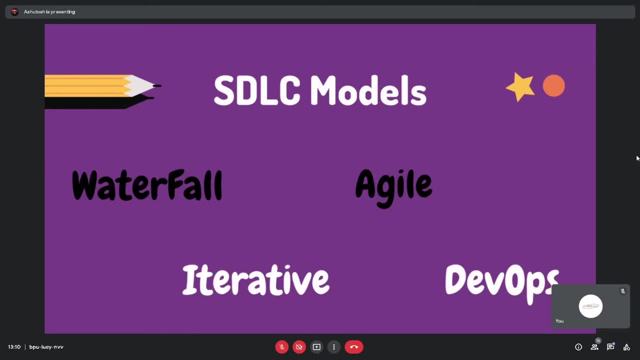 As of now on the screen, you guys are seeing that there are waterfall, iterative, agile and devof models. There are other models, so there is one model named Big Bang model and it is one of my favorite model, So I will not go that deep. 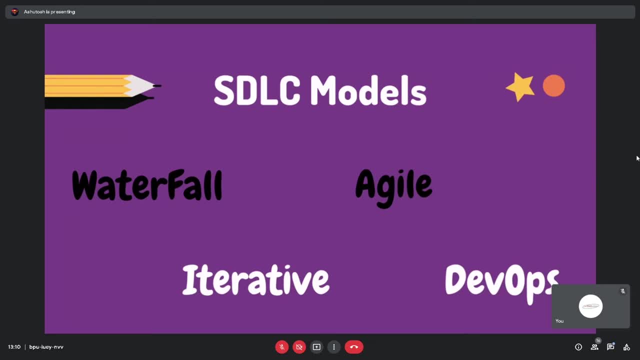 So, without wasting any further time, let us go deep into the agile methodology. Okay, So you guys ready? No, So before we start, we haven't studied so much yet. We just have to ask one question, That is. 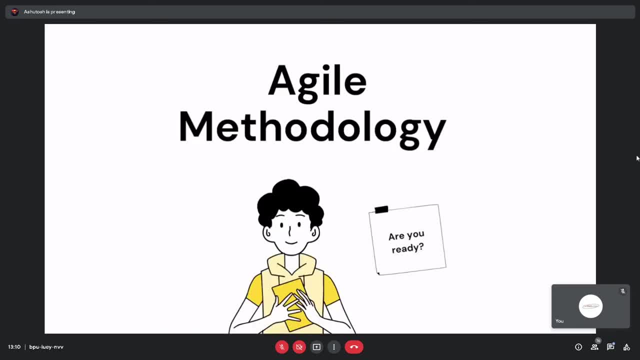 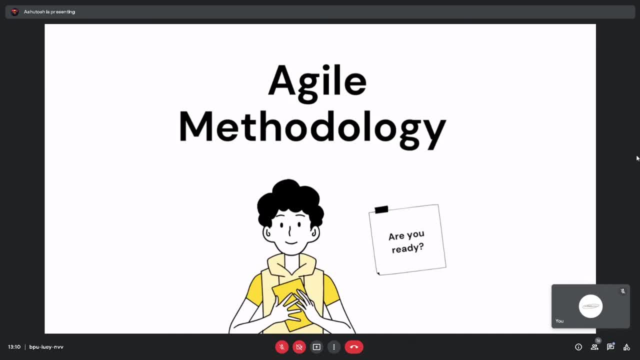 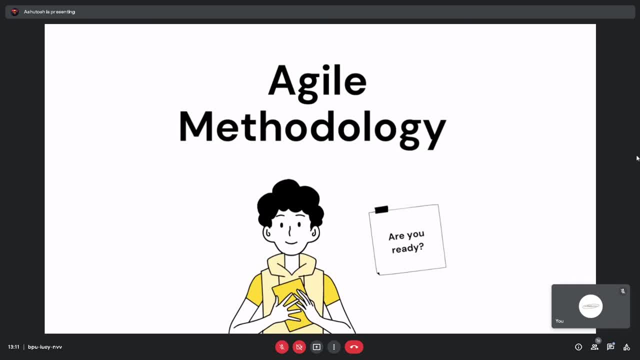 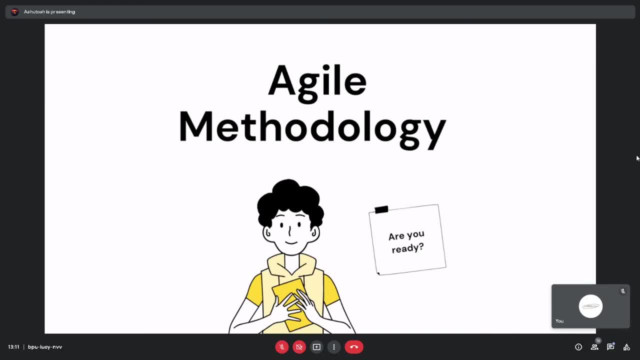 in your life. So what is the most important thing in your life? So how many phases? I'm not asking what are the phases? how many phases unmute and say four, five, six. at least you can do this thing, okay, anybody else want to? 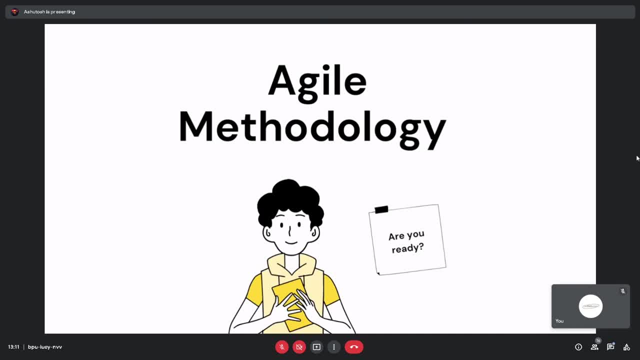 answer. Thank You, Ananya. I think her name is Naina. yeah, thank you for correcting frame. yes, ma'am, yeah, yeah, I'm really sorry, sorry, okay. yeah, shri tapas, are you there, tapas? yes, I'm here. yeah, total in SDLC. that was fine, I don't need to hear your voice. 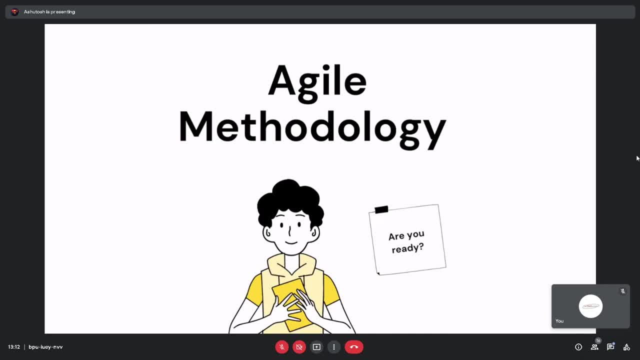 yes, this is wrong. if you guys don't respond, then I won't be able to fall asleep. okay, say it again. I can't get it right. no, I can't get it right. Abhinash, you are from the starting. please give an answer. 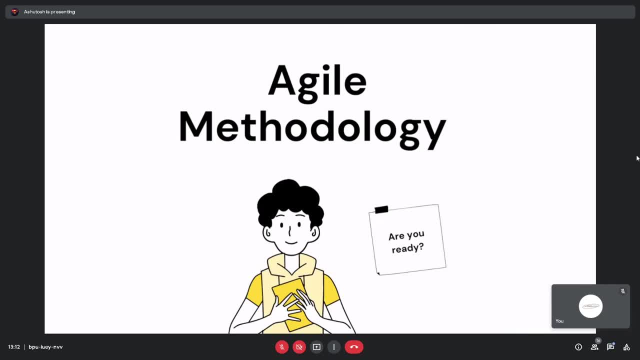 Okay, Mithlesh. thank you for the response. Kavita, You want to add any point, Like: how many are there Phases? Okay, we got as many answers as we can. Thank you for responding Okay. yeah, we can move on with the agile methodology. 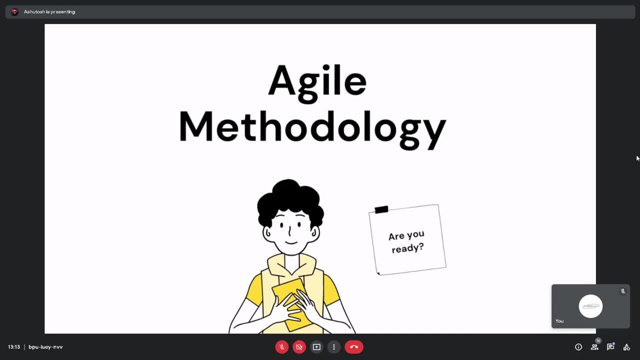 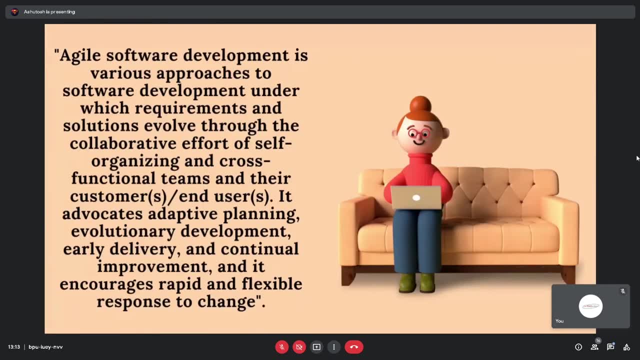 So, guys, Yep, yep, continue, Yeah, agile methodology- okay, So let me like first read this out: Agile software development is various approaches to software development under which requirements and solutions evolve through the collaborative effort of self-organizing and cross-functional teams. 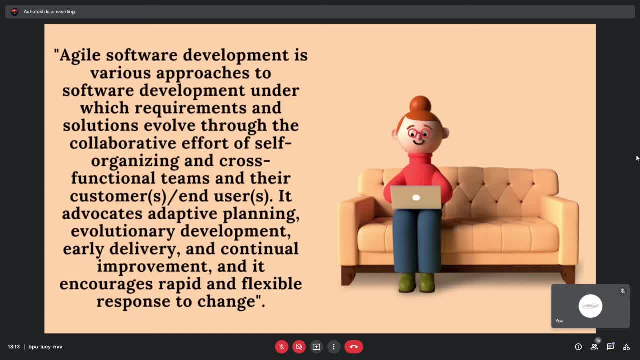 Okay. What happens in agile software development is that the software we are going to develop? okay. In any organization that is going to develop software, there should be the participation of the whole team. It should not be like someone is working and someone is not working. 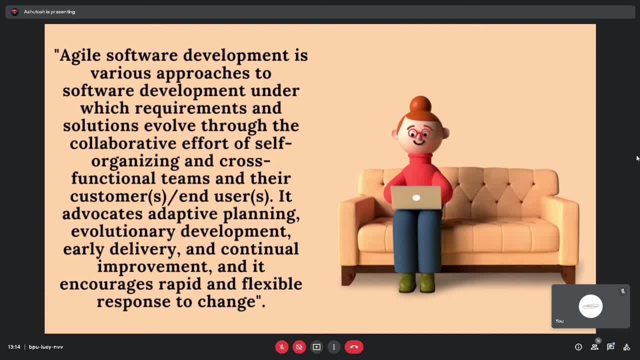 This type of work should not be done. All teams should have equal participation and necessary participation. Okay, All of them should be putting effort into one valuable thing, Okay, And cross-functional teams and their customers and users. It advocates adaptive planning, evolutionary development, early delivery and continual improvement. 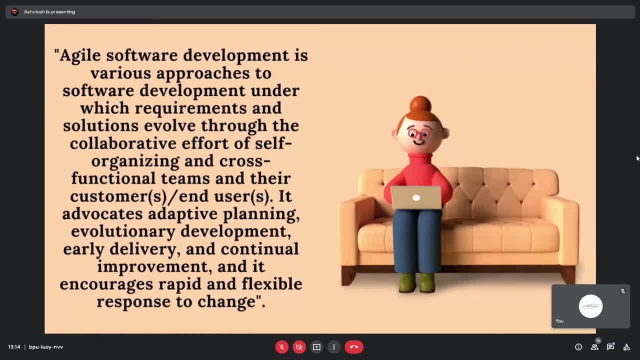 And it encourages rapid and flexible response to change Like. let me explain all these things. It advocates adaptive planning. What does this mean? This means that, like in agile methodology, we ensure that when we are building a project- okay, The project we are working on. 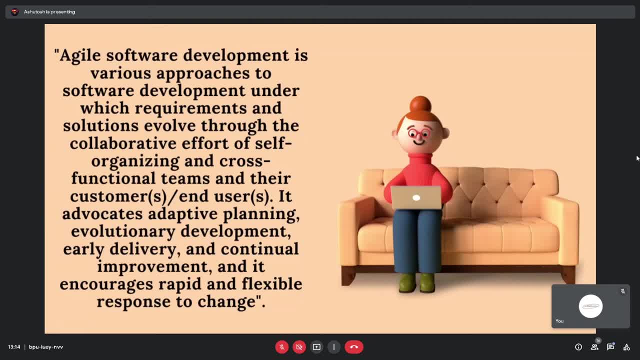 Like, the client told us that suddenly in between, this is an extra feature that we have to add, Or this is the feature that we have to remove, Or this is a feature that you have added, but we have to make these changes in it. 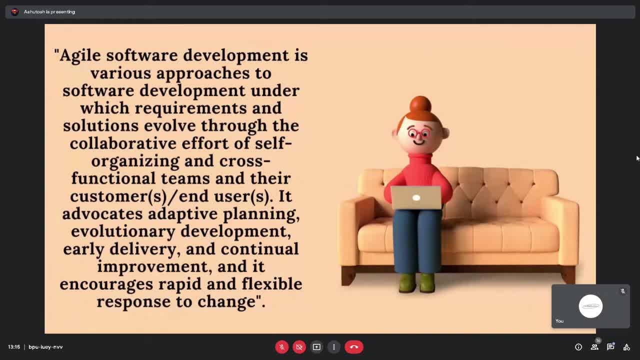 Okay, The organization that follows the agile methodology should always be ready for this. It should be fully flexible, that whatever changes come in between projects, okay, It can work directly on it at the same time. Not that we put it in the backlog that we will do it again someday. 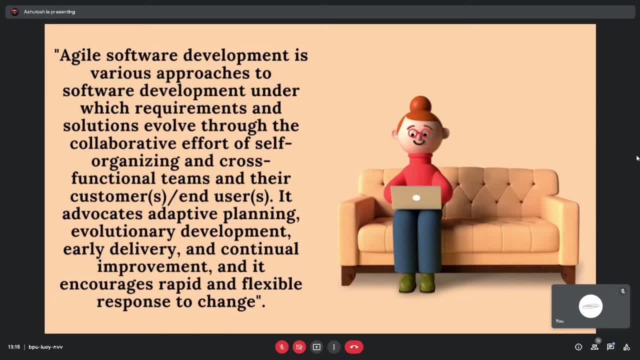 Okay, Whatever changes come like, at least the team should be responsive that whatever changes come in between our project development can work on it. Okay, The next step is evolutionary Adaptive planning, Evolutionary development, Early delivery. Early delivery ensures that our client, our stakeholders, have asked us to deliver the project, to build it. 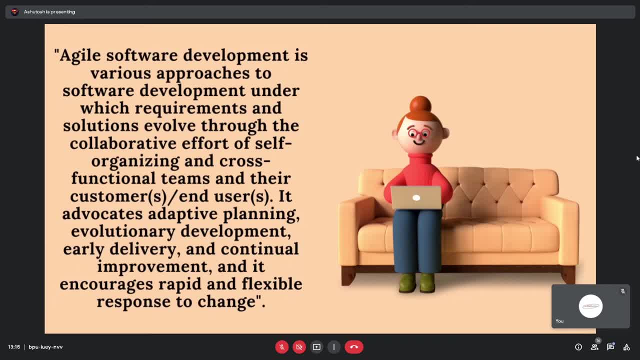 So we will want it to come to us in the future too. Like any organization, any other organization has asked us to develop a product- Okay. So obviously the organization that is developing that project will want that next time that company will bring its own project to us again. 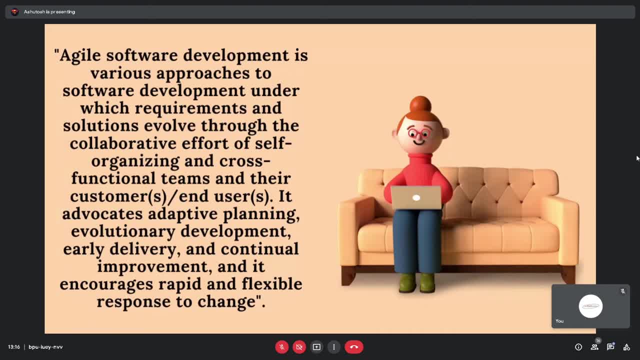 Right. So to ensure this, we have to do it. Okay, So we have to do it very well. Any organization has to build the product well, have to deliver it in time And we have to ensure that we deliver it a little earlier than the time. 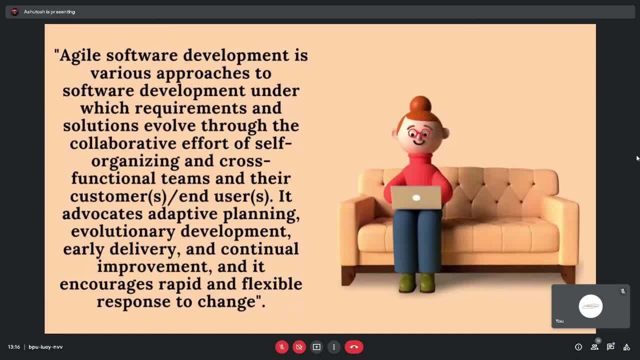 So that we have extra time to discuss some unplanned things or pay a little attention to it. Okay. Moreover, sorry guys, In agile methodology, what else do we ensure That whenever there is a meeting, okay- And that meeting should be between the team or the client- with anyone. 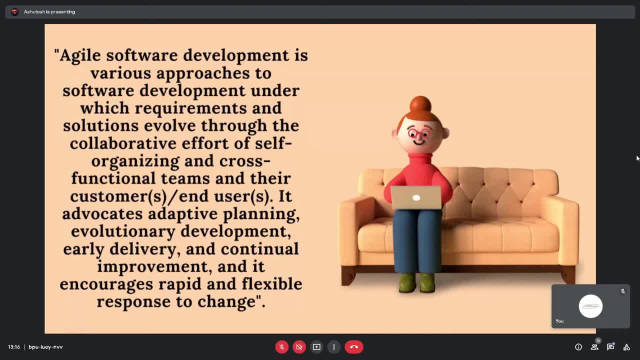 So there should be an interaction of everyone. It should not be like two or three people are speaking and the rest of the people are sitting quietly. This should never happen in agile methodology. Every individual should have proper communication and proper interaction. Okay. 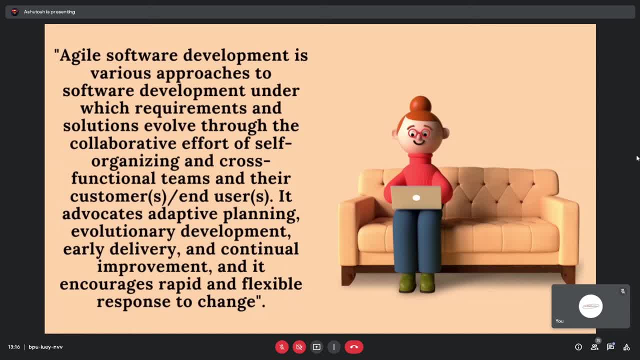 Then what else do we ensure in agile methodology? That whenever we like a client like this- Like- sorry to say, I don't remember the name, But you had said that we prepare checkpoints, Right. So this checkpoint in agile methodology works in such a way that when our in-between product development, when there is interaction with our client, 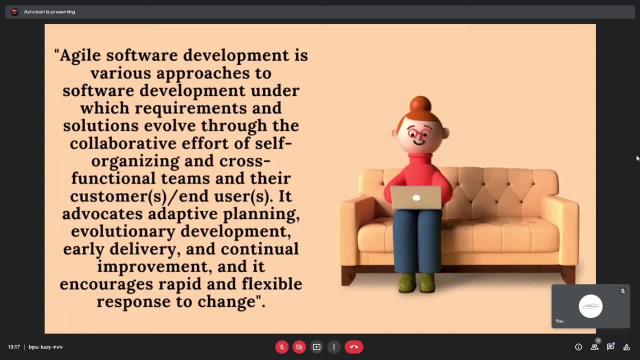 Okay, So you yourself think that you let someone work And when you are planning or meeting with him, in between, he showed you documents and in-paper that, yes, this work is done And there is another person. like there is another organization. 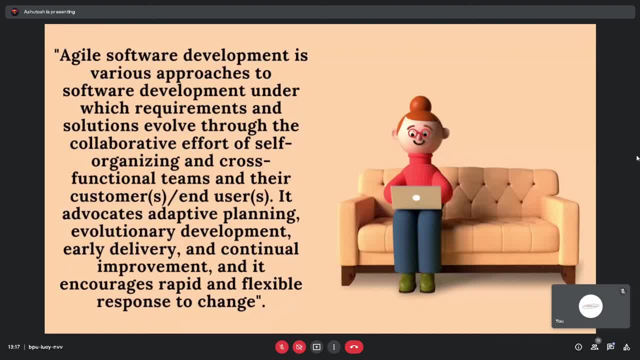 He is showing you that straight software is showing that, yes, you had asked for this requirement. We have added this requirement till now. Okay, So which one will you like more? That organization which is showing you in the paper that this work has been done till now. 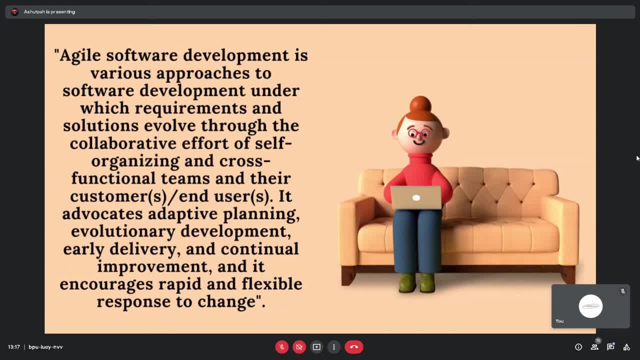 Or that organization which is showing you straight in the software that this work has been done, Like. it is like pretty obvious that everyone will like that which is showing directly on our working software that what work has been done. Okay, So this is the main motto of agile methodology: that we work on working software. 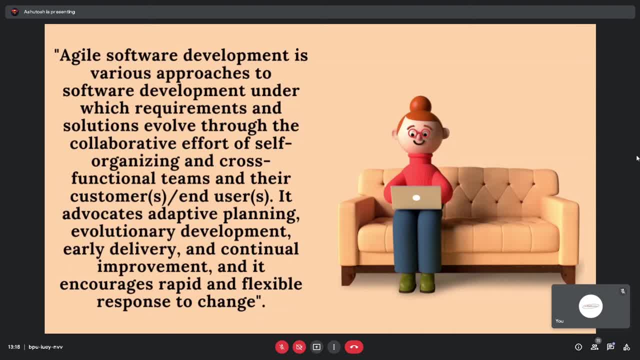 Okay, Documents will be made later. Okay, But first working software should be ready, Okay And flexible and respond to changes. I have already said this, That in-between, whenever there is a requirement, change, Okay, Always, we, our agile team, will have to be ready that it will evolve on rapid changes. 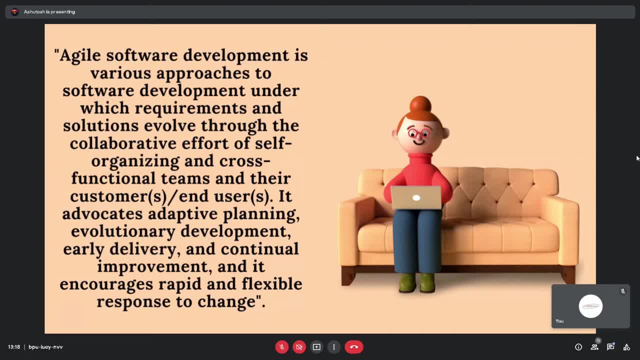 So we can easily focus on these changes. Okay, Ashtosh, Yeah, So we just came to know that what is agile developed model? Correct, So the agile model is SOVA, So you can tell which one, basically, which one, which methodology is there in it? 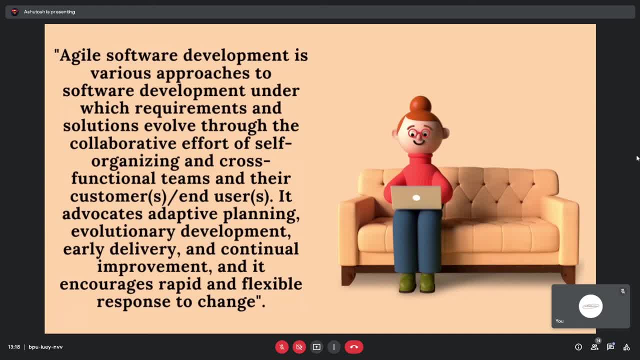 Or you can say what framework is used nowadays. Okay, Scrum is there, isn't it? Yes, Scrum is there. Some people say that Scrum is Agile, Agile is Scrum, But it is not like that. Scrum is a part of Agile. 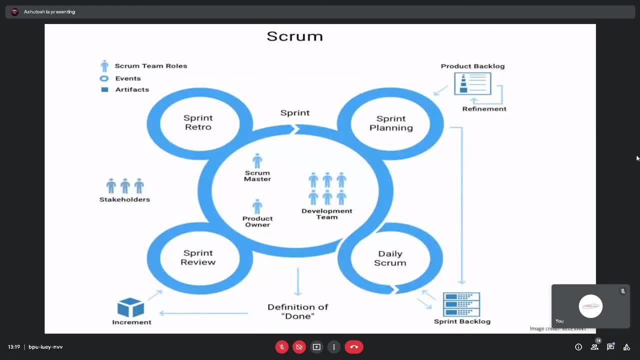 Okay, And in Agile there are many other frameworks which are used, like Cannabina, Extreme Programming and all the other frameworks, But basically the most popular one is Scrum. Okay, So now we will not read about them. We will read about Scrum, which is being used more in today's days in industry. 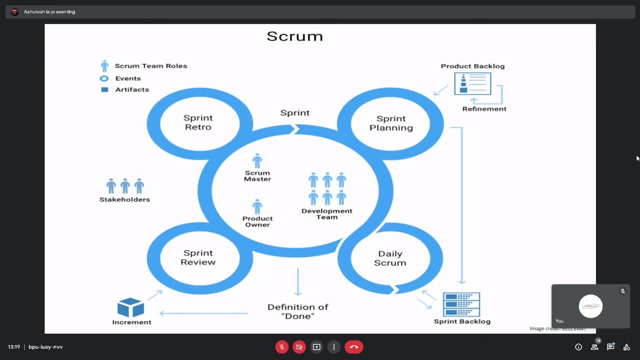 Okay, So you can see the diagram here. Some Scrum masters, Product Owner, Development team and Tester team should also be there, But this picture we want to credit RedLivent. We have taken this picture from there, So just to describe you all guys. 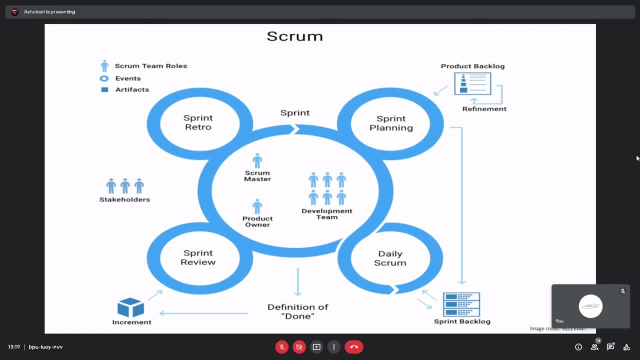 Okay, So, as we had told something earlier, So those who did not know, So those who have no idea, they will understand, of course, after this. Okay, So, in Sprint, let us suppose we take an example, that we want to develop the home page of Zomato. 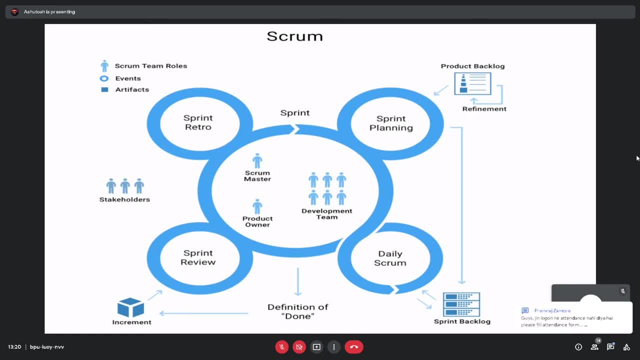 Okay, I am a foodie person, So that is why I am taking example of Zomato. So our target is to make the first page of Zomato. Okay, We have to design it. Where should we get the food? 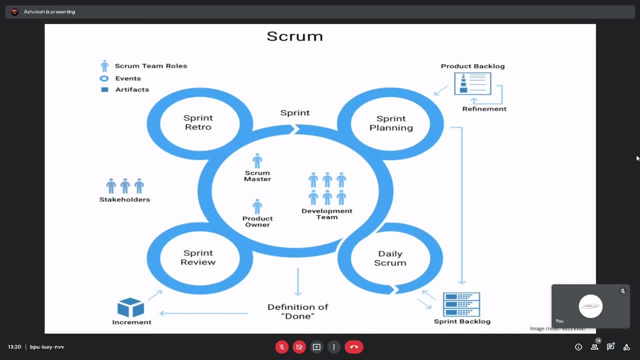 Where should we get the veg non-veg? Where should we get the name of the restaurant? All these things should come. We have decided this, So we have decided Basically, we, as you all had said, so we are the developer. 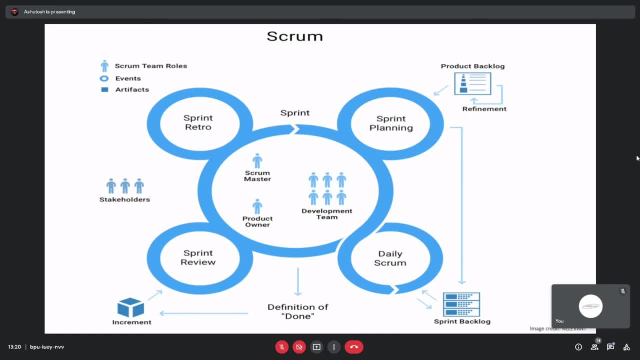 Kavita is our tester, Yashya Shree is also our developer And our client is Prem Raj. Okay, Those who want us to develop this thing, They want us to develop it. So we are all a team, right. 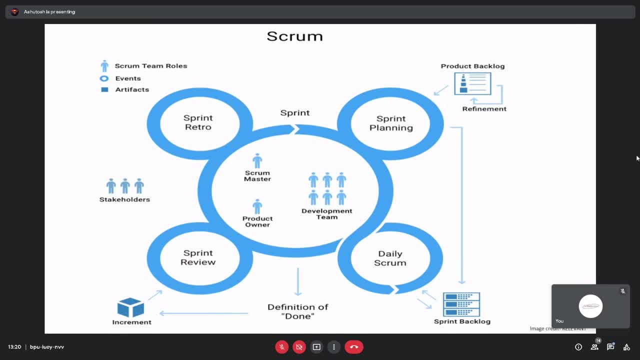 Say yes, Okay, And you can say okay, So we have decided, Okay, So we have decided, So we have decided. So we are all a team, right? Say yes, Okay, So we have decided. 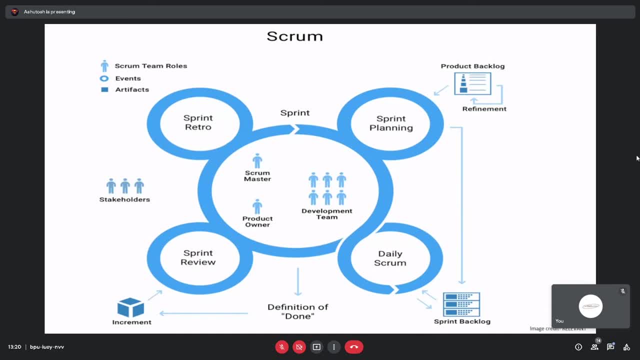 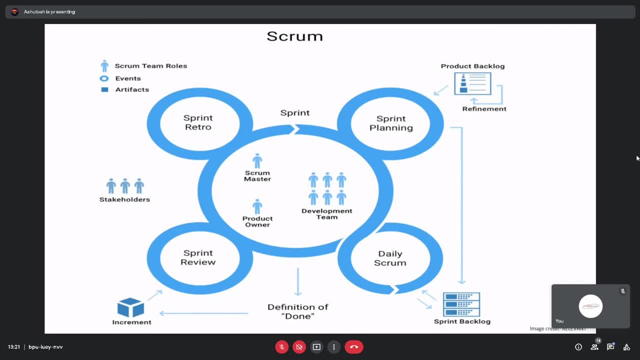 Correct. So the developer's team will start to develop, And this methodology is so famous. What used to happen first? that after developer's work was over, tester used to start testing. But now what happens Along with the development? tester cannot start testing, but can start to plan out. 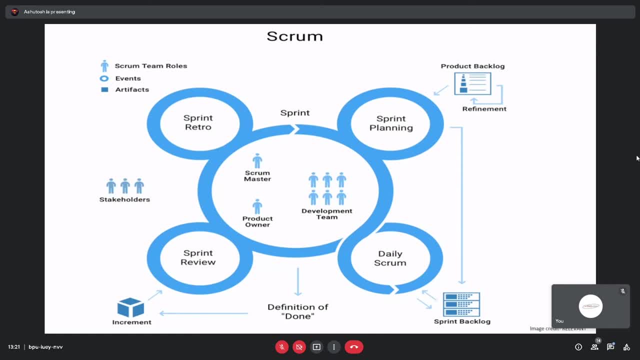 But now what happens? You don't have to wait for the development to be complete. then we will start the testing planning and making the strategy. You can start together. As soon as you get the testing, the tester starts testing. 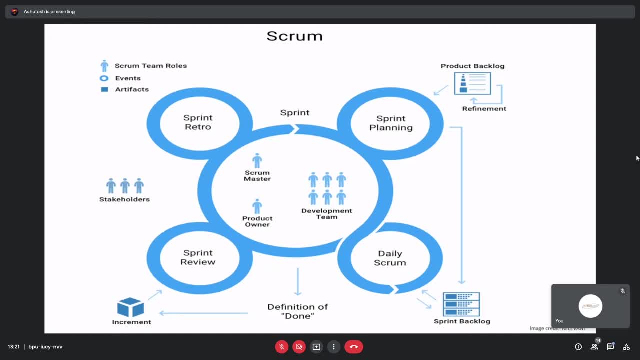 During the whole sprint, this thing is decided. As you can see, here there are so many words written- sprint, sprint, sprint. So you should know what a sprint is. What a sprint does is we have taken a set of work. that is the amount of work we have taken to complete this particular sprint. 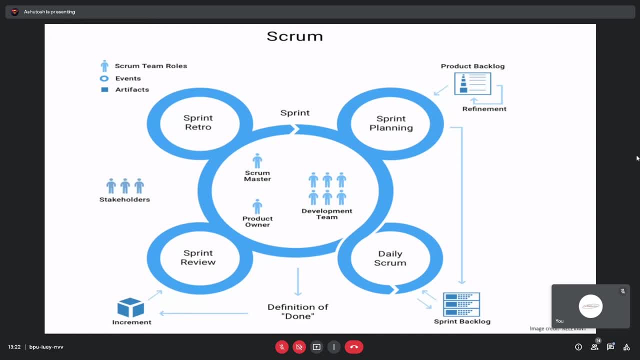 So we decide the time period. We basically take a week's target and we have to complete this thing, this designing or maintain the database. Okay, So we have taken this task in that sprint. So what is a sprint? Any small set of amount of work which is decided to complete in a particular timeframe. that is a sprint. 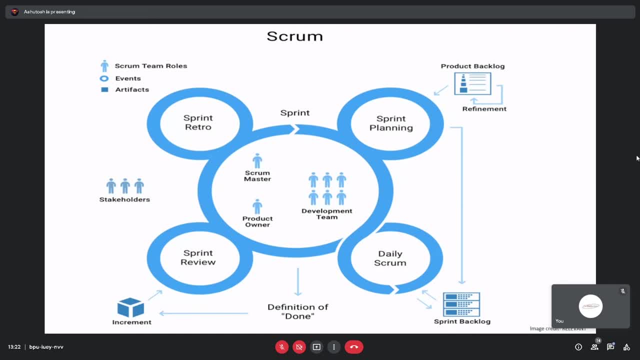 Okay, So in sprint planning, as I told you earlier, in a particular place right now you can imagine, there is a notepad where we have written that Zomato needs this page to be designed like this: He needs the restaurant claim. 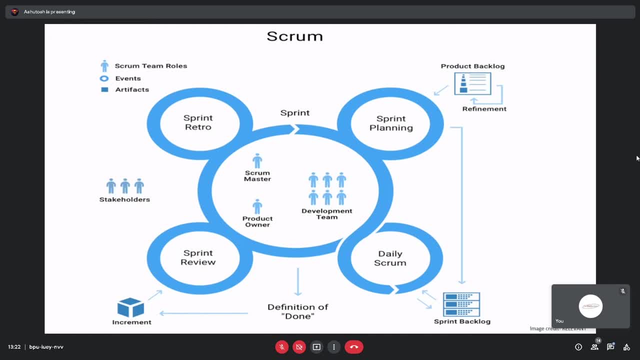 Okay, So basically, best seller restaurant should come in the first page. So we decided this in sprint planning After deciding. so we were given some work that you develop this. Yashashree was given, Mithilesh was given, Tapas was also given. 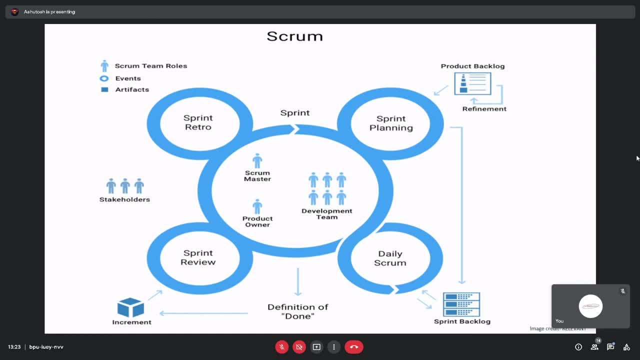 These are all our developers. You all were given some work to complete. Okay, Now, the biggest advantage in this is basically that you have daily scrum. we call it scrum call. You have to attend that scrum call And that is about 15 minutes. 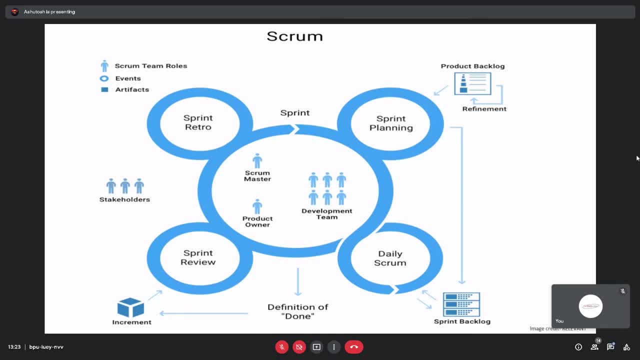 Okay, Where you have to report yourself That: how much work you have done today, How much work you are going to do And what is your plan. specially Okay, And this meeting will be held for scrum master. So, right now, who is your scrum master? 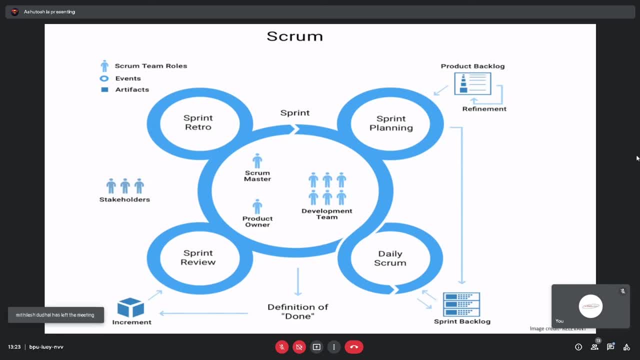 Tapas, you tell Right now. we had given an example. So right now, if you are our developer, then who is your scrum master? I can tell. So scrum master means team meetings. This is normally in my case. normally in an organization case, it is team leader only. 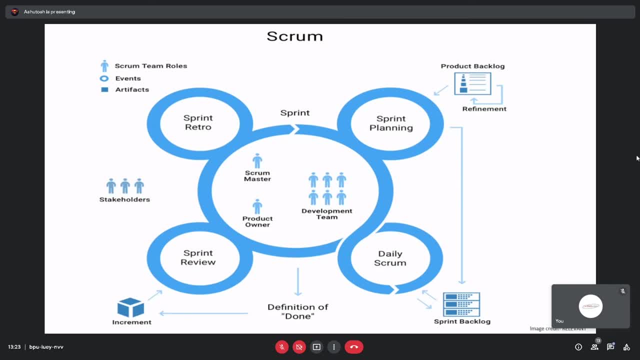 Yes, Like a team leader. 5-6 people form a team of collaboration, So one of the sign is that the team leader has more than 5 years of experience. Correct, So that will be Yes. yes, You can continue. 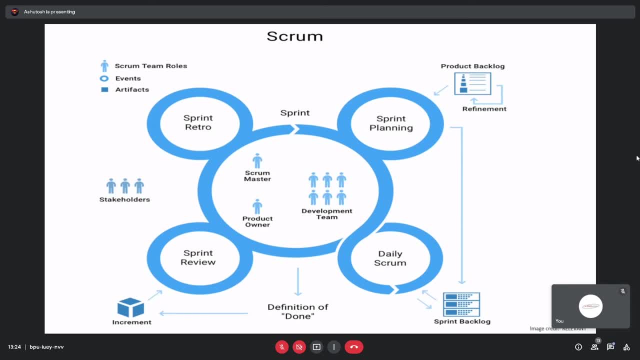 You can continue. Yes, Okay, You had said about testing. Testing is normally the easiest work. What it does is that it returns a script That today, by doing this, this will happen, Like test cases, if we go to hacker rank and do some coding right. 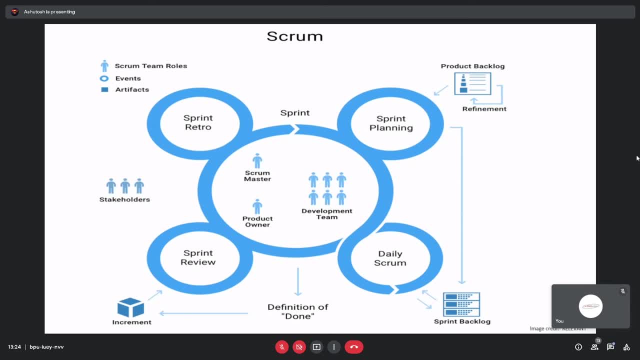 Right, So we have done some code. it has some test case, So normally it is the same case: The code that we are writing has developed And the testing, the test cases that happened. what happens? It is made only by testing. 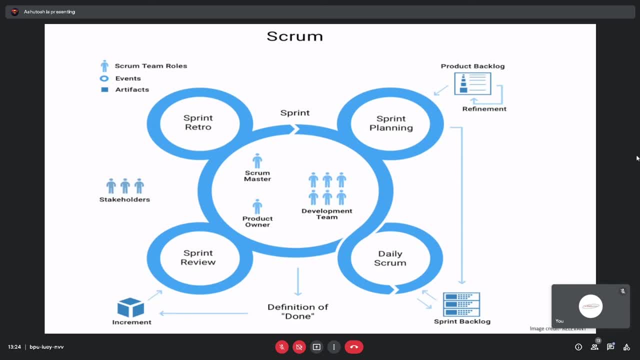 Test. Okay, okay, Correct, correct. So I was asking this. Right now, I am your scrum master, So I am your scrum master, Anyways. So this example was taken. So, yes, Everyone cannot become a scrum master. 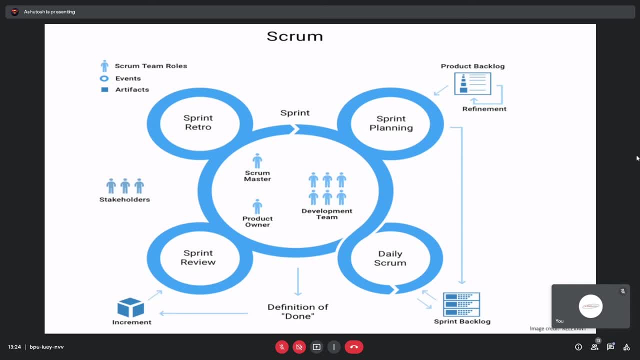 5 years of experience should be there. They are technical leads And especially in the name of scrum master, it is that he is a master. So a master can only become someone who has all the knowledge. Everyone knows how to handle it. 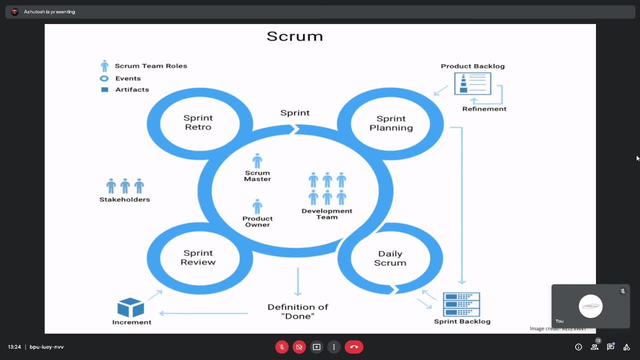 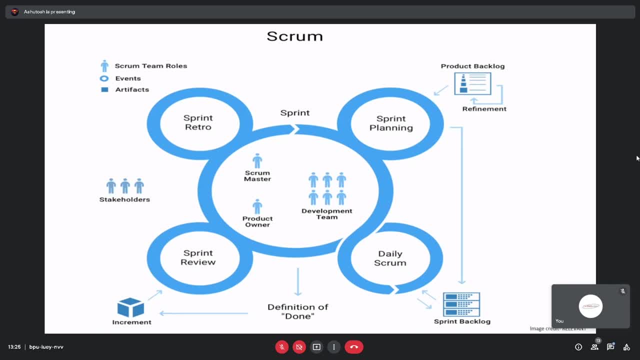 Yes, Yes, Yes, Yes, That is what we said. Okay, After scrum master organizes a meeting and the scrum master is taken so that he can explain to the developer's team as to what work you have to do. He knows it from the beginning because he is assigned the work during this daily scrum. 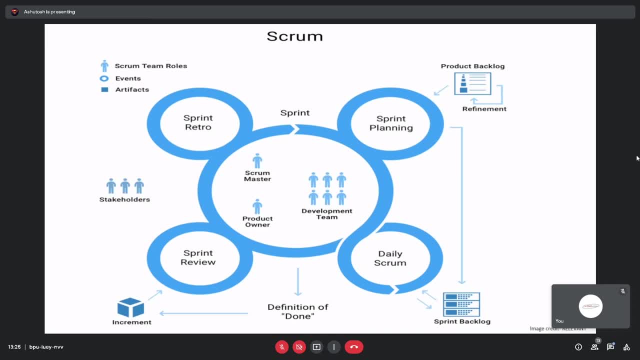 meeting, Okay, Decide Or planning, And especially during planning, Not in a daily scrum calls. So the sprint planning is done. That is the first one. In the meantime, the scrum master assigns which work to the developer and which to the tester. 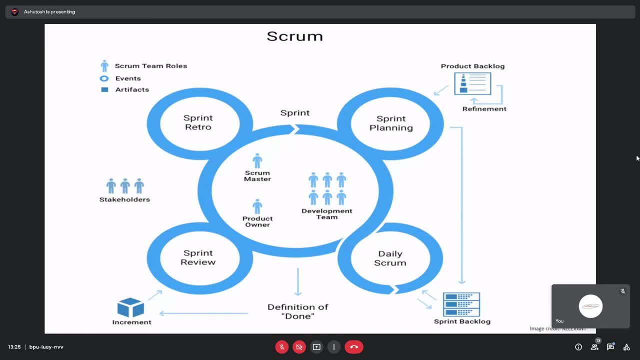 The work of the user tester is easy. but if the tester does not remove the defects then his ban will be saved. So the tester also has to remove the defect. He cannot see it from the perspective that the developer has made it, then it must have been made right. 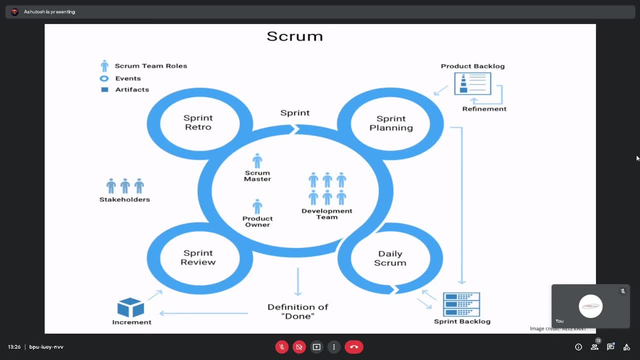 No, he will have to see it from the perspective of the bug and he has to find bugs. And it is not that the bugs do not come out, thousands of bugs come out. You can say that the tester should have an enemy from the developer. 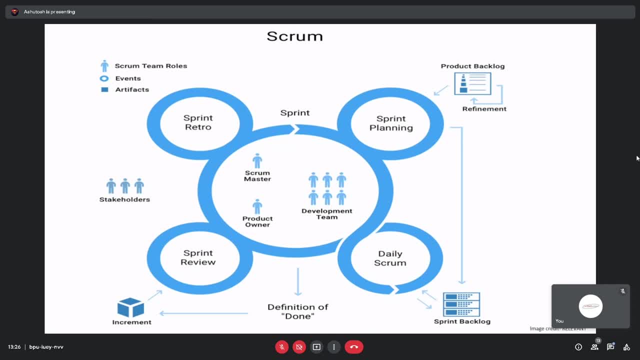 So the enemy can show in his work that, yes, you have done this work. now, this is a bug in it. you solve it and give it Yes, yes, yes, Cutter enemy, you can say, And in daily scrum you have to report everyone that today I did this work, today I did this test. 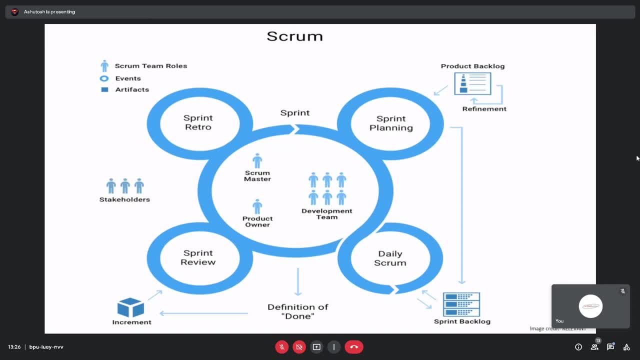 today. I did this. After this thing, there is a sprint review, So one week is over and every day there is a meeting of 15-15 minutes. Now, after the meeting of 15 minutes, if someone has been given any work and he has not completed it, 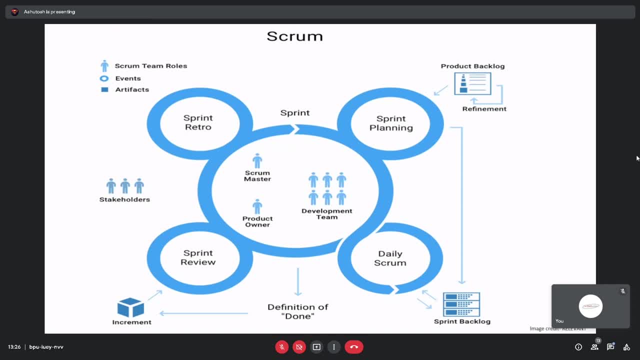 Suppose Soham was given 10 jobs, Tapas was given 15 jobs and Kavita was given 5 jobs. So he has somehow completed 50% of the work because there is a duration of one week, Right, But some work is left. 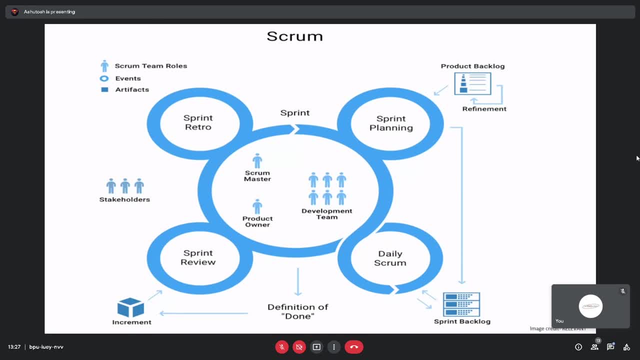 Okay, So we will take that in the next print. Okay, We will ask this in the sprint review. So, scrum master, they will ask you how much you have worked on and which story which is written in your notepad, or whatever task is given to you. 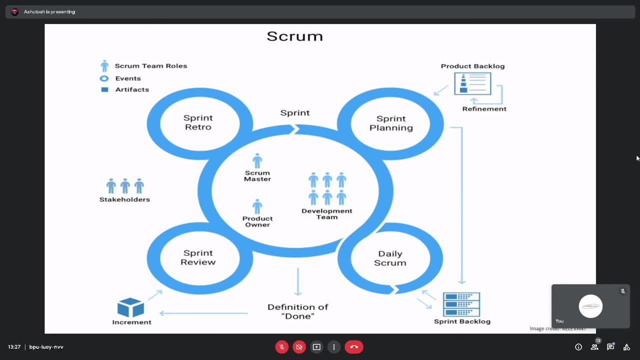 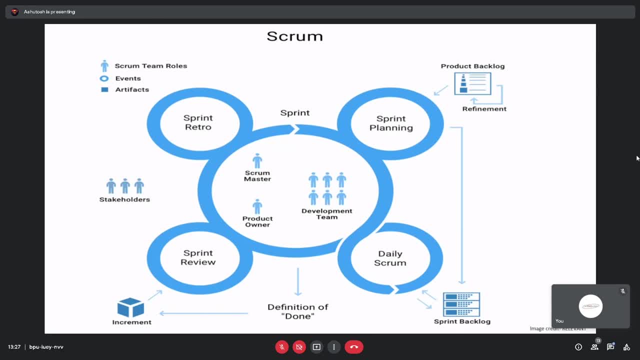 So when you use up yourج Apps, Yep, So the permission for each one is very good, It is Ok. hello guys, am i audible? yes, it's your audible, i think. no problem, no problem. so, guys. uh, as we were talking about like sprint planning, what is daily scrum? what is it till now? you? 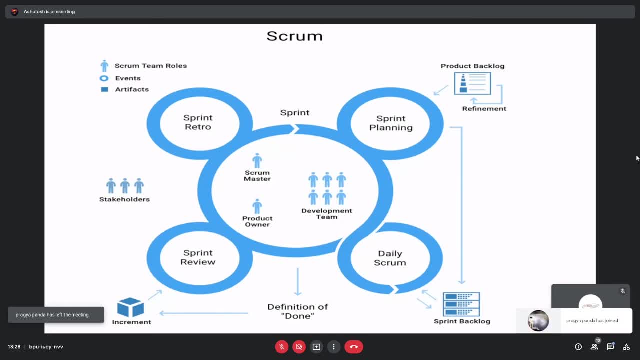 understood like things, that when we attend daily scrum then we have to attend for 15 minutes so that we can plan out things like what we have done or what we have to do. okay, before forwarding this, i would like to tell you something which i thought i will say in. 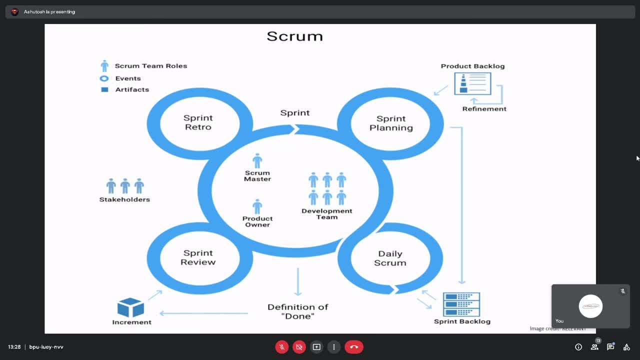 the end, but i will say it now. okay, like, as someone told, that tester has to do a lot of work and all those things. uh, by that time, premraj, can you like check in the background that what is the issue? sure, sorry guys. uh, yeah, welcome back. yeah, yeah, thank you, thank you. 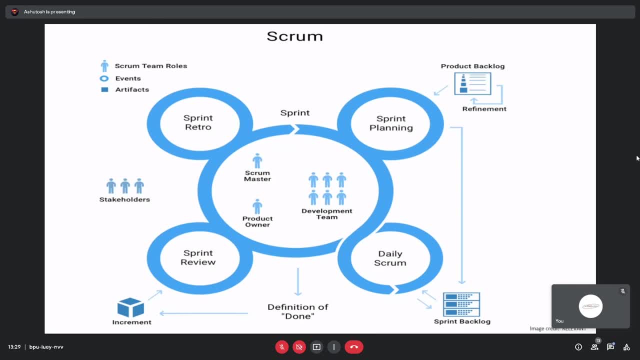 so in this, with the whole process done, yeah, if you want to add some point, uh, you can continue. from the stack holder: yeah, yeah, uh, stakeholders, uh, do you guys? uh, okay, so leave. i will just directly tell who are the writer, who are the stakeholders: stakeholders in our organization, the people who are directly affected by our project or our business. 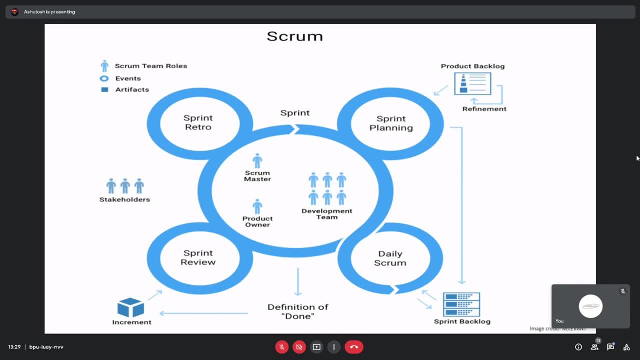 a stakeholder of us, like manager of our organization, who are leads of those who are ceo or those who live like big people in our organization, those people- investors- who have invested in our organization or our company. they are government people like those who are getting gdp through. 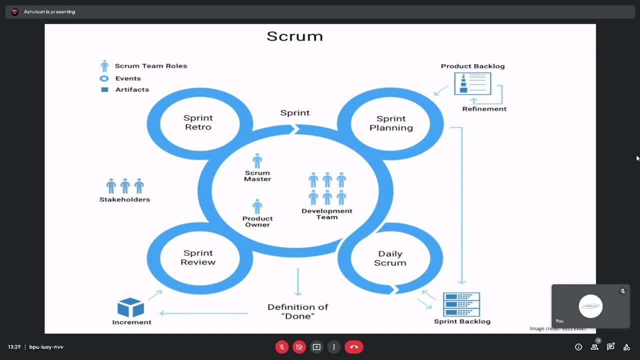 our organization, in country growth and all those things recompensated. so from these particular people believed, i mean, what is the best way for us to improve our organizations? and the kashgar? yes, you guys have well as well. i am happy that i have made up my mind about all. 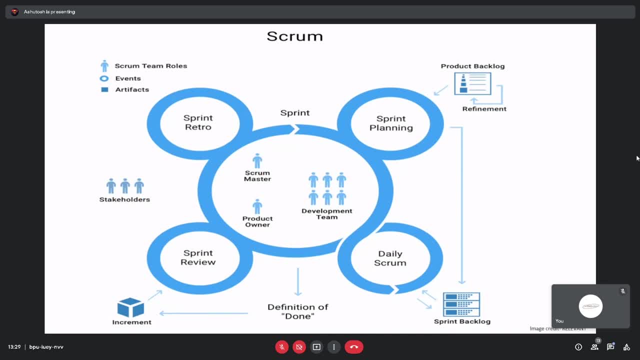 and all those things. all those people are the stakeholders. in simple terms, stakeholders are those people who are directly affected by the work of our organization. our stakeholders provide us with resources, our stakeholders provide us with investment. all these are the work of stakeholders. now, like this is the what, all the things that we have to tell you. 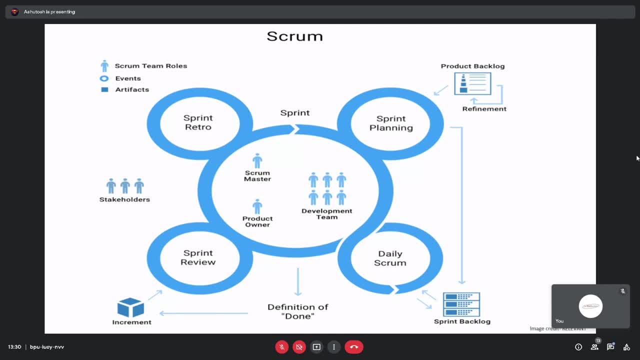 guys about the scrum. apart from this, I was saying something like the role of a tester, like the work of a tester is a little less like as, like some people here are of 4th year. sorry, sorry to interrupt Ashutosh. yeah, so what we say is that we are tied to time. 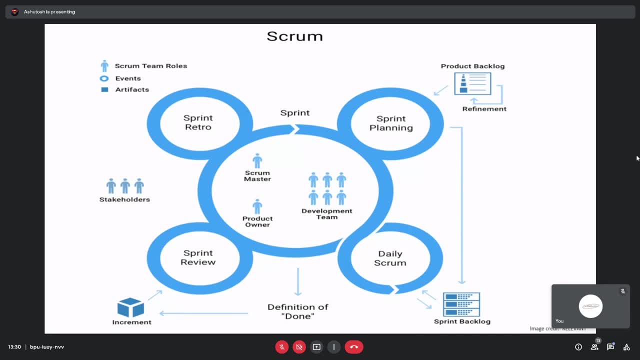 so we have very less time. yeah, yeah, yeah, it's not like that. so so this session is almost over, so thank you, which we are going to provide you. what is SDLC? there is a short summary for this, so thank you, which we are going to provide you. what is SDLC? 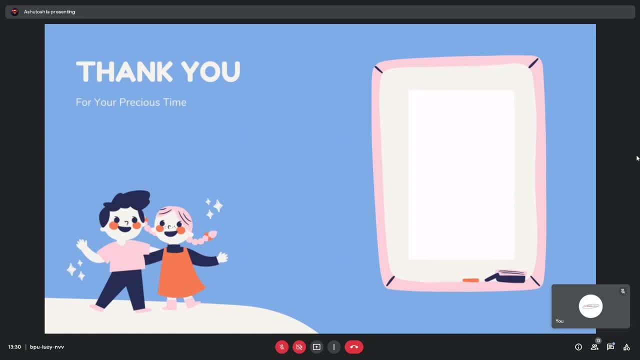 so that when you enter from the corporate world, you should know what kind of system is going on, what are the procedures, and thank you for your precious time. it means a lot for us. yeah, it means a lot to all of us. just wait for one minute if you want to. 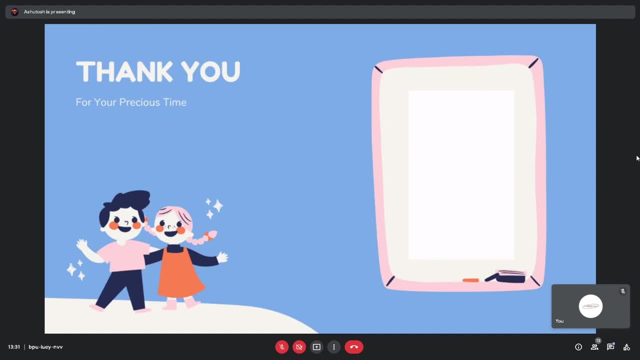 and it will be. we will be very happy. just wait for one minute and I will ask Prem Raj to tell about Urbara's. yeah, so before we start, Prima Raj thanks a lot to all of you guys and like I will like stop my presentation now. 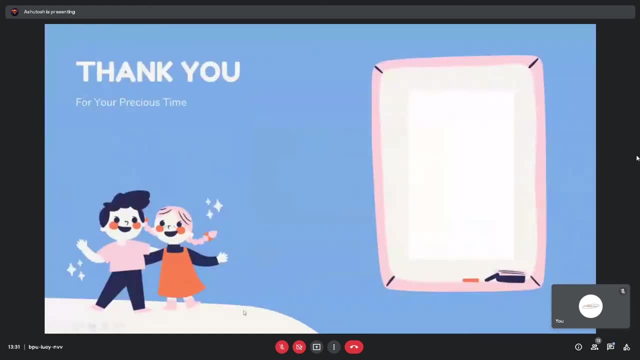 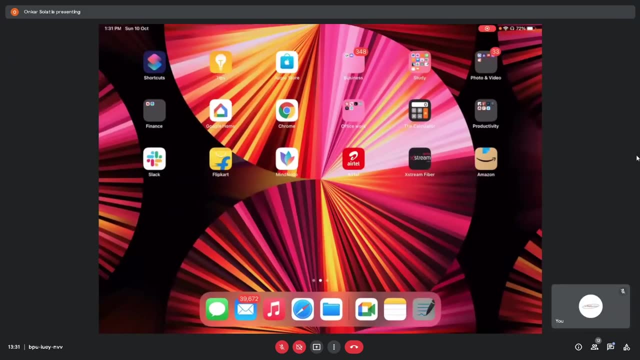 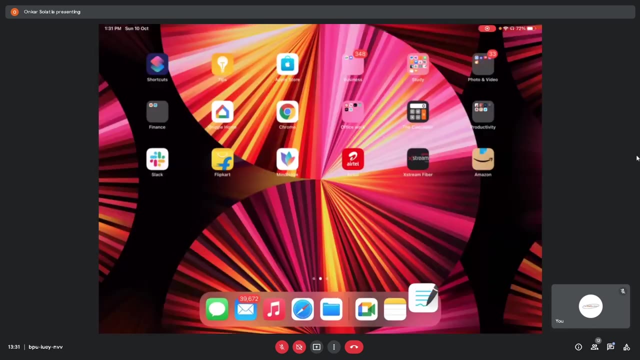 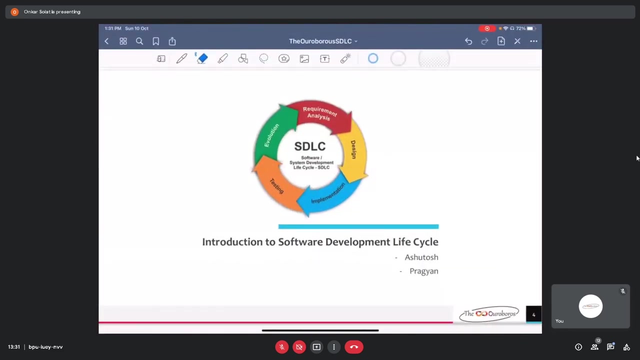 you can carry on, Prima Raj. yeah, thank you, Ashutosh and Pragya, for the lovely session and the informative session. yeah, Unkar, can you please take over the session? hello, Unkar, yeah, sure, okay, so am I audible? yeah, yeah, yeah, you are audible. 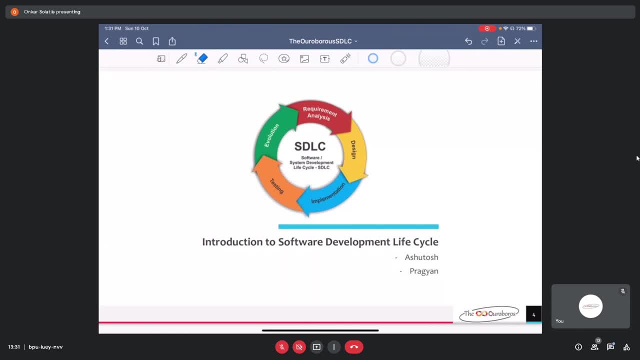 so I would first- really I am thankful to Ashutosh and Pragya. that was a wonderful session. so it was about SDLC. it was awesome. I hope everyone enjoyed it. I will give you a bit information about what we are doing here, why we are gathered here. 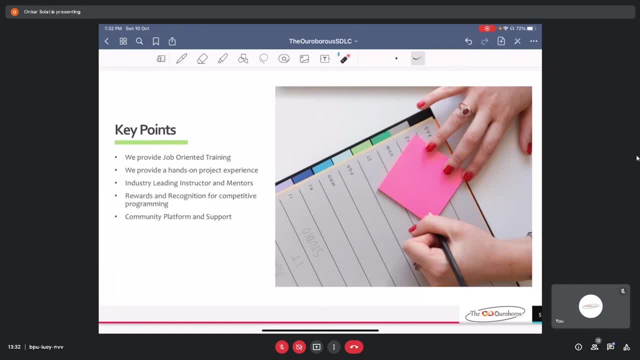 okay, so we are Ouroboros. you might have heard this a lot of times. so we are Ouroboros. this course, or this sessions, are leading to leading you all to a specific course. the course will have certain points which will be in favour of you. 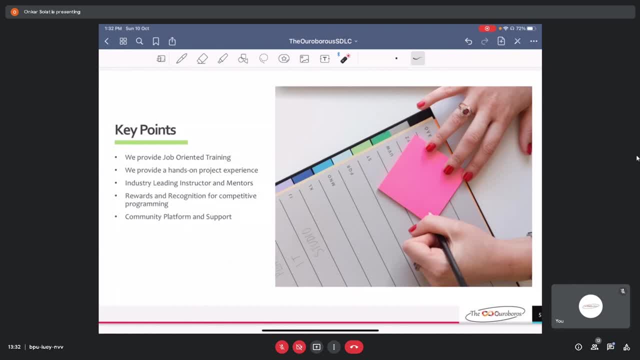 you, as in students like 2nd year, 3rd year or 4th year students belonging to computer science or computer engineering or other computer related branches. we have job oriented trainings. we have hands on project experience. we will have a lot of projects that will mimic live projects. 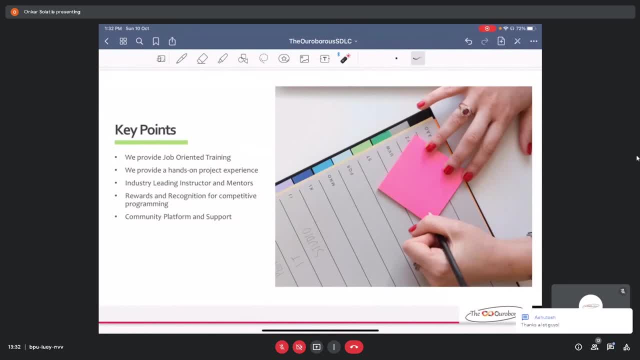 also, we have live projects, but those are for students. so we will have live projects, but those are for students, some specific students, like for last year students or some other people, but also for the initial who are really new to the industry or new to the college ecosystem, like, say, 2nd year. 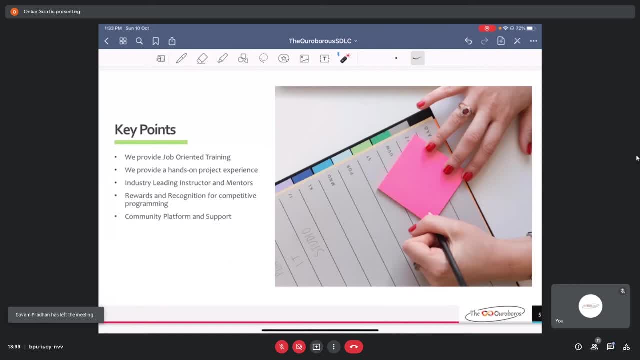 or 1st year students. for those, we will have projects which will mimic live projects. that will be a really good hands on experience for you guys. all the mentors you will get are either from MNCs or have pursued multiple internships or are currently belonging to the. 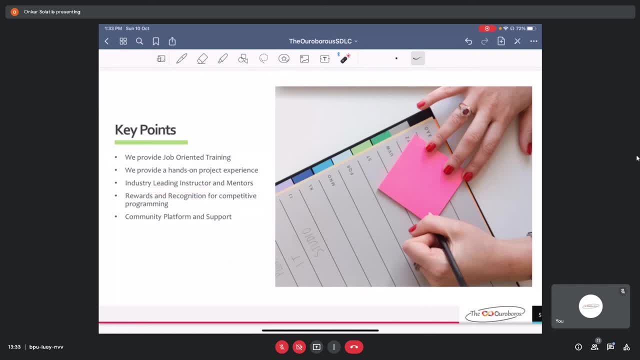 industry, so you will get industry leading instructors, mentors. a very important thing you have to notice is that we are not doing any magic for you, that we will do something and you will get placed. okay, you have to put in a lot of efforts. you have to accept this. 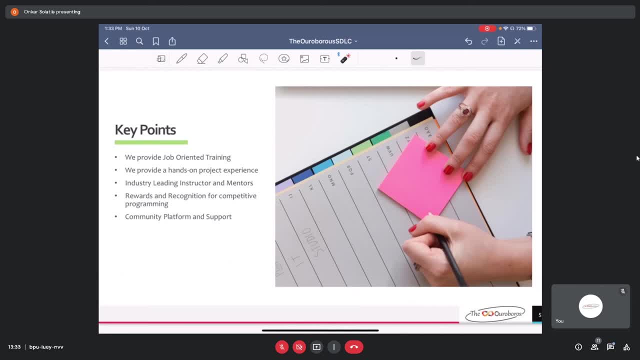 that you will work very hard, but the thing is that your hard work should not go in any wrong direction. like you, should not start doing multiple things or go in some wrong directions. here is where mentors and instructors will help you, because the mentors here work in very big industries. 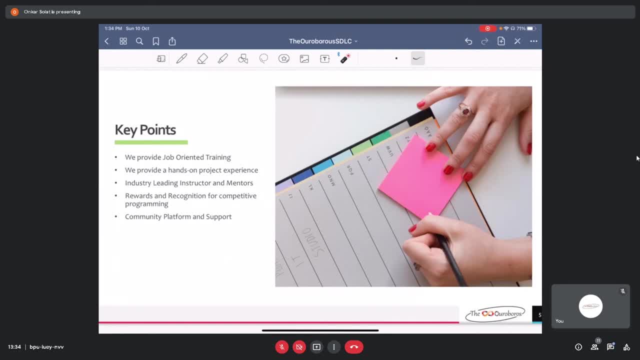 and they all have gone through that phase, all their mistakes, all the positive things that they faced and experienced. their experience will be very useful for you. so that's where these mentors come in, and they will help you. no doubt you will work very hard, that's for sure, but 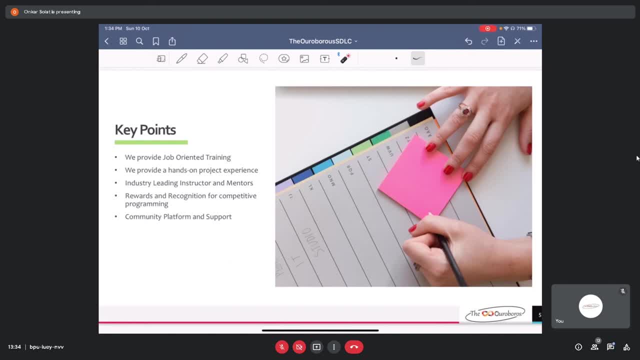 we will make sure that the guidance that you need, that direction, will be given by the mentors. next important point is we will also help you for how to enter competitive programming, what all things should be done, everything about competitive programming, and the final thing is we have a community. 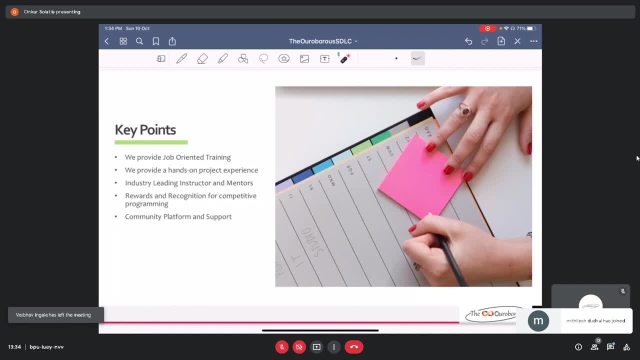 where you can ask doubt 24x7 and people will answer your doubts no matter what. so you can ask your doubts on our social media platforms. there are multiple platforms. we have our discord servers where, if somebody don't know about discord, discord is a platform where you can come in. 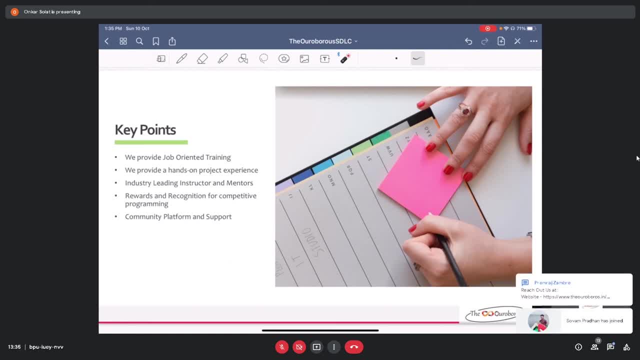 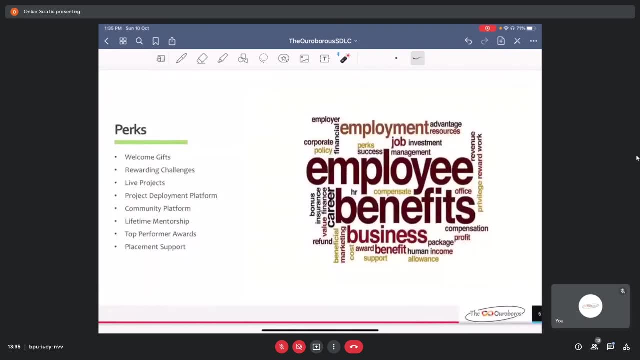 you can chat, you can have group meetings, you can have calls- everything. it is a community platform that will really help you. so these are some important points. if you join this, if you join the Ouroboros community, you will have welcome gifts you will have regarding challenges. 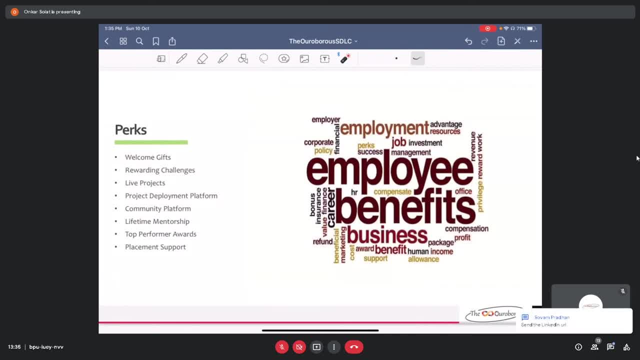 you will be overwhelmed with the challenges and you will be really happy to solve all those. you will get many live projects. there will be project development platform. you can discuss with your mentors and other people, other colleagues, other friends- so that will be really helpful for you. you can ask in your doubts. 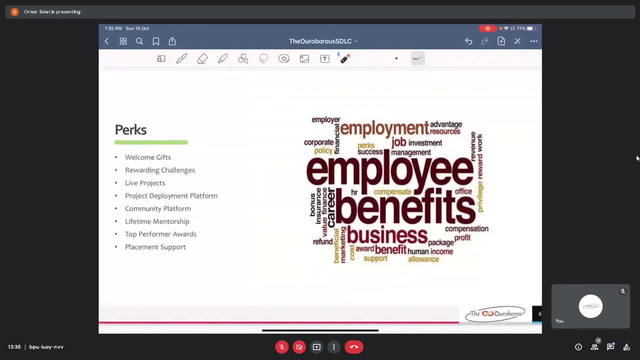 not only doubts regarding the projects, I am saying any kind of doubt which you have about your career, about anything which will lead you towards your job or towards your dream company. that will be helpful, that will be fulfilled here. so any doubts, all are welcome. we have lifetime mentorship support. 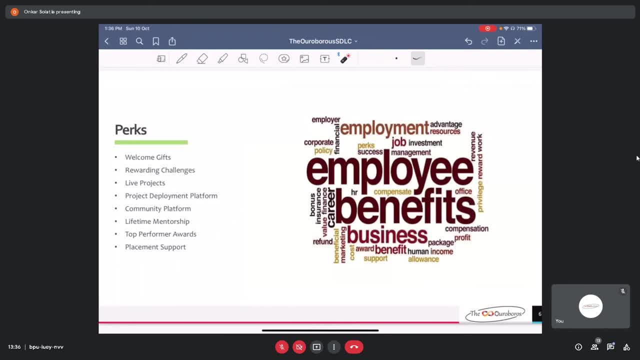 so our mentors will never say no, they will ask for some time. as you know, these are industry professionals. they will be really busy, but they will ask for some time. but they will surely answer. after this we have like awards for the top performers, so we have challenges. as I told before, 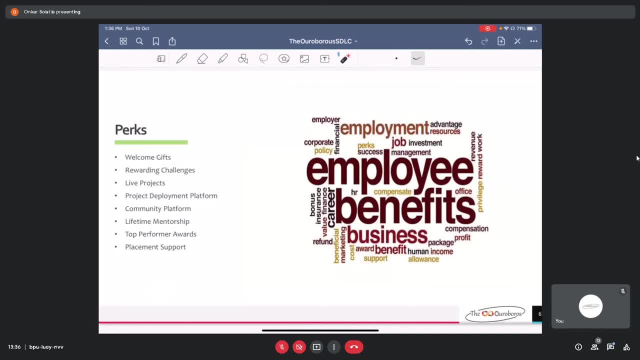 so whoever are the top performers will get many awards or kind of gifts or something that will inspire you again for the next challenge. that is really helpful. and the final thing: we have placement support as well. we I will let you know in the further slides what we have for the placement support. 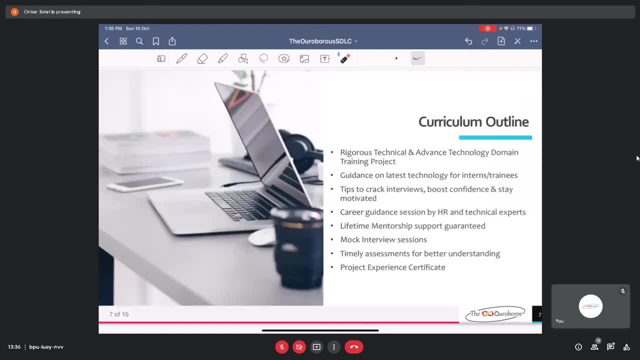 you will be really happy for listening that. so the career, the specific course we are talking about, just confirm. am I audible? is my connection still good? my screen is visible. yes, sir, thank you. so the curriculum we are talking about here: it will be a rigorous technical curriculum which will consist of: 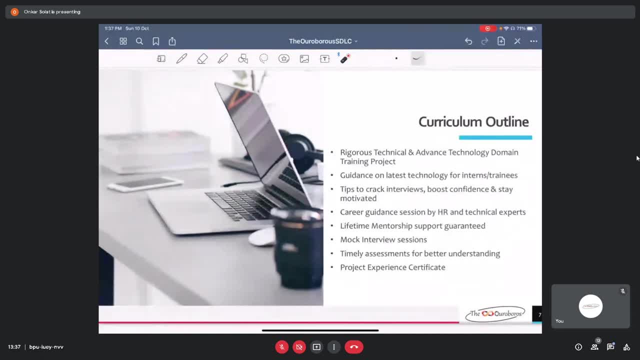 a project which will consist of a lot of things here, not only about the technical, also about your behavioural aspects, about your communication and other things which will help you to crack not only one, but multiple job offers or internships for the earlier students, like second year, third year students. 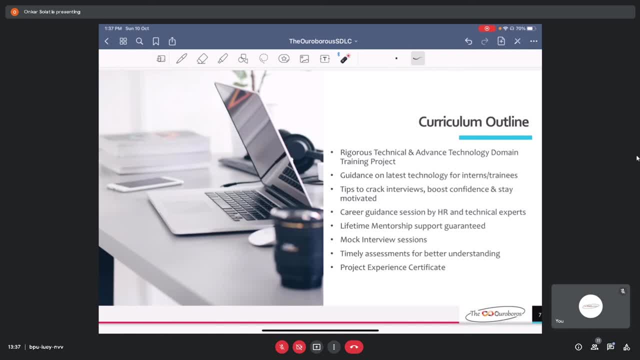 but also for the fourth year. we are talking about job offers. so it will be a rigorous training wherein you have to put a lot of efforts. we will put a 1000%. we expect you to put your 100% here. so next point is we will guide on latest technology. 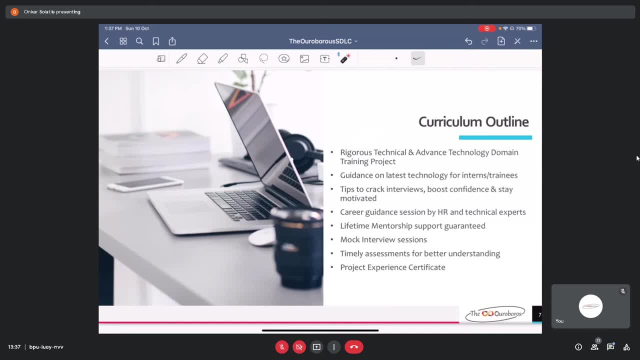 because the mentors you are getting here are really widespread with the knowledge, with multiple technologies, with various latest cutting edge technologies they are working upon. one thing for sure is like if you, if I roughly divide the curriculum, 40% is about teaching. that will be very much like coaching. 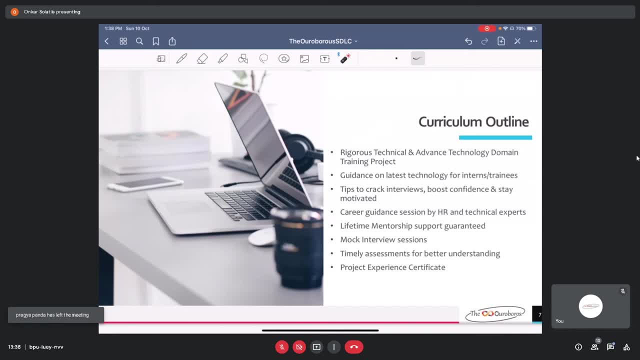 but the 60% is customized, like for mentors. so whatever you specifically, as a student, have your doubts or you want to pursue some career, that will be guided here and that will be of more focused, that will be of more focused. so I guess you are getting the 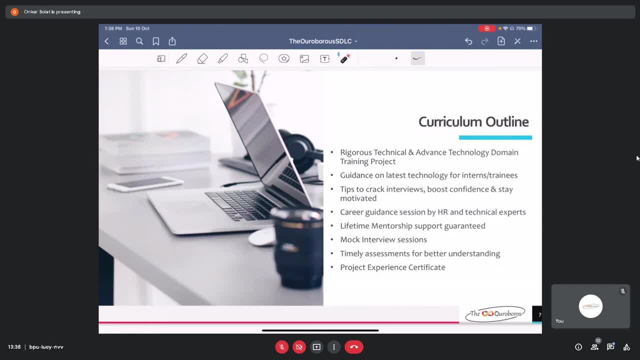 gist of what we are bringing for you. so, as I told you before, there are industry professionals who have gone through all this process. they have a lot of knowledge now, lot of mistakes they have done. they have overcome that and they will guide you. they will have lot of tips. 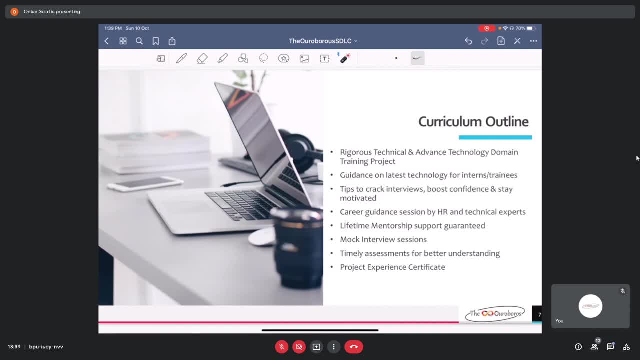 what to do, what not to do, how to boost your confidence, how to do other things, how to gain everything. so that will be really helpful for you. for all this in this curriculum, you will have mock interviews. there will be a lot of interviews. after a point, you will be like: 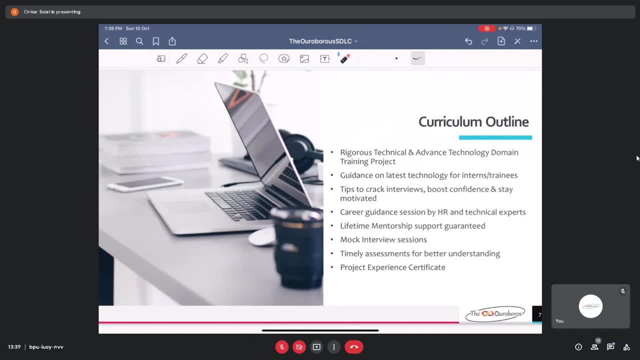 let it be any company's interview, I will be prepared already. these many interviews are going to be there for you, so just be there for the interviews. it is clearly going to be enjoyable. it is really going to be tough, but we will make sure that you enjoy the process. 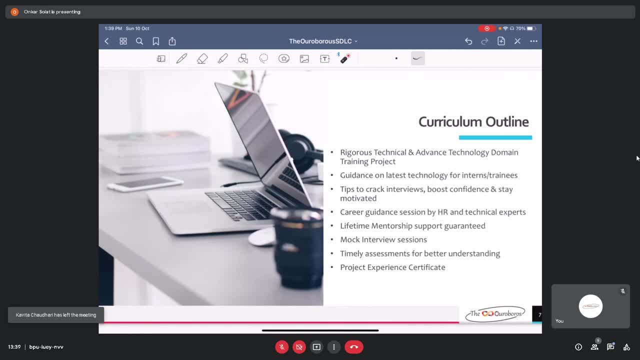 last thing is we are going to have certificate for the project. whatever you want to do, there will be groups for the projects, or there might also be some individual project for some specific cases, but mostly there will be group projects, so you will get the certificate of completing that project. 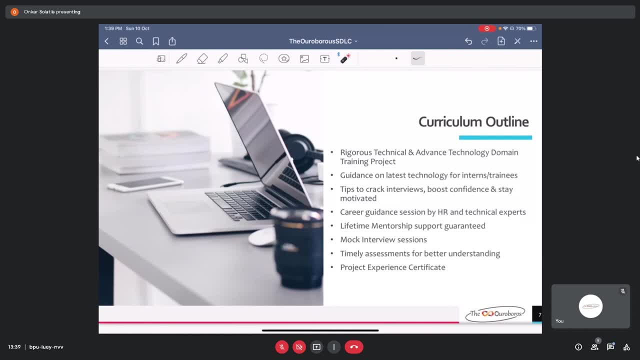 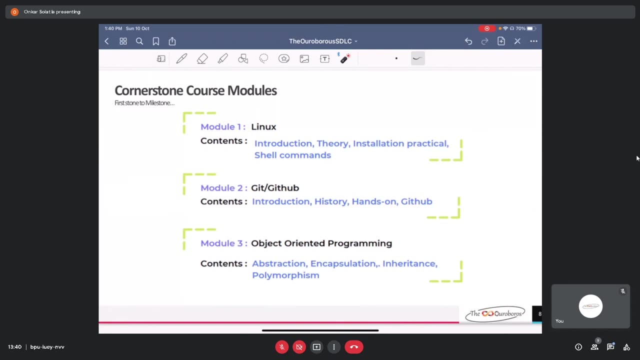 you will have that project in your resume. you will have that posted somewhere so that you can showcase it whenever you go for an interview. so that will be a really increased in credibility in your resume. that will put some weight on your resume. so we will talk about the course itself here. 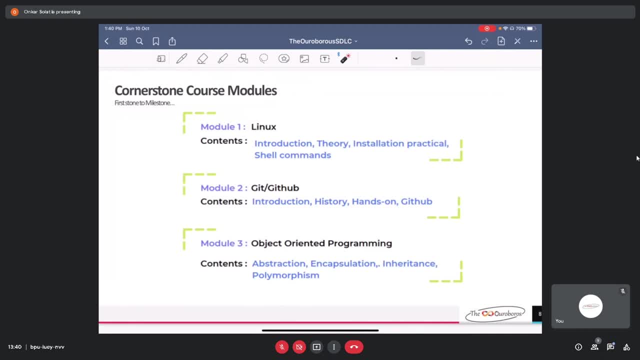 so the course is named as cornerstone course models. we are talking about the course models here, the cornerstone course. in this course you will have all the modules from very basic to really advanced. so those who know things before it will be a good refresher for them and those who don't know anything. 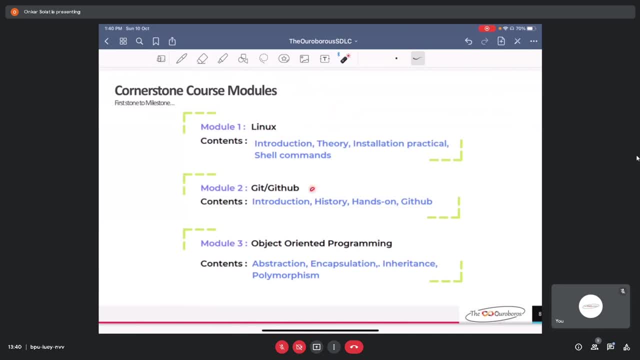 it will be a really good start for them. so we will understand linux here. we will understand github- how to use it, what is it why it got introduced- and we will also use it in our project, like almost all of the things we will learn in these modules. 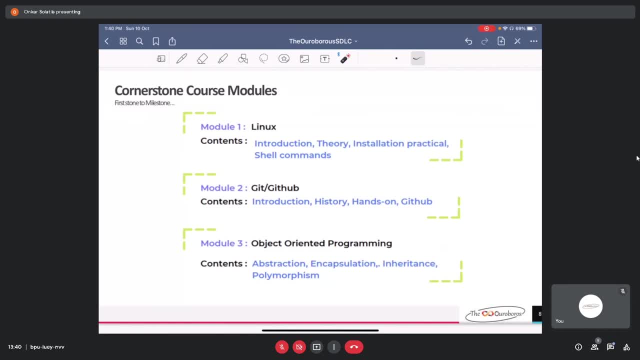 so just stay tuned. we have object oriented programming, which will be way more helpful while building some projects. after that, we have data structures. this will be helpful for your competitive programming, for cracking interview questions, for other aspects wherein, like you, participate in some competitions, hackathons or other things. 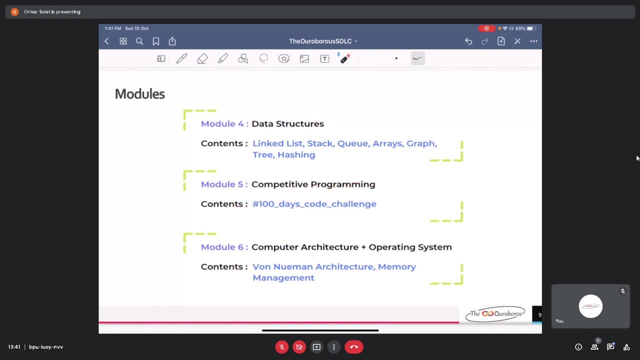 we have 100 days code challenge wherein continuously for 100 days, leaving a single day, you code for certain problems. you get stuck in between, you have some doubts, we get it solved and we complete the 100 days challenge. this is really helpful for the previous batch of students. 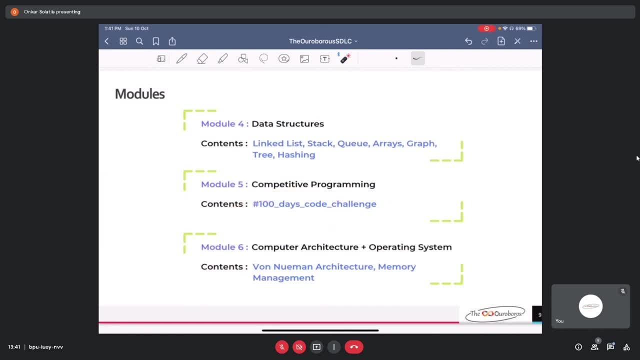 so make sure you start this from the day one. we will obviously help you to start it. but yeah, next part is computer architecture and operating system. this part explains you how a computer works in the background. what are the things it will be helpful for making efficient projects? 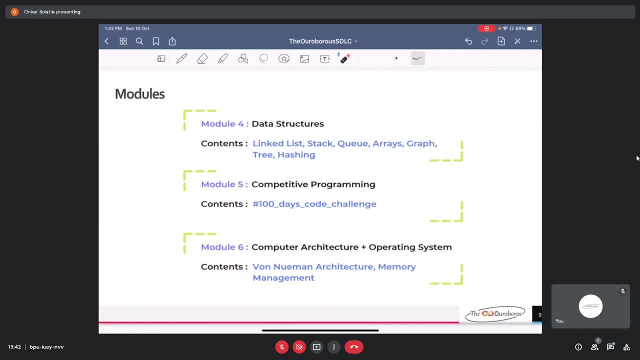 it is really necessary in the industry also. so there are really good instructors, industry leading instructors, teaching everything here. so there are some important parts coming up. next one of them is database. every project needs a database. you will get to know database concepts in depth. you will also use it in the project. 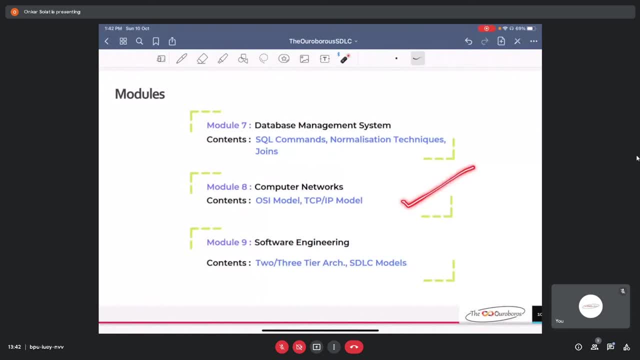 so that will be also helpful again. computer networks is the next part. we will learn networking here, various models, many more things. next is software engineering. like today's session, we learned about SDLC models, some introduction about SDLC model, but in this model you will learn in much depth about everything. 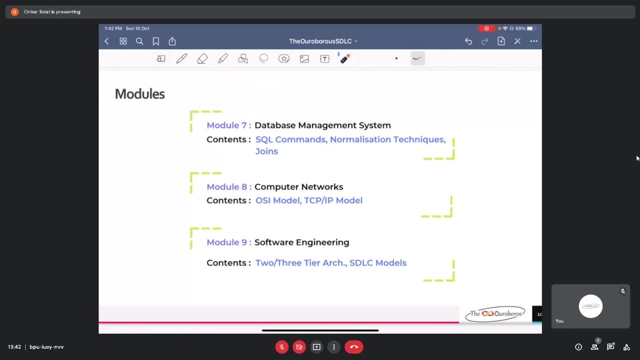 about software engineering, about 2 tier, 3 tier, architecture, about many more things. so this is the last portion. end of the modules. by this you will have been done many interviews, mock interviews. you will have been done a lot of things before. so now, by the time you reach module 10, 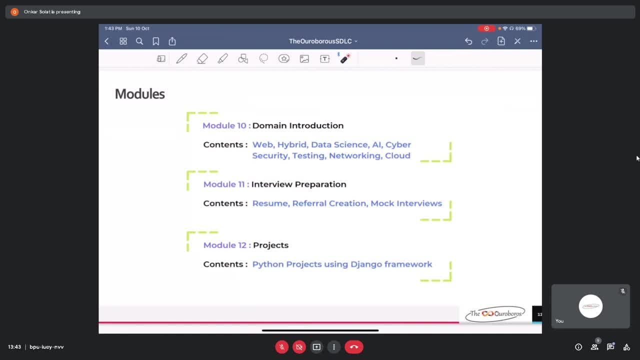 you will be an expert already. so here is where you get introduced to the domains. there are a lot of domains which are being used in the industry. there are many students who are still confused or in that phase we are really confused. so here you get introduced to. 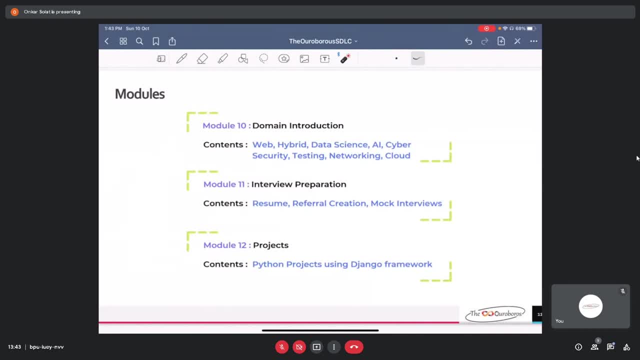 various domains. those are prominently used in the industry. so whenever you get introduced you can choose something, choose a specific domain and then work towards that. so this domain introduction helps you to understand many more domains, like web or hybrid domains or data science, AI, cybersecurity, testing. 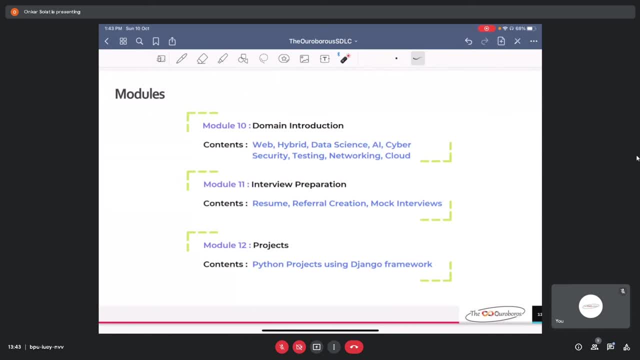 networking cloud and many more, but you will get introduced to the domains so that you can choose something for yourself that you like. after this, we have interview preparation. we will conduct not only technical interviews but also behavioral interviews, so interview preparation module is really necessary. you will personally 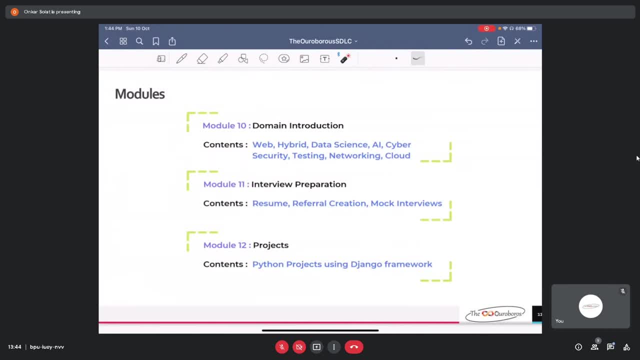 mentors will talk to you, understand what problems you are facing in your interviews, the things you should improve upon. that's where mock interview comes in. we will also help you build your resume to the best we can, and everyone. apart from this, we will also have referral creation. 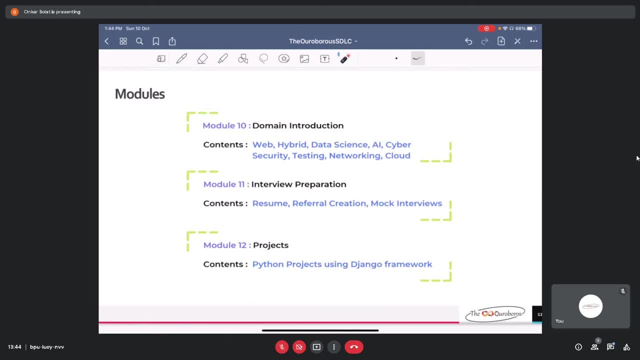 so you understand. you get the gist. because we have a lot of people in industry, this will be a bit helpful, but we will keep this as the last option. generally, people will not need this. after going through all the modules, you will be so strong that you will crack multiple jobs. 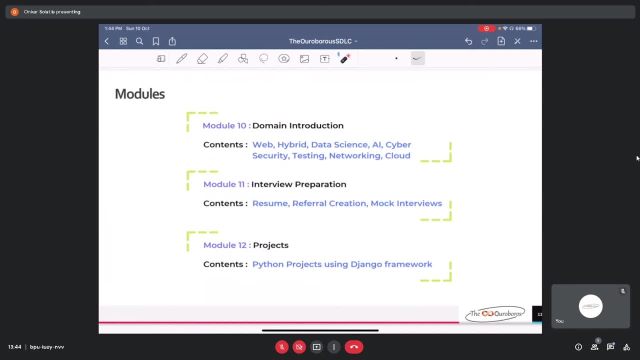 after this rigorous training. and the last point is the projects. so we will be doing projects on hybrid development or django framework and other technologies also. so this will be a module where you will be able to create projects on hybrid development or django framework and other technologies also. 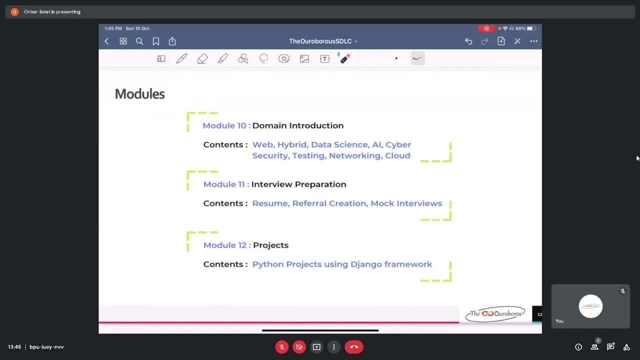 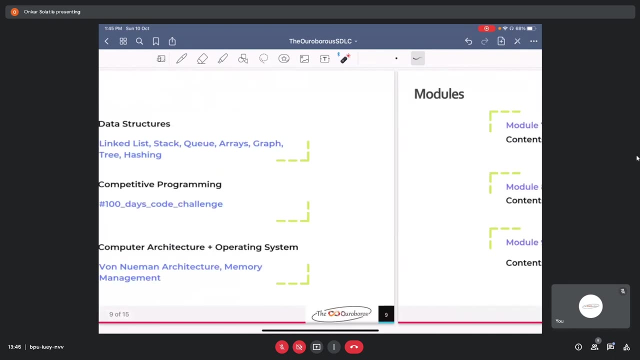 so this will be a module where you will be able to build a project of yourself. it will be a group project or, for some cases, individual projects. so this will be the last one, you will get the certificate for the project. i hope everyone gets what the course will be. 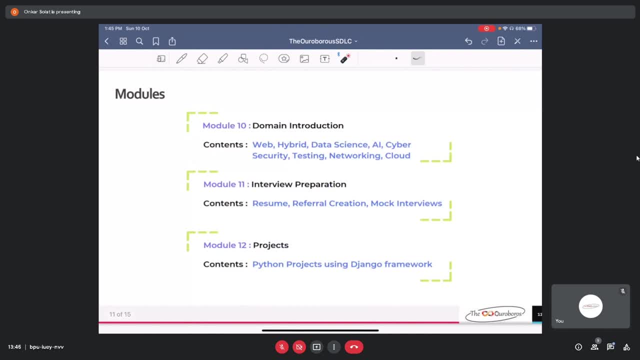 i will surely share an email with you where you'll get all the details, so don't worry about this. apart from the cornerstone, yeah, does anyone have some doubts or anything they wants to know more about this course? can you send the links of linkedin and all? 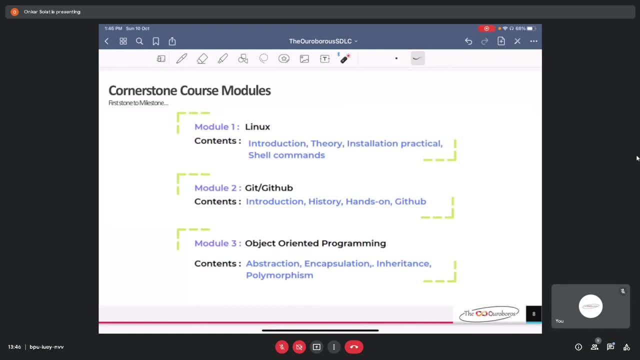 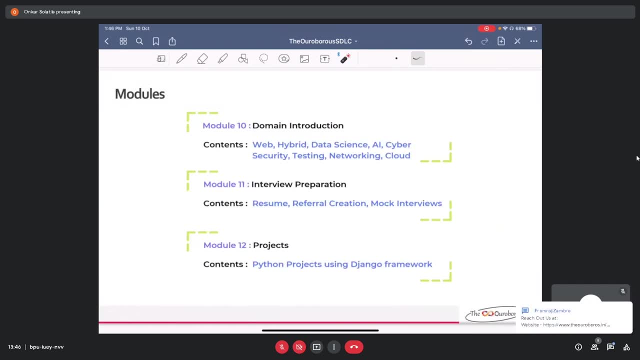 yeah, sure, sure, uh, it will be in the chat. i will again post it. sure, sure, we'll again again post it. don't worry, i'll get all the links again. so any doubts till now? mm-hmm, anybody? nope, okay, cool. so apart from the main cornerstone course, we have individual modules also. 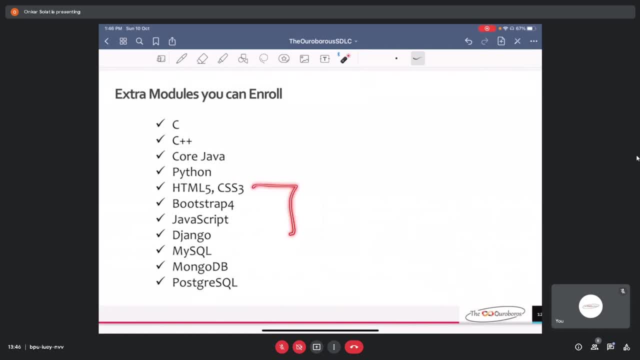 we have certain core programming languages. we have web development frameworks and basic technologies and databases so you can also enroll in any of these specific modules. for details you need to contact on the links given or you'll also have some contact numbers so you can contact directly for any doubts you have or any description you want. 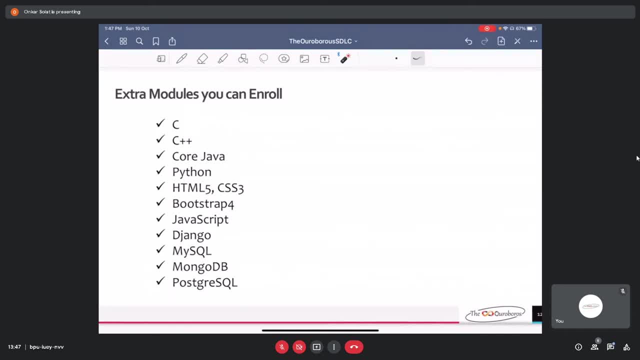 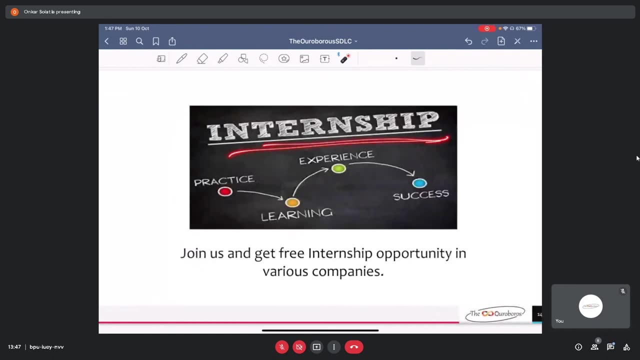 about controlling in either cornerstone or specific courses. uh, we have a box of surprise for all of you that we assure, along with all these courses, we also assure you internship, okay in in industry, which will really help you to like put in some heavy credibility in your resume. this. 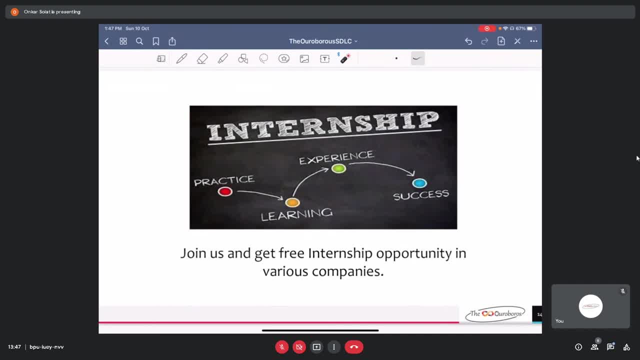 will. you will really stand out with the help of internship and i will also make sure that those internships are in and really edge like cutting edge technologies or the latest technologies- really good projects will be working upon. so don't wait anymore. you'll get the links in the chat to the. 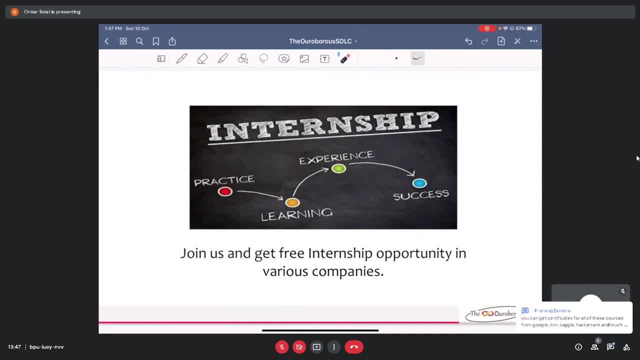 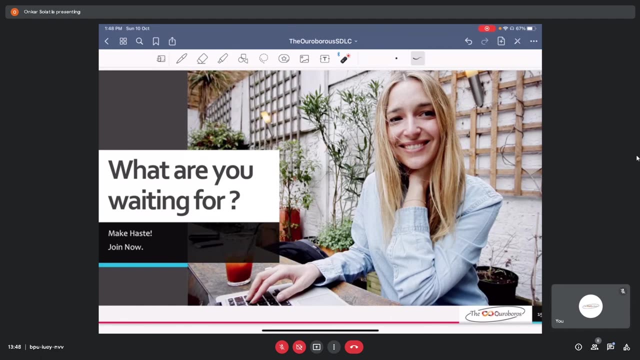 website and also you can follow us everywhere, or we are almost on every social media platform, so that you will be kept posted. so please do join and if you have any doubts, you can just pop the doubts in the chat section here or afterwards later on. if you have any doubts, you can. 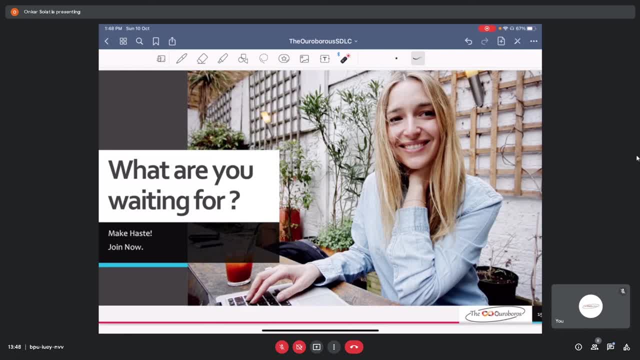 chat or you can send messages. you can also email. you'll get an email link. you'll get an email first of all for the registration link and, uh, please don't reply to that email. that email is not monitored, but you'll get a email in the bottom of the registration page where you can post your. 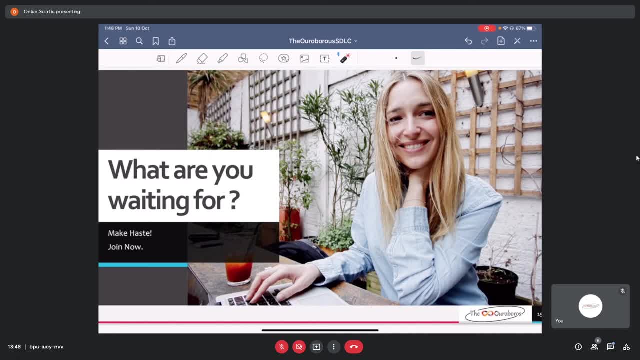 doubts or anything you want to from us? okay, anybody has any doubts till now or anything you want to know more about this over community? uh, um, can you please mention the from where they're going to be able to contact you so that they can get certificates for all of these courses like? 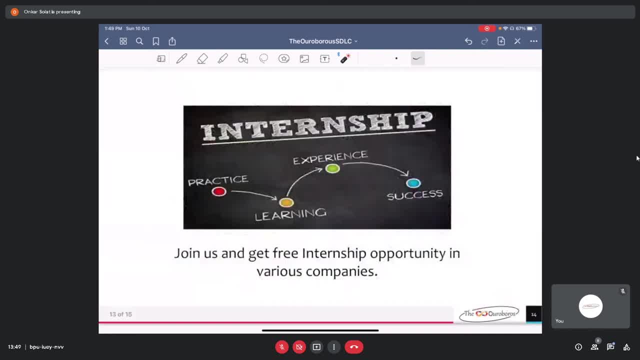 so we have some official certifications tied up: uh, first of all for the internships. understand this: your projects are the live projects that will be done in the industry. so internship certificates, you'll get it from the uh forms or the companies you'll be working upon. we are. 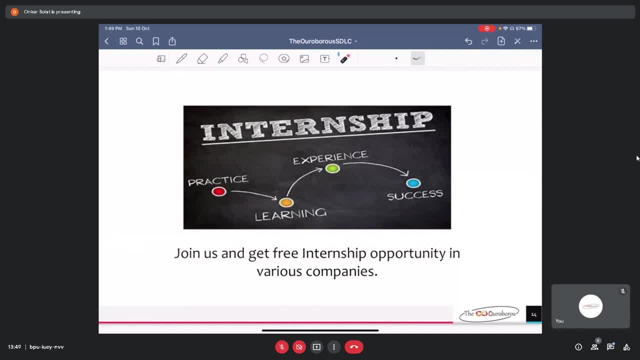 tied with uh- multiple companies where you will get live projects, internship certificates and also about some of the modules you'll you'll get certificates which are recognized by the industry. those are not related to projects. we're just completing about some examinations. you'll get certifications for those.